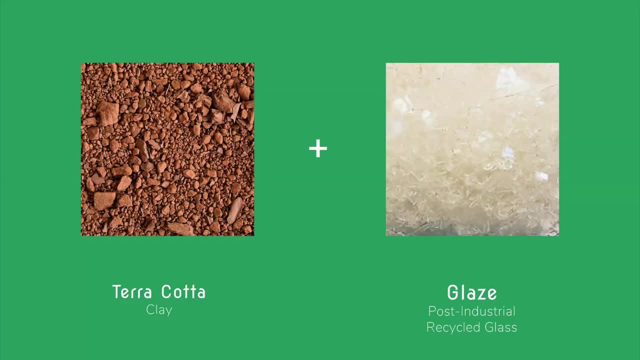 Andy Braman was at this very moment researching using recycled glaze from post-industrial processes- so lab equipment- and trying to figure out if this would be a good alternate or alternate path for glaze development for Boston Valley. so at this same moment we're also we. 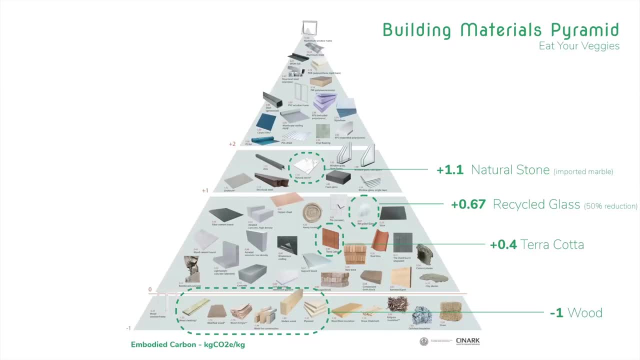 also looked at the building materials pyramid, which is a complement to your food pyramid and, as everybody knows, you have to eat your veggies. so using wood already in this mass timber building really filled up your plate in a good way and we knew we were gonna have to eat your veggies. so using wood already in this mass timber building really filled up your plate in a good way and we knew we were gonna have to. 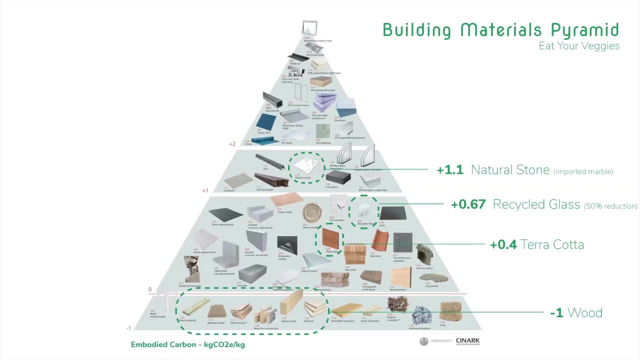 and we knew we were gonna have to use aluminum and other metals elsewhere. so we really were trying to bulk up on that zero to one range of embodied carbon. so, as you can see, terracotta fits well within that. it's a 0.4 natural stone. actually, if you're close to a. 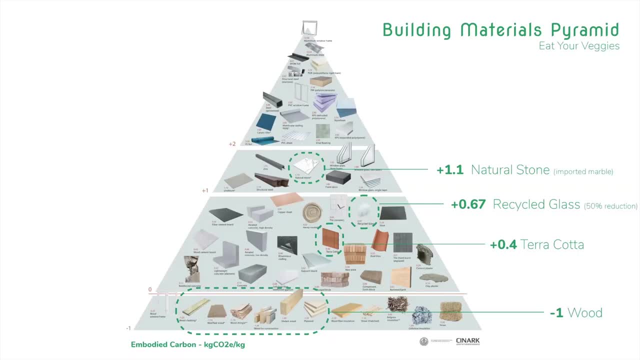 quarry. it's pretty sustainable. it's at about 0.5. but when you're thinking about a specific marble that's very white and has very crisp gray lines that don't have any green, yeah you kind of zero in on very few places on earth that can supply you with that. so 1.1 is actually. 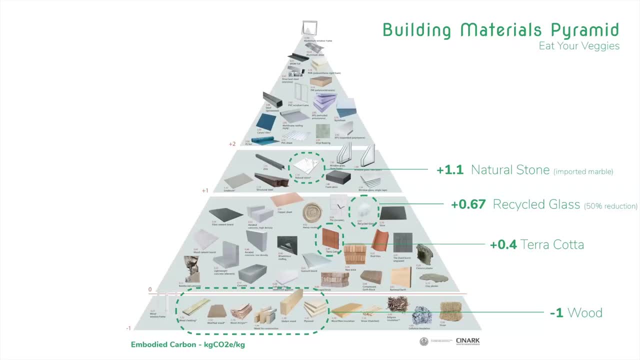 pretty conservative. this is an average over all the EPDs of materials, and so we suspect it's much more. but, and especially if you're further away from it, it just drives up the environment and it's a good way to start your day, so having terracotta and then using that recycled glass glaze which is 50% of a. 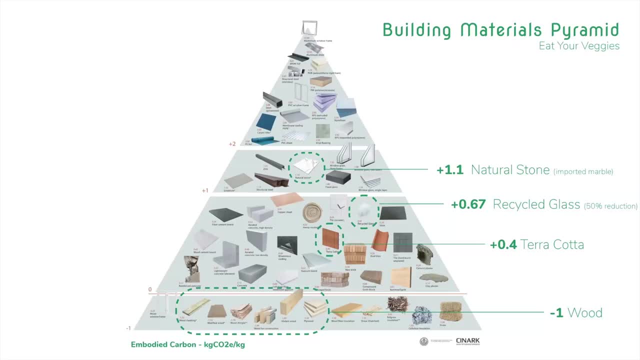 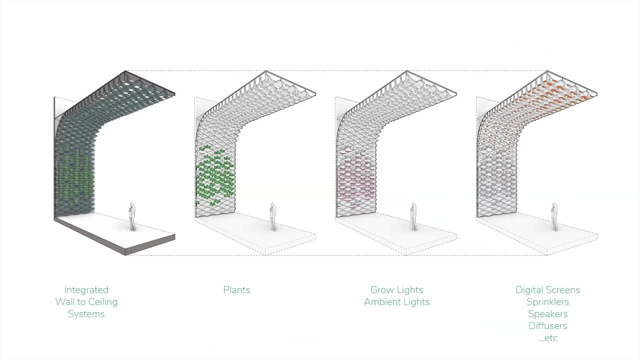 reduction from an original from the original is actually a very compelling story and a compelling argument. of course, the real argument for terracotta over the over natural stone is that it can take on any shape, and so what we wanted to do in the lobby is really create this integrated. 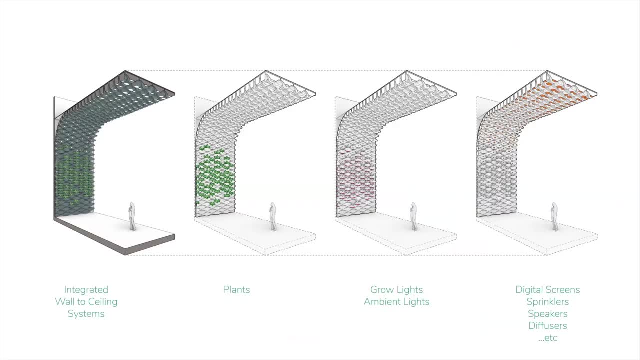 design that would take shape from from a vertical into a horizontal ceiling application and with that take on all the different stuff that's in a lobby, so like your sprinklers or speakers or diffusers, the technical stuff, but then also client requests. so our client really wanted plants, so we incorporated. 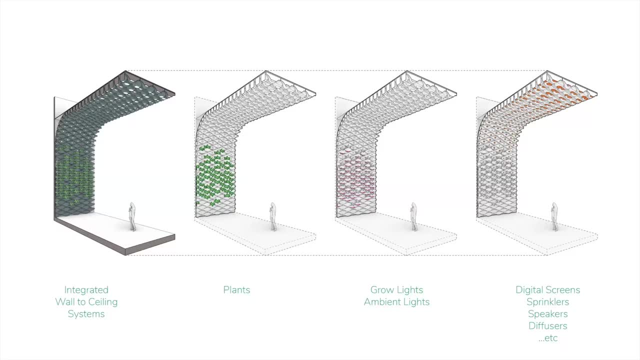 a plant cell and then these floor plates are on the large side and those trend towards the more tech tenant, particularly on the west coast. so we were asked to incorporate digital screens and a level of interactability so you can see those cells as well. this is a very early rendering of the lobby as you're sitting. 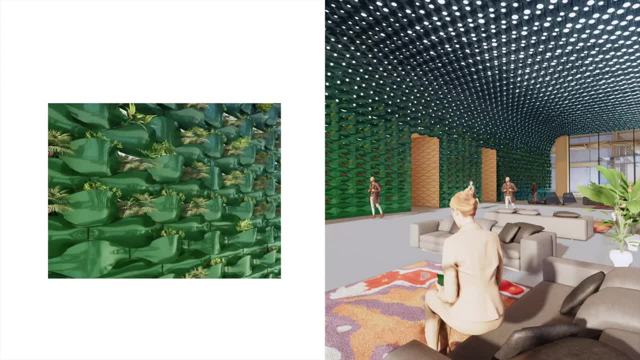 um looking at it. so you have that seamless transition from wall to ceiling. on the left you see a little detail of the plant cell and how it interlocks with the cell above it to create space for the plants. we'll show you more about that soon. here you are seeing the whole um. 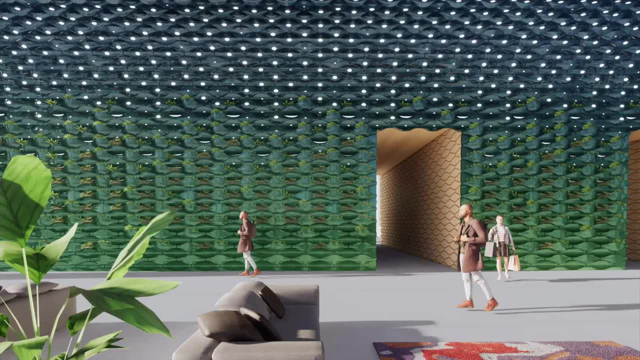 extents of the elevation. so you know, you can see all the cells are kind of working together. there's a robust grid, there's repeatability within each one of these types of cells. i think in the end we have only i think we have- eight different cells that repeat. 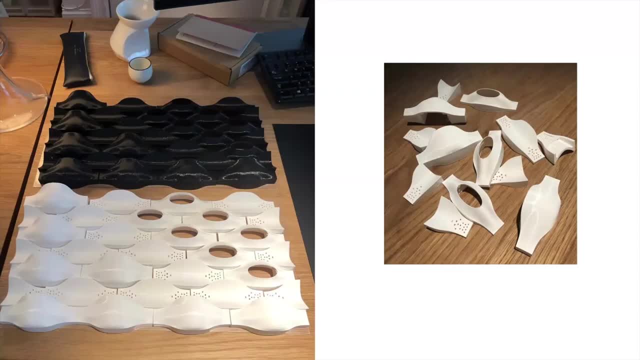 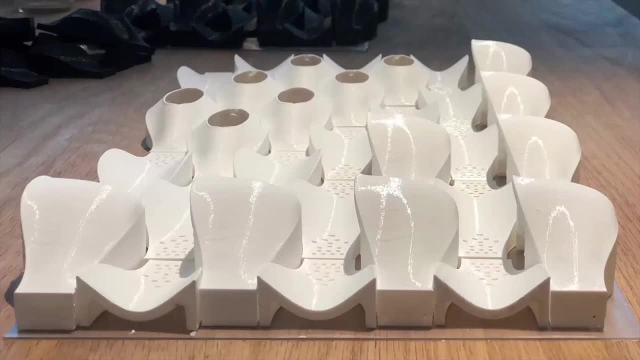 uh, we 3d printed them and started to see what kinds of patterns could emerge by combining them next to each other. and then we also had to um make sure that all the micro adjustments we were making in the interlocking actually worked the way they were. 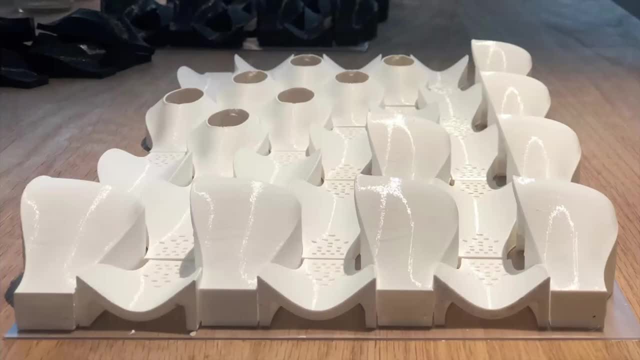 supposed to, so you can see um. on the right there's a cell that kind of cups out and that is a plant cell, um, so you need to have space for all the plant material. so we were able to carve that out so it pops kind of out, but the cell that's directly above it. 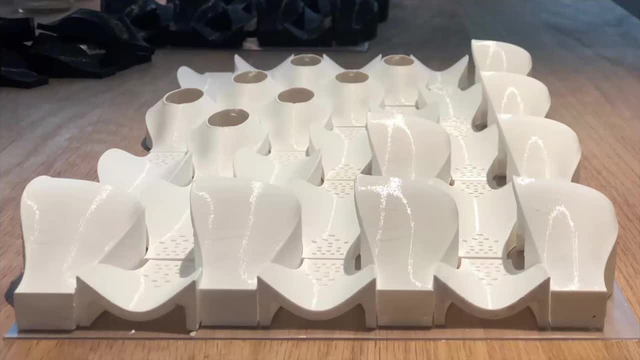 can't pop out as well, because then you wouldn't have space for the plant, so that that cell cups back. towards the back of this you can kind of see those digital screens popping out, and we had to do that so that we can optimize view angles for the digital screens. 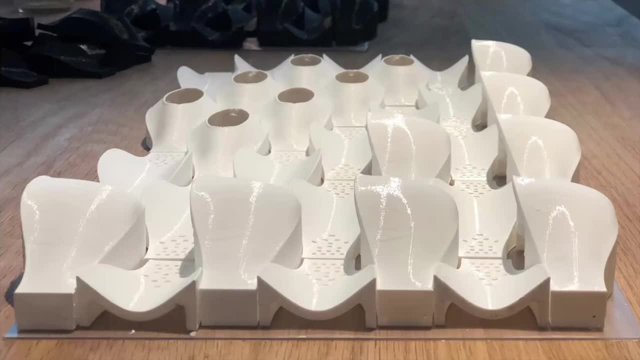 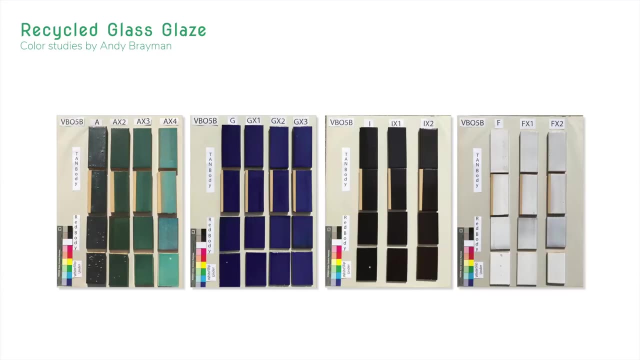 so in a way it's performative, but they kind of have to all work together. these are some early studies that andy sent us of his experiments. he sent us many more like maybe three times as many, but the ones that we were thinking about um were really the gr, the blues and 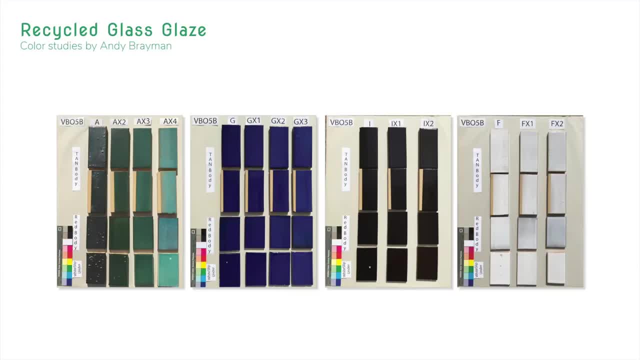 the greens, we had this notion that it would be amazing if this wall wasn't like a charcoal. it would make the plants really pop. however, we thought that might be a bit oppressive. uh, over the full extents of the lobby. and then white: certainly beautiful, you can accentuate. 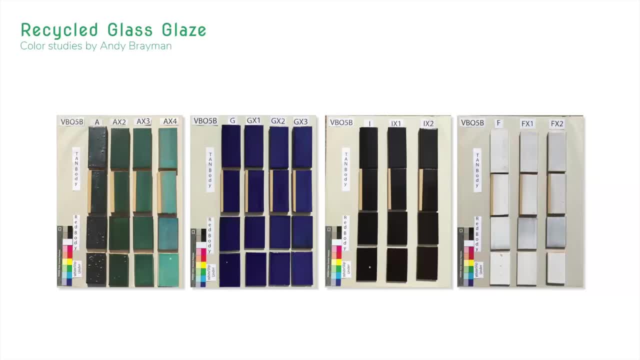 you can see the form in the light and shadow, but maybe a little bit too expected. so we um honed in on the greens and the blues. we kind of had this idea that if we remap it in a smart way, uh, we could actually make something more out of it, which means that we 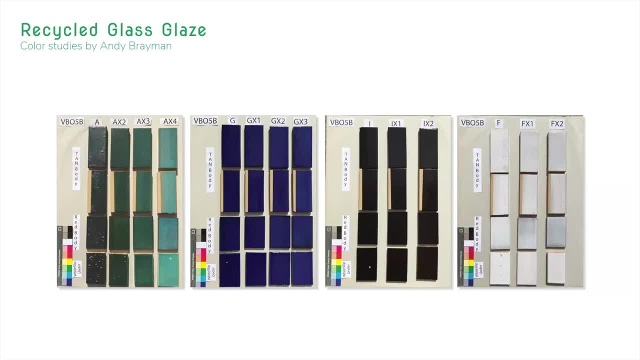 made the plant cells green, um, so that even if a plant dies- which, as you know, in a green wall happens, uh, and there's also a time lag between when it, you know, passes and it gets replaced by building maintenance- um, anyway, that cell would continue to be green because the glaze 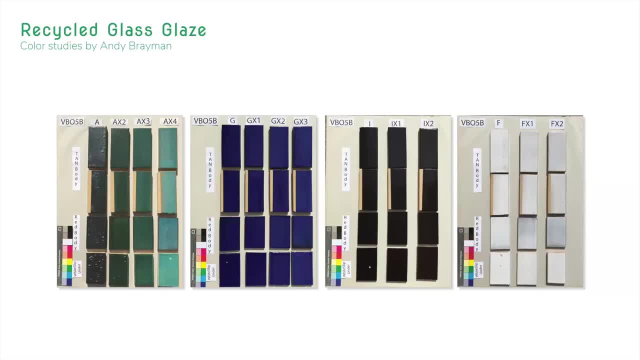 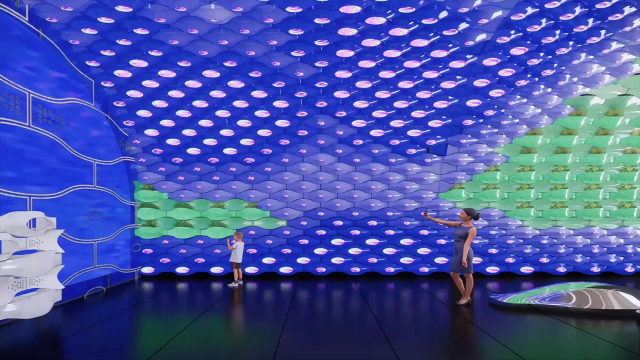 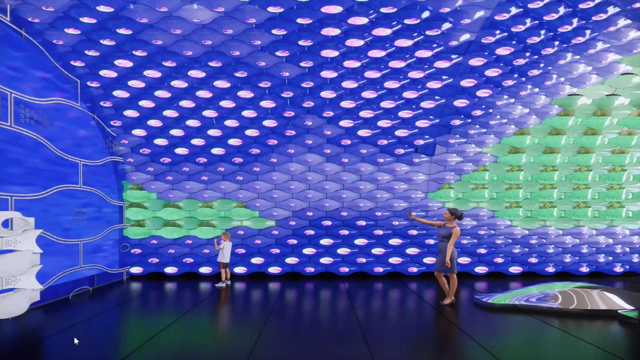 is a beautiful green color. so, um, that was kind of the start of our gradient. and then blue is our digital screens, um, and we pick that color because, um, it would interact less with the light. so here we are, here we go, oh, sorry, sorry, okay, um, here we are in the green wall and we're going to take a look at the green wall and we're 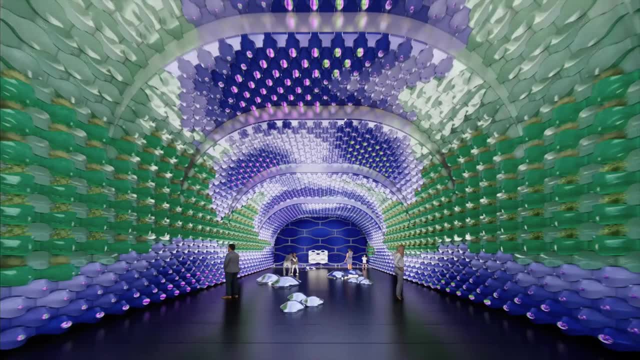 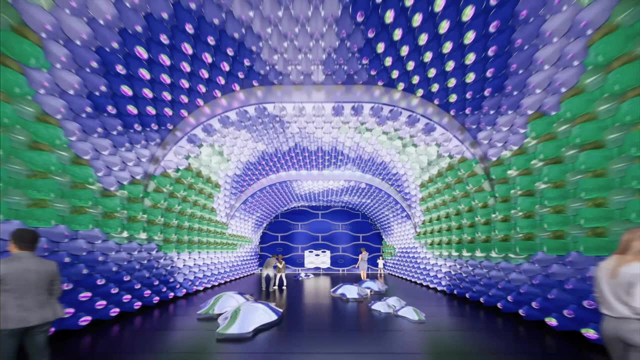 going to take a look at the green wall and we're going to take a look at the green wall and we're in the nonagon and, um, you're entering this tunnel of terra cotta and we were thinking about this as a sensory experience where you would see changing light, um, changing color. you would 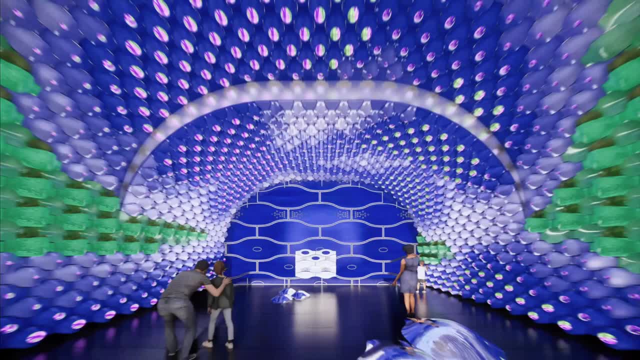 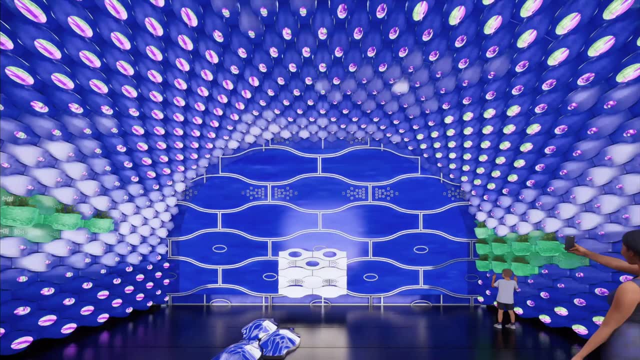 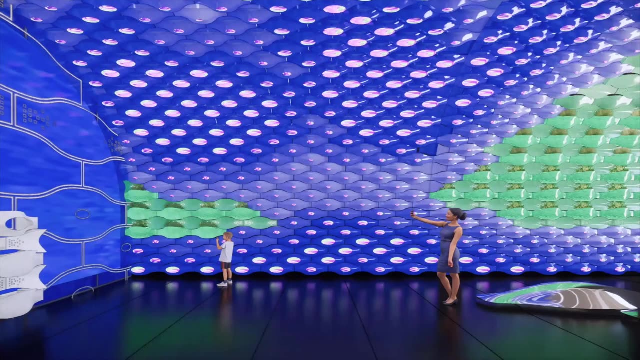 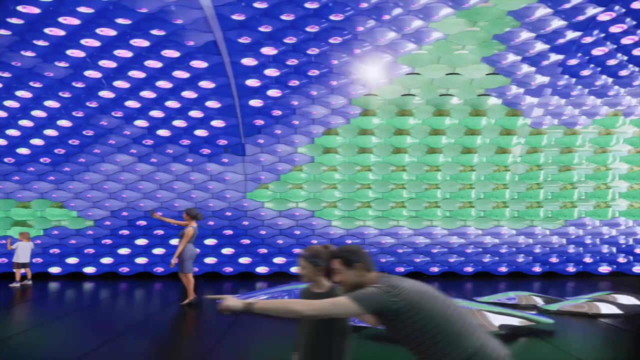 smell the different scents of the plants, and there would be an oral component because there would be embedded speakers. so maybe you're hearing some water or wind here. you are panning across. I think in this, in this view, you can really see the difference of depths that are achieved. 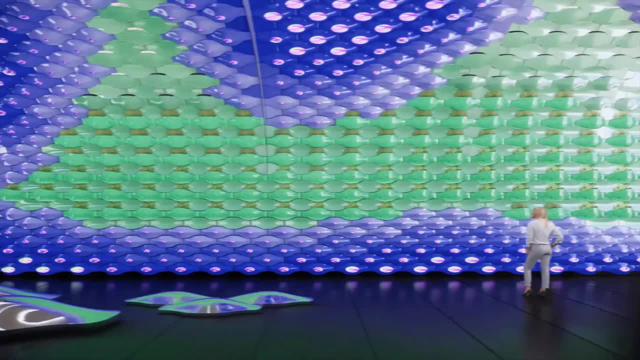 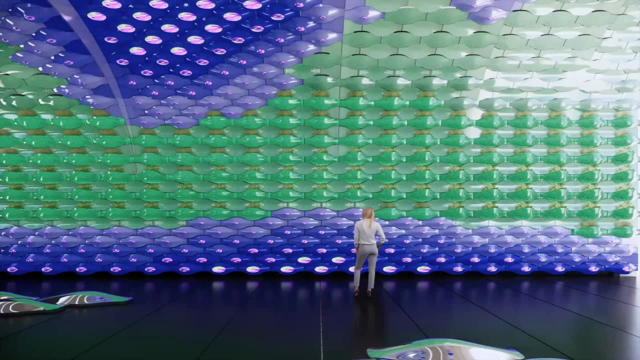 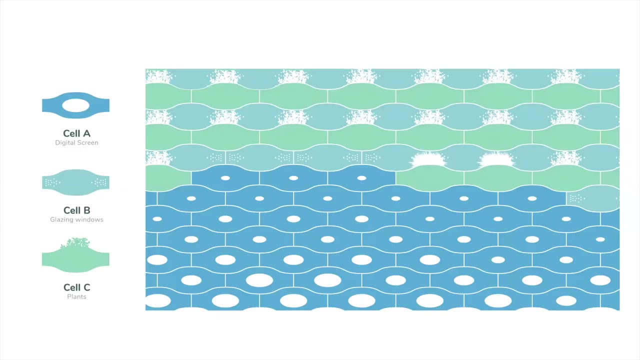 through the different tiles. like the reason for having depth for a plant cell is complemented by the, the light module that's behind it, that needs to curve back. hi, guys, for the next part I will go through our prototypes. basically, we'll have three types of cells that form up our entire. 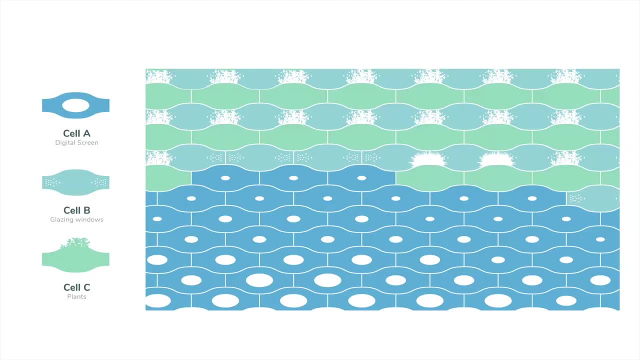 feature wall. the three types are a digital screen, be glazing windows and see plants. Sally has several variations on the digital screen. size. parameters that control the sizes could be anything like height or even specific passes. so B and C are staggered so that the glazing window with grow lights are right at the back of the plants. so this will 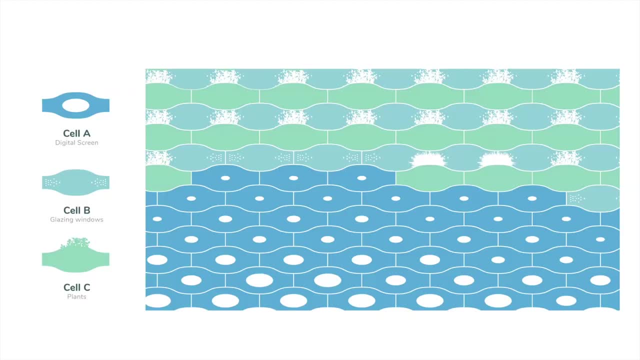 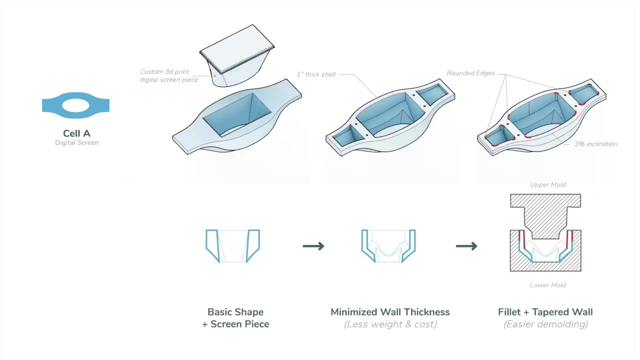 create, create a really good growing environment for the indoor plants, then I was could explain each type of cell in detail. next, please, here are some diagrams show how we generate our final detail for fabrication for the cell. a first: on the left there is a basic shape with a hole that 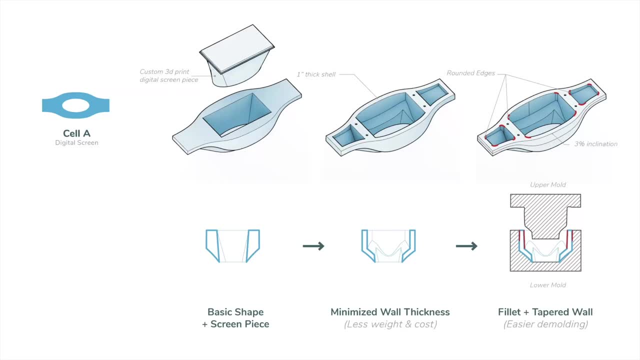 sees the custom 3d print digital screen bracket. we will put a rectangular digital screen on this back and then. in order to help minimize the weight and material and to make sure it maintains its original shape and structural integrity, we keep the shell as one inch thick and two ribs. 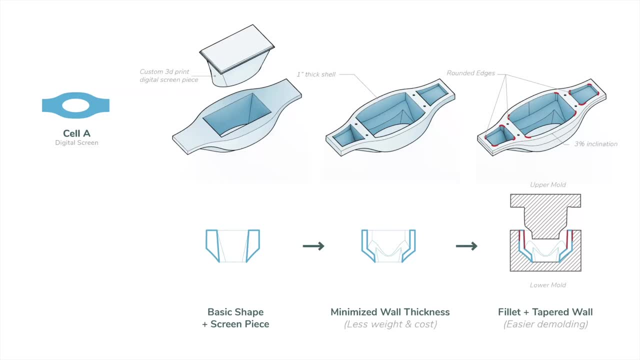 for future assembly holes are kept. and finally, considering mold making and for easier the molding, will fill it as much corners as possible and we tapered the sidewalls. and we tapered the sidewalls with 1% to 3% inclination. the last section shows the two modes that could be used for both the 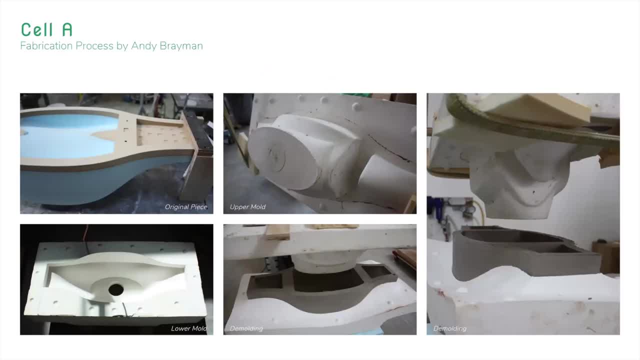 past and impressed. next piece. so here are some fabrication photos from Andy. the top left is the original piece that it made by the mill: full phone and MDF for the shape and based on the shape, he made two moles and then cover them together, pulling material and wait until it dries next. 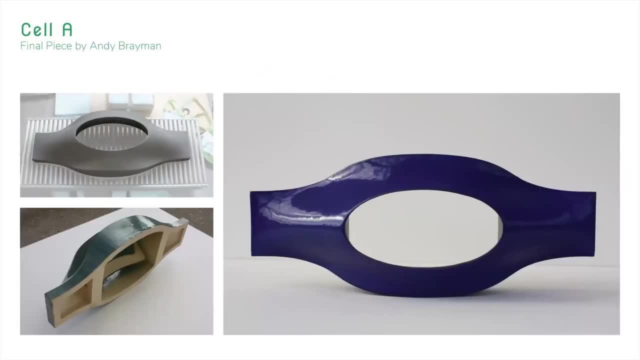 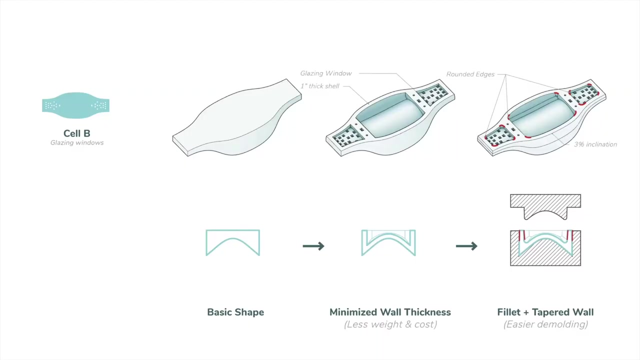 piece. so here we got the final prototype after coating with recycled glass glaze. for Sally. next piece- and this LB is similar- has a similar process as for Sally: minimize one inch thick wall and incorporate the glazing windows within the safe zone that one one is structural integrity and 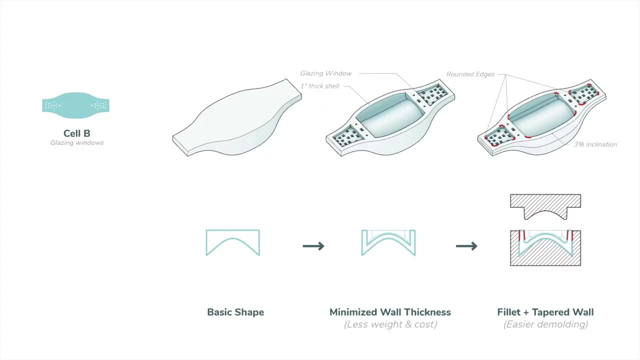 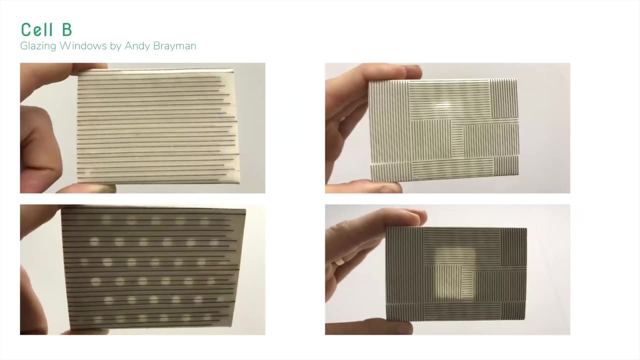 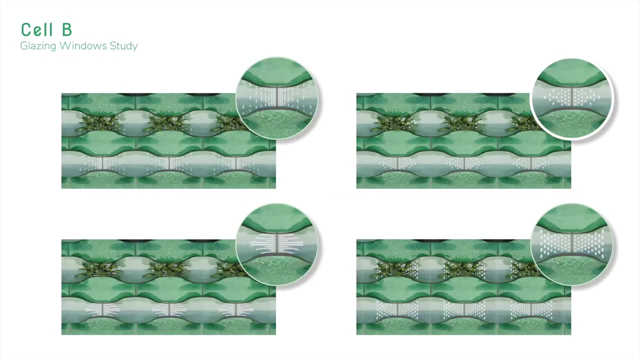 rounded edges, tapered walls for fabrication. next piece, and for this LB were highly inspired by Andy's artwork: the glazing windows, glazing span on the ceramic holes and lighting lights coming through- really beautiful. next piece, for designing the glazing windows on the side of cell B, we made several studies. considering the others might has more. 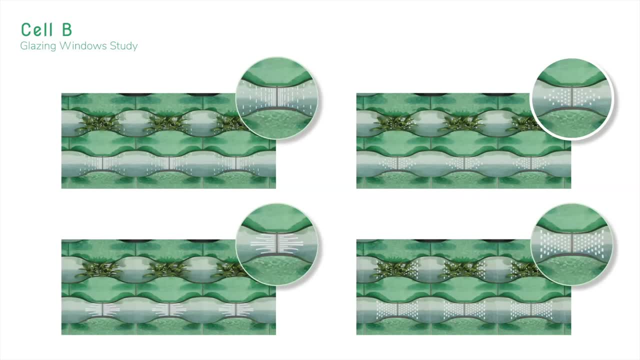 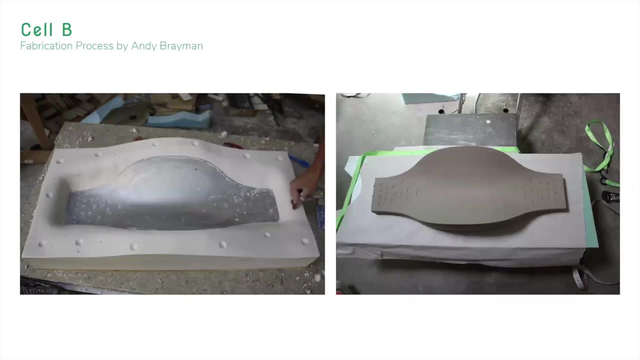 perforations near the edge which might compromise the structural integrity of the of the cell. we chose the top right. one next piece, so the slightest is about the mold making for selfie, and it's rocky's after demolding. next one, and this one shows the process on window cutting by Andy's exquisite head making technique. next, 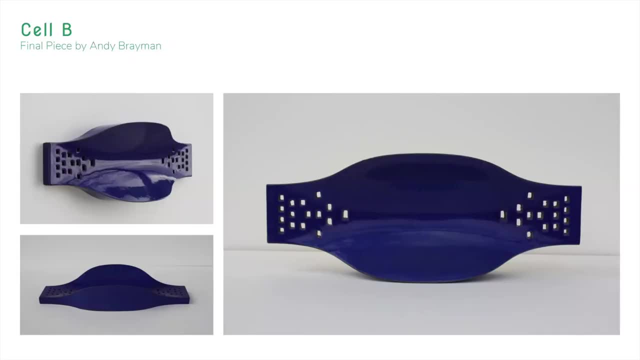 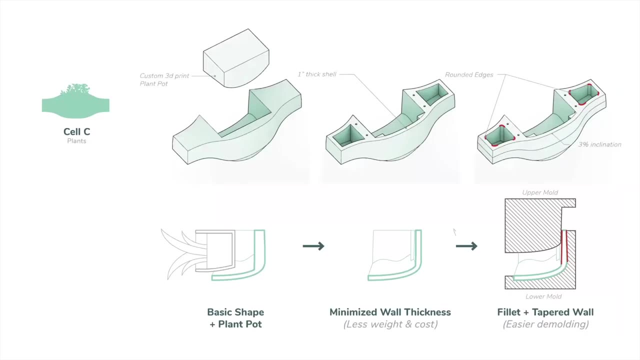 piece. here we got a coated final piece and the glazing window look really nice. we love it a lot. next piece and finally, the cell see a type four plants. funding is shaped by adding a 3d print plant, then modify the details by make sure it would meet the fabrication requirement we set before and next. 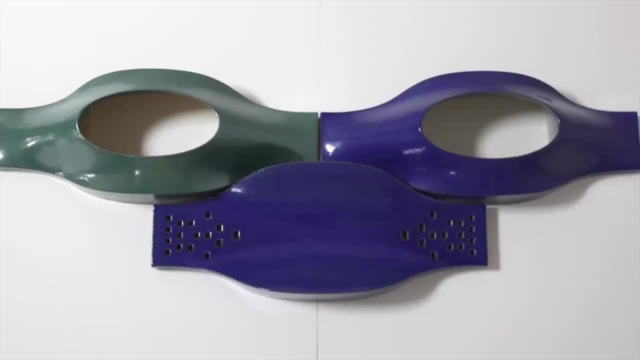 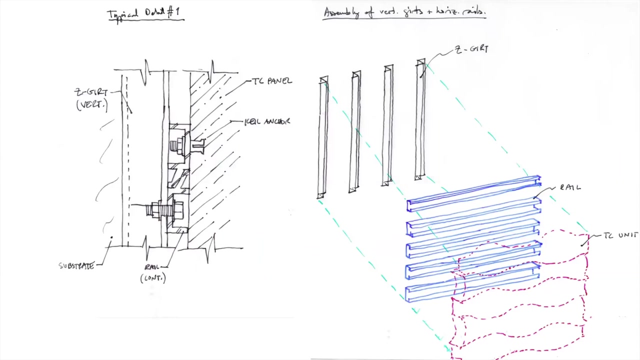 the final one. so here's the final look of our prototype pieces. the glaze highlight the gentle curvature and integrate itself within the environment. we love it a lot. thanks, Andy. thanks, thank you Chuchi, Darina and Marianne and um, thank you for uh contacting us about this project. we're 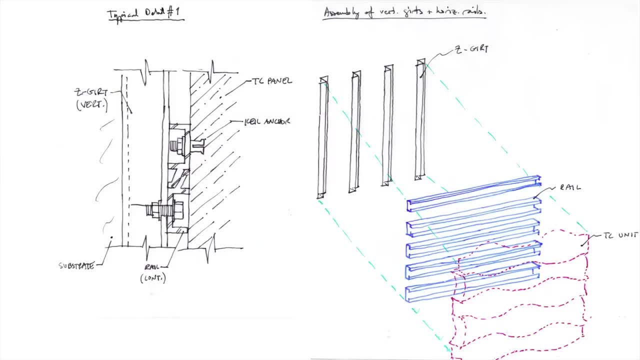 really thrilled when we were asked to do some engineering consultants in this, since we worked with, uh, with Boston Valley before we worked with terracotta, kind of future walls like this, um, so we already had some ideas basically as to maybe how the system could, could, best work, what 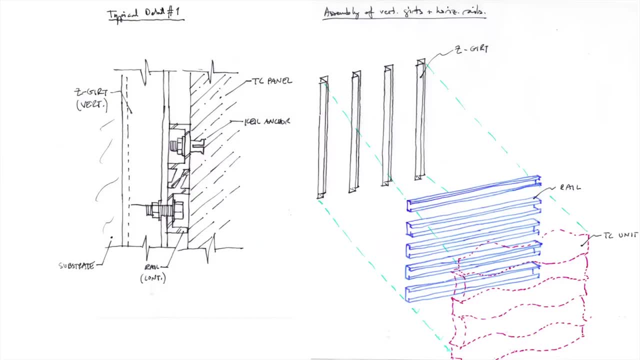 you see, here is a kind of typical attachment detail of a sort of uh French cleat uh or or a z-clip uh attachment between a um vertical, vertical z-girt that holds up a continuous rail onto which you then clip the um, the terracotta unit. that unit itself is held. 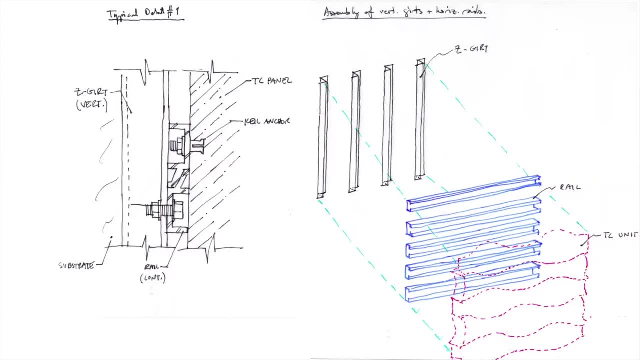 um with something called an undercut anchor, which is, in this case, made by a manufacturer called Kyle um, which we were interested in looking at uh largely because of the uh increased pullout strength you have in that sort of system over um other kind of rain screen type attachments. 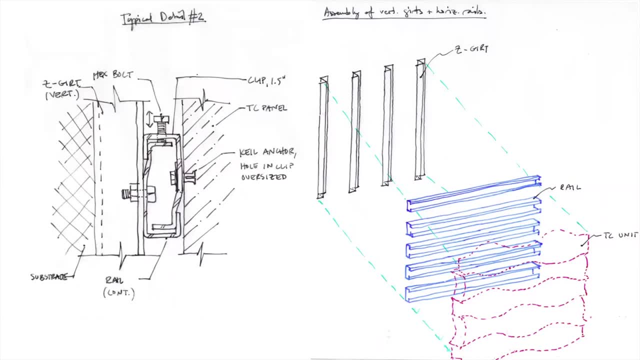 um, and it also um, early on was kind of became clear: yes, please, thank you next, next, please. it also became clear that, because we would have such a large ceiling component, um, uh, meaning overhead kind of horizontal terracotta, we wanted to make sure that we had a. 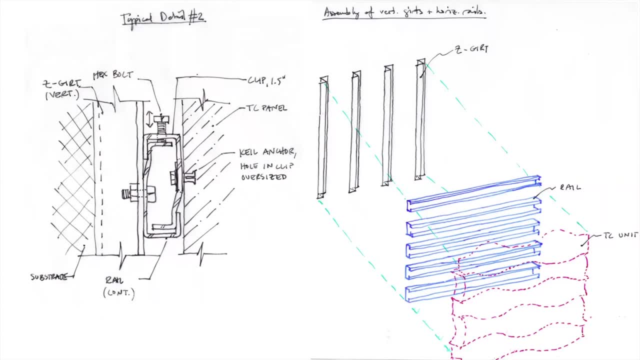 both a robust um kind of pullout strength, um study behind it, as well as a a clear kind of replacement strategy for the circle. and because these modules, as you've seen from from the team before, because they're kind of undulating nature of them and the number of cutouts- 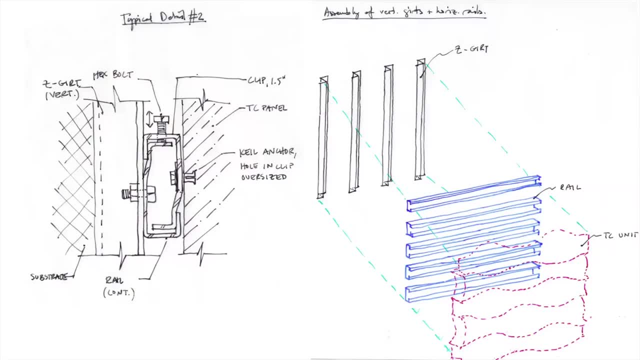 back. there isn't really a straightforward way that you can attach this sort of continuous, um typical rain screen, uh, rail, uh, with a clip, that that you may have seen on other systems, like the one used in one, vanderbilt, for instance, that was presented yesterday. um. so, therefore, we went with 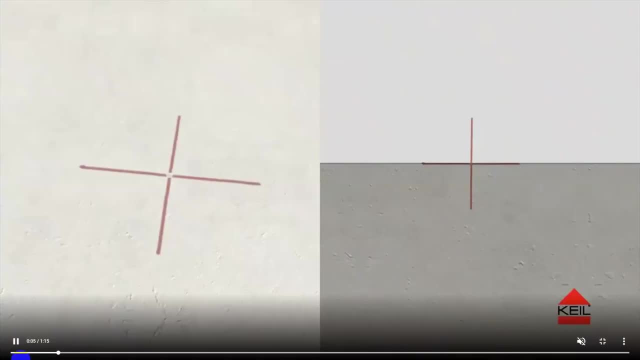 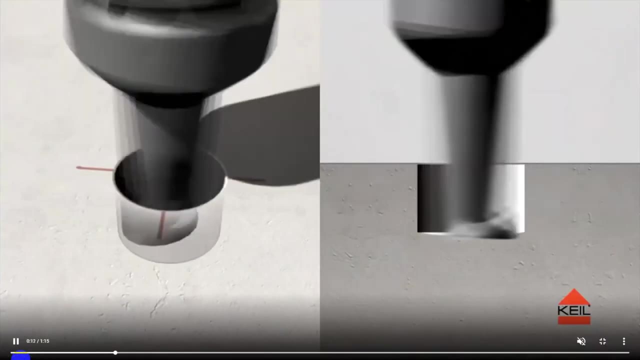 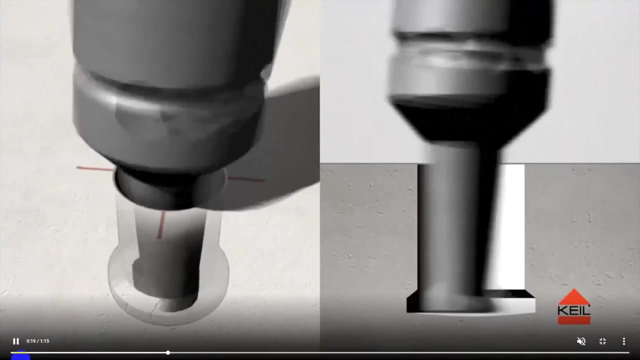 if you go next please. therefore, we went with this um anchor system, which basically is achieved by um, this kind of asymmetric uh mill bit that drills down to a very specific depth uh into the terracotta on the back. um, then it's moved slightly. you see how it's kind of tilting, so that actually, 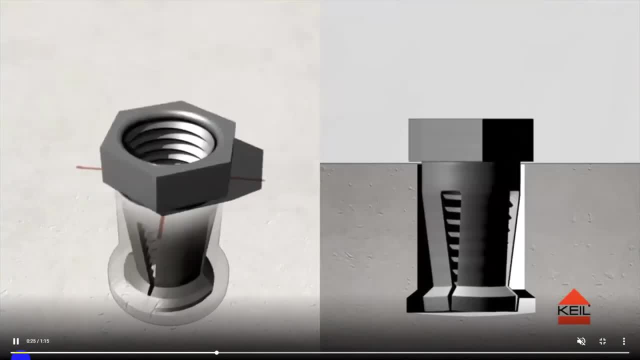 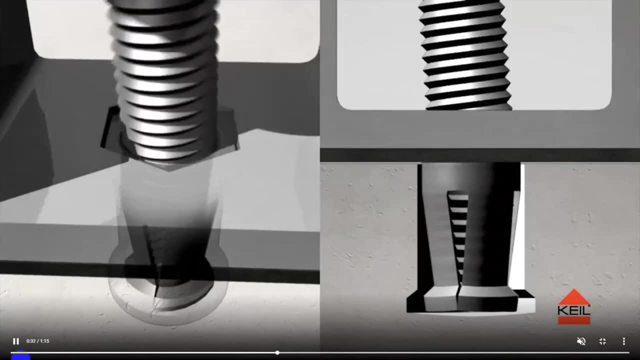 creates this undercut in one, in the same movement, and after that the uh, the expansion anchor is inserted and finally, it's uh, it's expanded by this, uh, this bolt, that's uh inserted into it. the difference to this video and what we are intending to do is actually, we have a 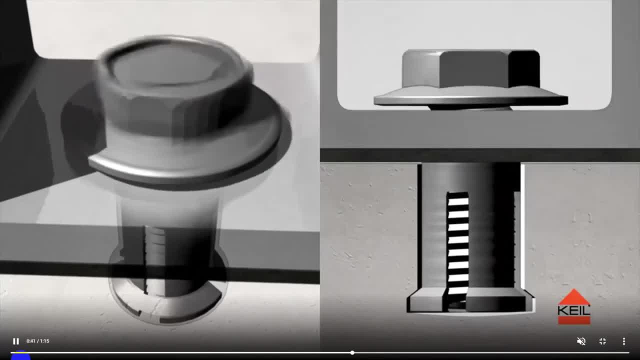 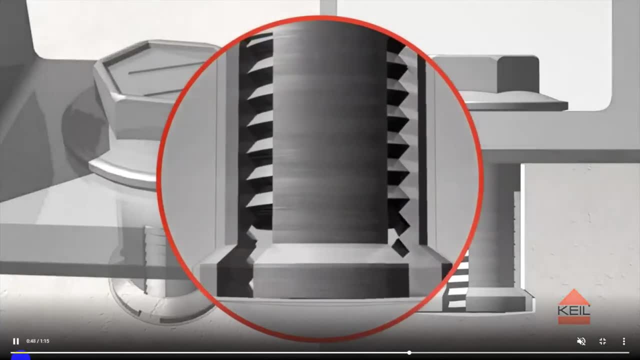 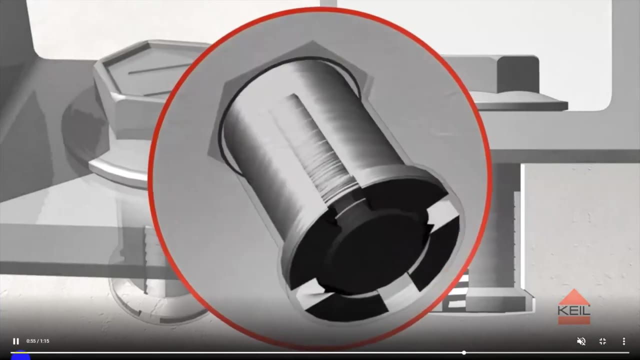 uh, we have a threaded rod rather than a bolt to the head, but in principle remains the same, and we also intend to uh to explore kind of the idea of an oversized hole with washers here, so you can actually do some some final, um, final positioning kind of in the plane. um, if you 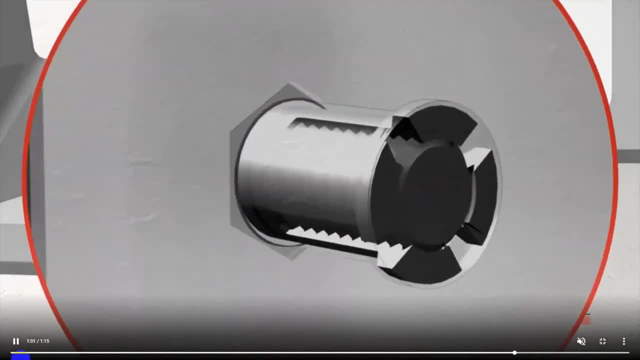 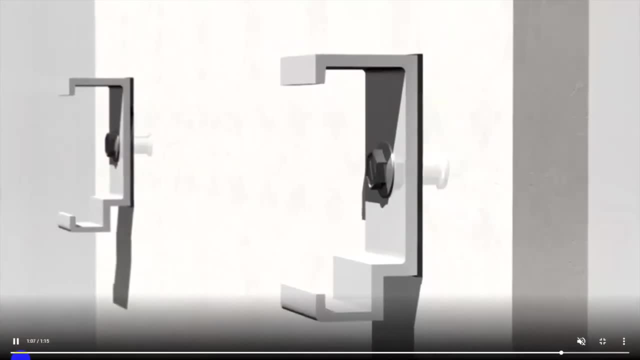 no, actually let's look at this to the end, because it has. it shows kind of how, the how, the non-continuous clip, what it looks like as well on the back of the panel. so, in difference to this, uh kind of typical bit that we're going to be looking at today, is that we're going to be looking at this? uh, kind of typical. 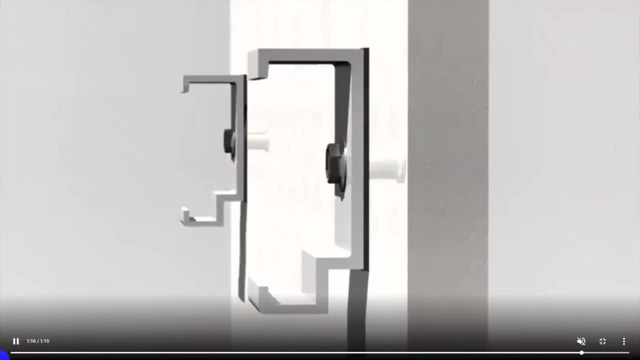 demonstration panel that kyle provided um. we have a very complex backside to this with uh with only very specific places because of the penetrations etc and the kind of routing of the um uh, of the electrical and the drainage uh systems where the holes can be, which is also sort of in favor of 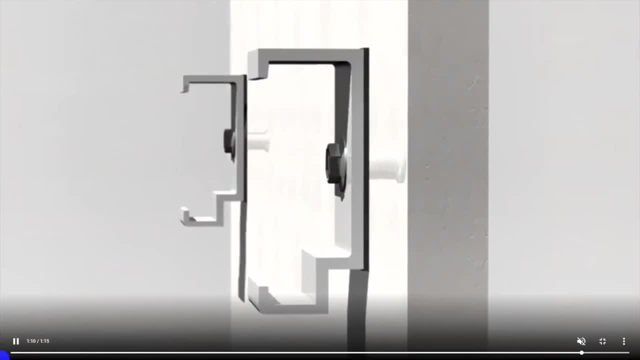 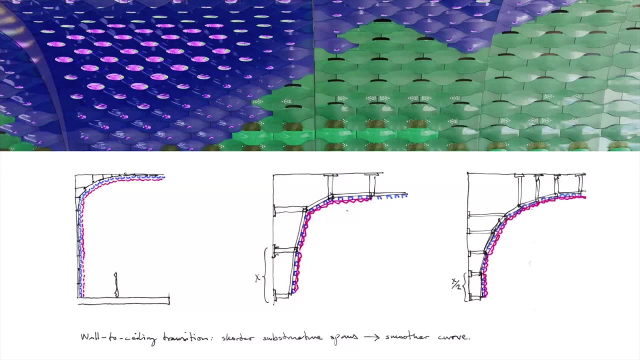 this system. so if you go to the next slide, please- and the other advantage, of course, of doing it in a potentially unitized fashion like this is that we can, we can- hang it fairly easily. we can, uh, we can- control the kind of geometries of transitions from wall to ceiling in this, um, curved fashion. 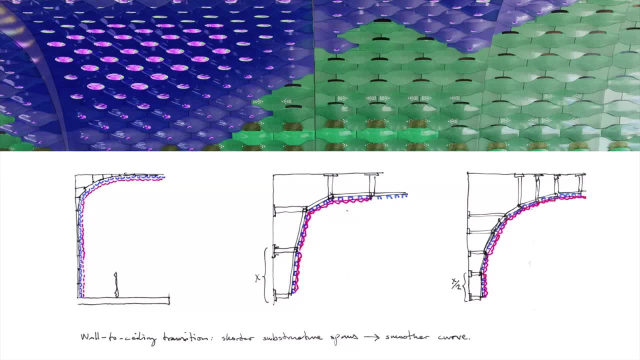 that kpf have envisioned. we would still potentially explore the uh possibility of curved z guards on the back instead of facets like this, depending on how tight radio we actually have to we have to achieve. but that's sort of a um you know, something we will be looking at in the further. 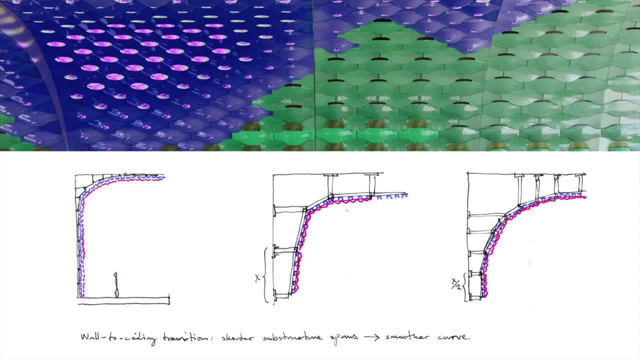 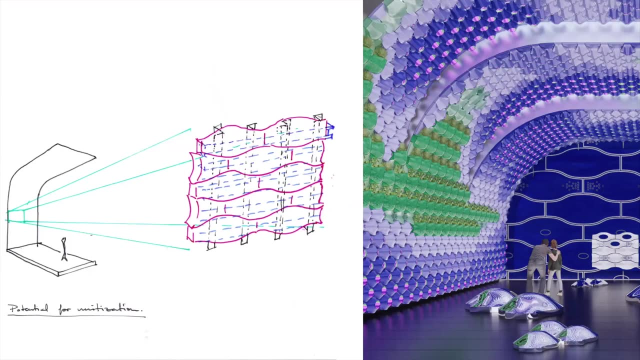 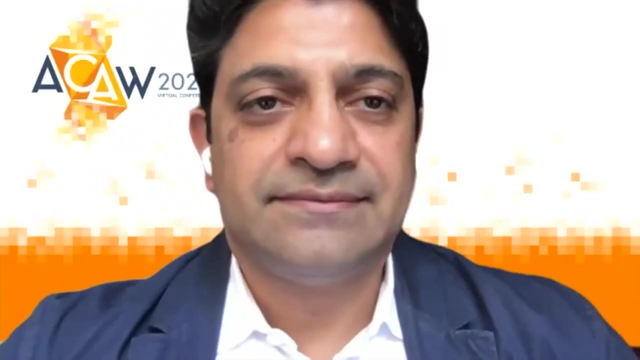 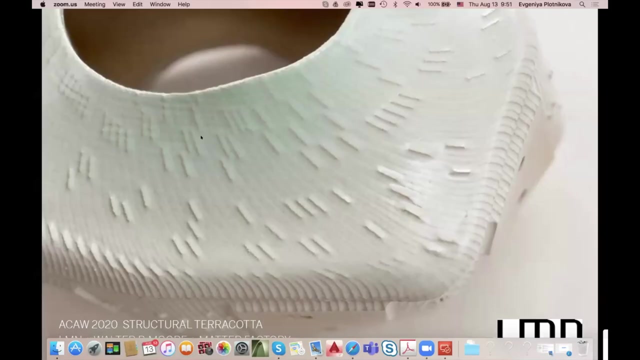 study, um, and then next slide. please, this should be my final one. i think you know we're a bit over time, yeah, so here you see, this is kind of a quick look at how, um, how this in principle, how this principal, uh, good morning, thanks, omar. my name is alex woodhouse, i'm with element architects and, uh, we also have 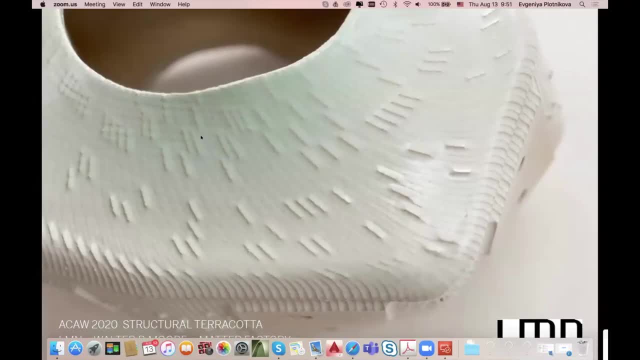 speaking today, uh plamina melusheva and evgenia platnikova, and i'd like to also just mention the other participants, uh stephen van dyke and scott crawford and vanessa abin um, and then we worked with walter p moore. 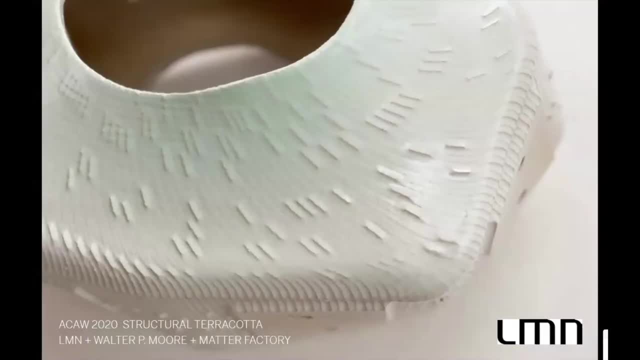 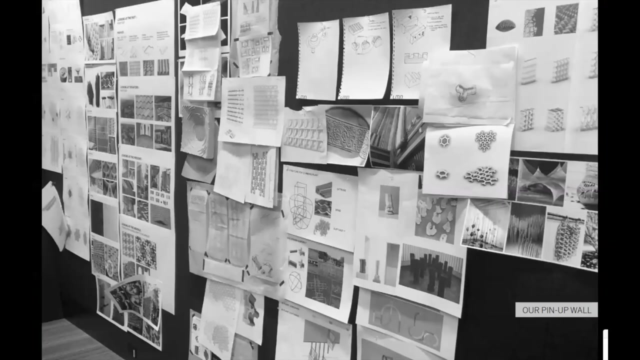 uh, norman richardson and laura karnath, and then, uh also, uh, jacob barkin, james renda and brian nickpon from the university of buffalo. uh, next please. so, uh, we started back in in december with a an open call for entries in the office and we had a wide variety of projects. um, looking at both. 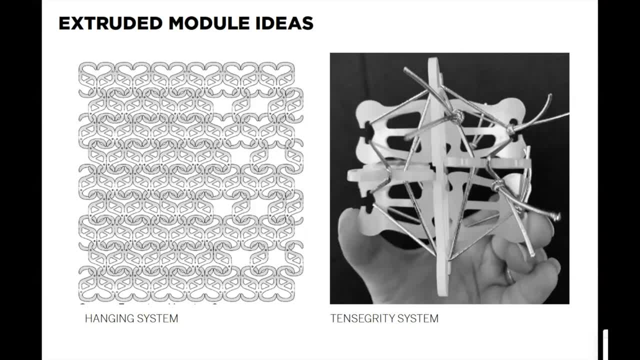 slip cast and extrusion. so, in this case, actually rethinking um the standard, uh, boston valley dyes and trying to think of a way to do that, um. so we're going to go ahead and get started and we'll go ahead and get started and we're going to go ahead and think of new ways of using them. 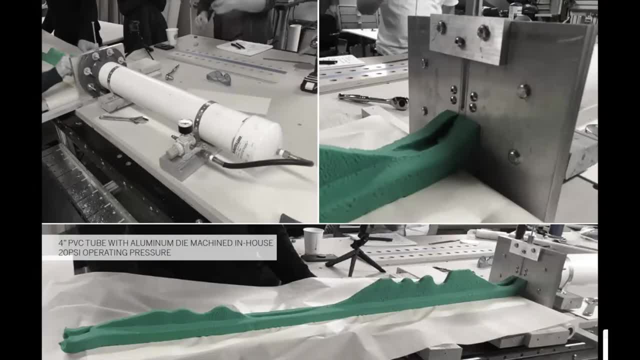 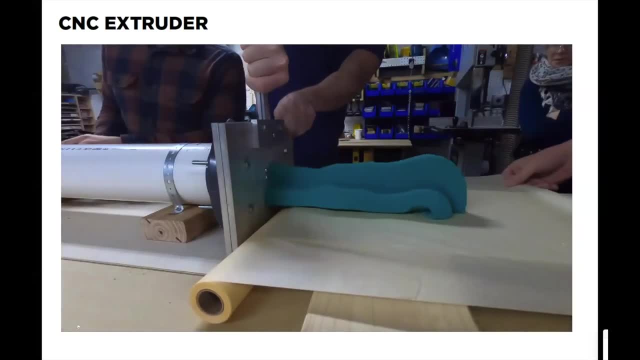 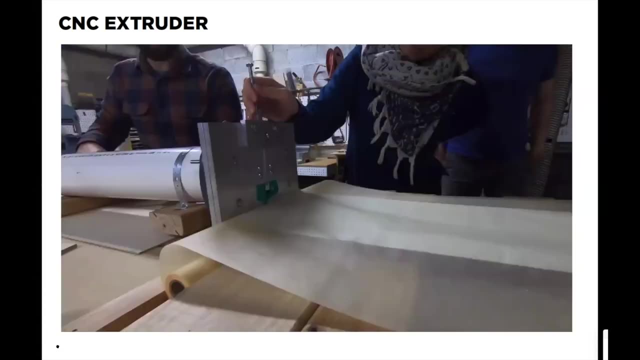 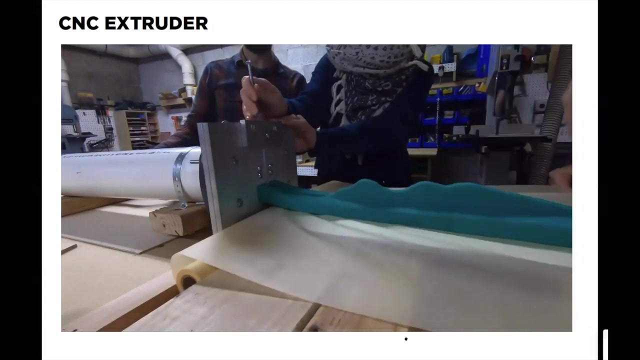 and then also actually kind of rethinking the extrusion process. in this case this is a proposed cnc extruder which would actuate a dye manipulation. just a quick video of one of these early prototypes in our office just to see some of the other ideas we were looking at um, but ultimately what we ended up. 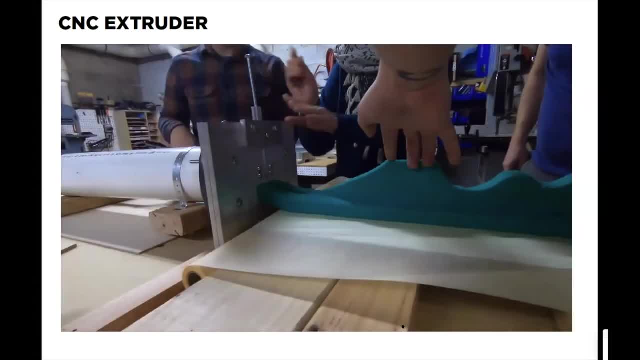 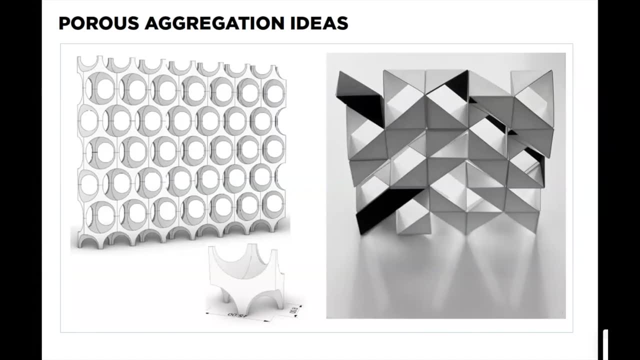 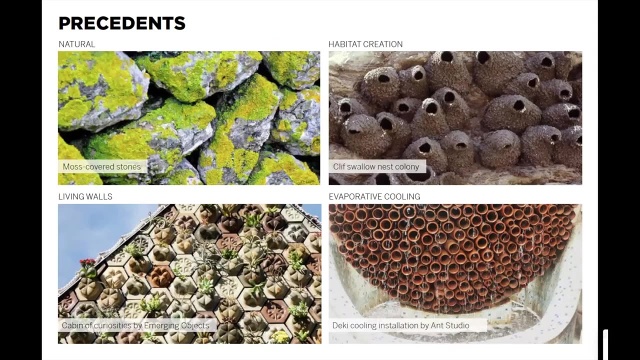 deciding to go with was more of a slip cast route. um next, yep. so the the idea was that we had a few different projects that were proposing more of these volumetric, freestanding ceramic assemblies utilizing one typical module on the side. we actually had a number of precedents which are consistent with other projects. looking 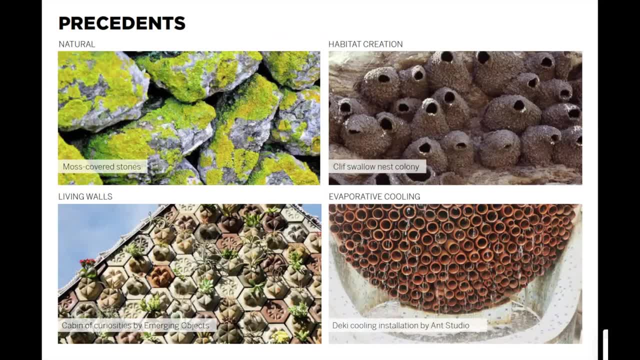 at um on the bottom. here you can see different uses of terra cotta as more programmatic elements, either as evaporative cooling, as Perkins and Will had mentioned, also looking at the more of a planted wall aesthetic, and then also looking at biologic reference points, like looking at moss. 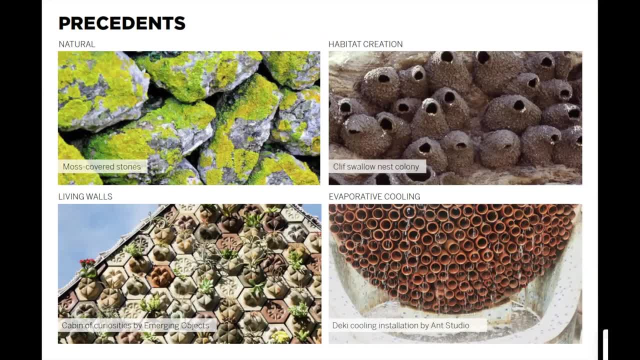 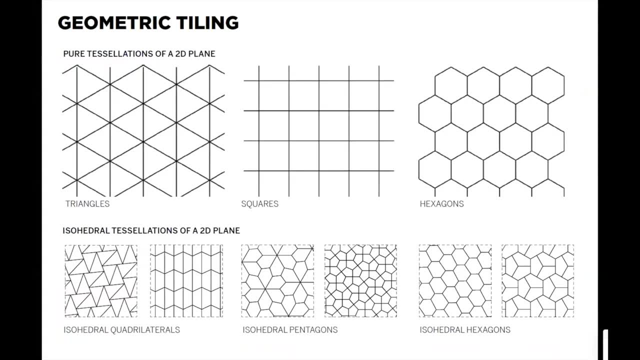 growing on ceramics and rocks, also the nesting colonies of cliff swallows. So then for the actual project we ended up going with, we looked at tiling of a 2D plane using a single module. So of course you have the top three, your pure tessellations. but then what was of more interest? 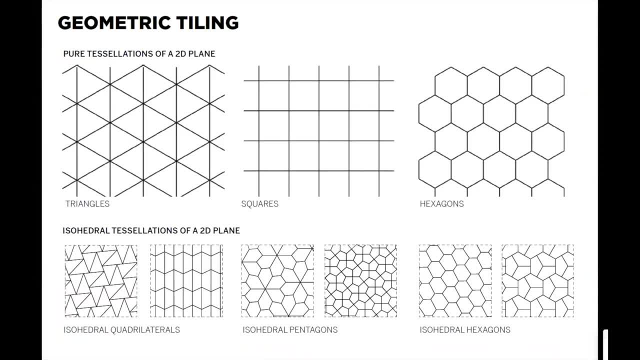 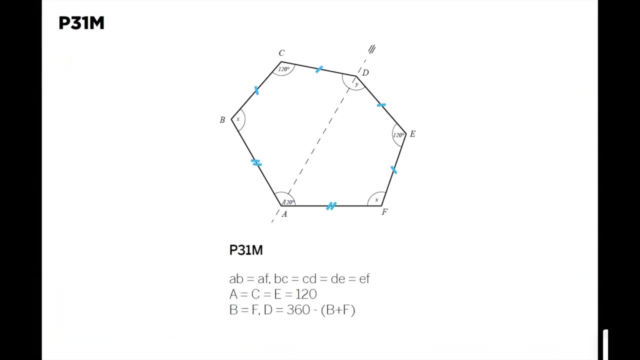 was actually the bottom row, starting to look at other shapes that can be tiled in a uniform way using rotational, mirrored or translational symmetries. So the module that we ended up choosing is called the P31M. It's a hexagon and it has four sides of equal length, and then the 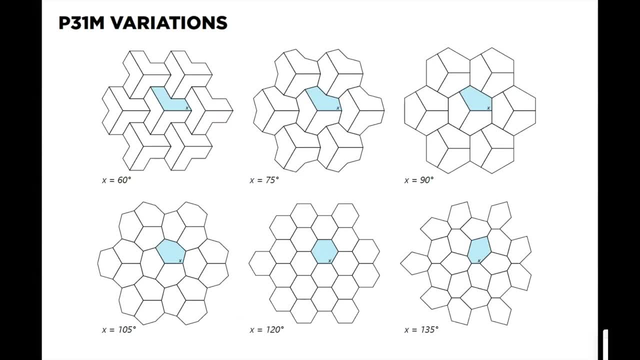 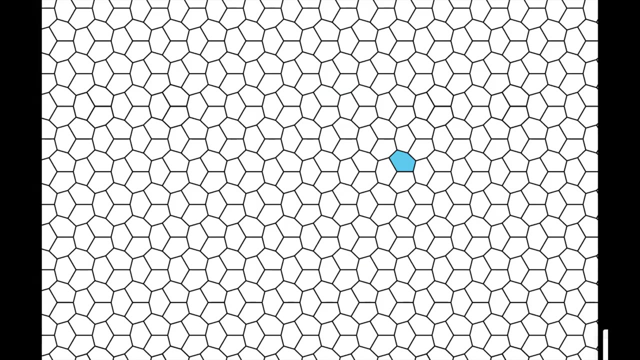 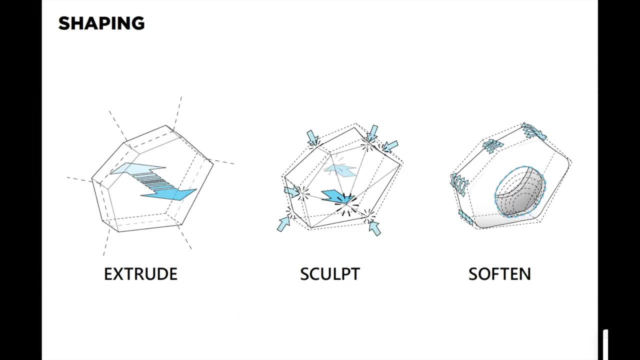 two remaining sides are of equal length And if you look at this next image here, you can see that within that module type there's a lot of variation And we ended up picking the bottom left as kind of our default cell organization. So here is the typical cell arrayed And from there getting back to the project itself and 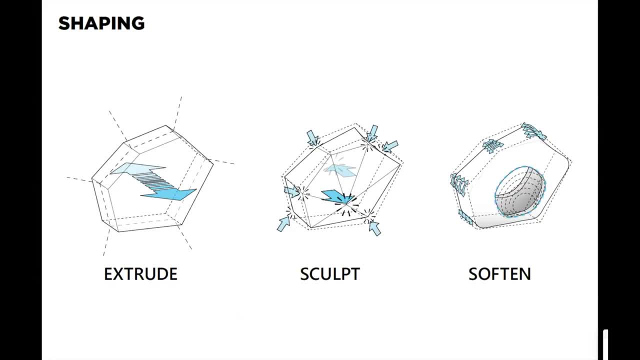 looking at more of a freestanding volume. we extruded this cell and we then slid it into the, started to sculpt it a bit, pulling out the two outward faces to give it some more depth, And then we actually tapered the waist, the middle section. 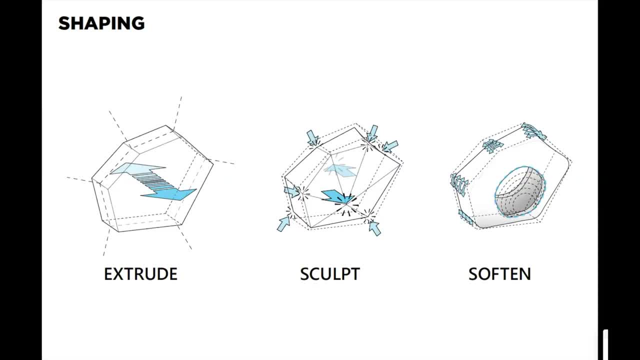 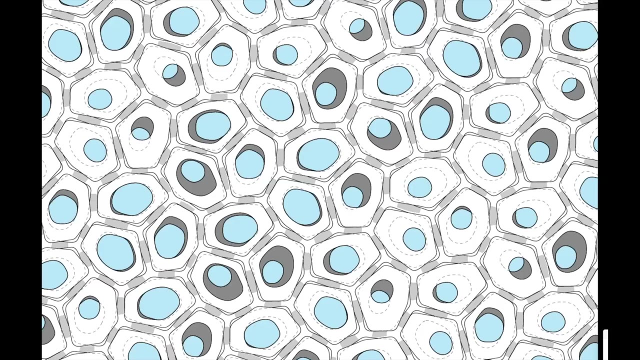 of the module. This is a strategy for more of a dry stacking assembly, which then kind of changed as the project developed. And then, lastly, we ended up softening the form and trimming out the face. One thing to point out on this slide. 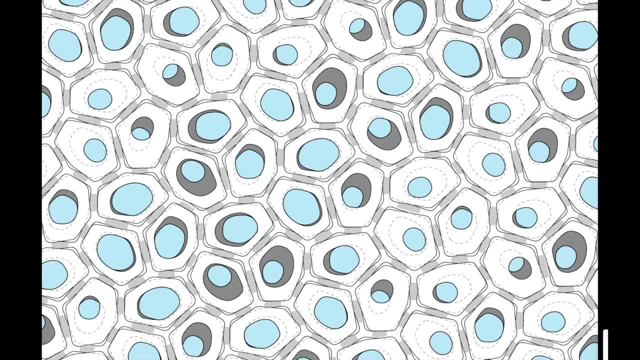 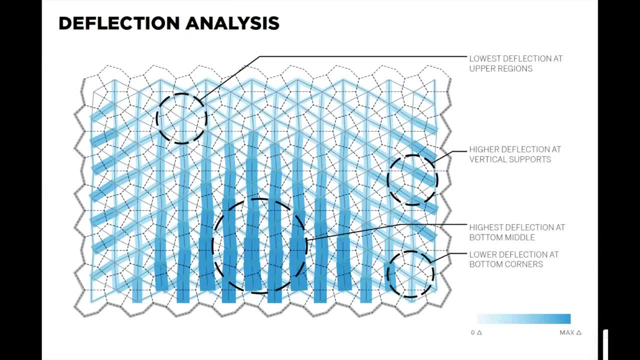 this is our kind of completed elevation, is to note the negative space that's developing between modules and then the spacer element, which we'll talk about in a little bit. One study that Norman, with Walter P Moore, had performed was looking at how this overall assembly deflects. 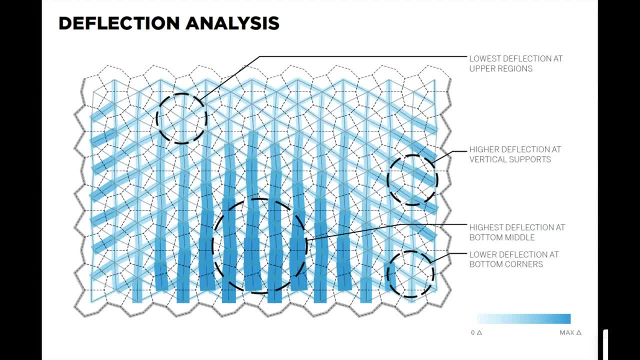 as a uniform aggregation. So imagine this is three sides supported. Of course, with the ceramic you would expect there to be a lot of load and, in this case, a lot of deflection occurring towards the base. But one thing to point out of interest. 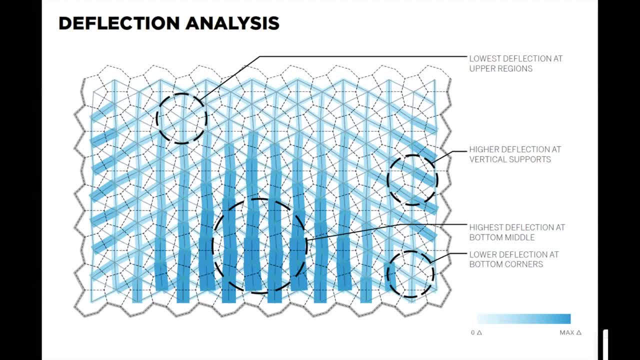 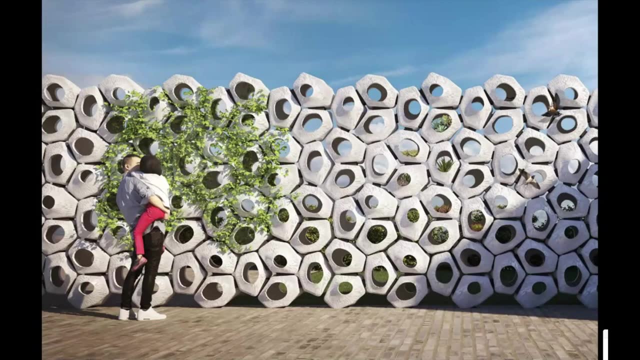 is the fact that at the corners here you actually have fairly low deflection relative to both the center base as well as the sides. So just an interesting result that occurred as we got into it, And here you can see just a rendered elevation of what this could potentially start to look like once you. 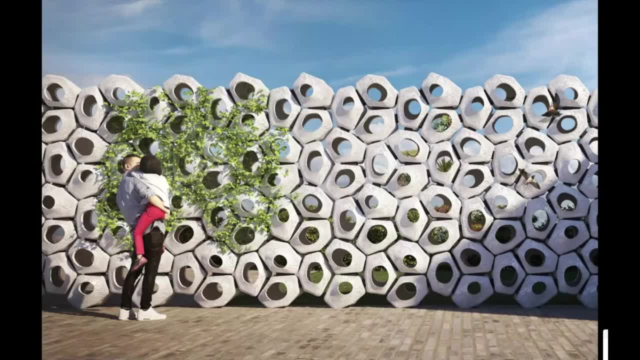 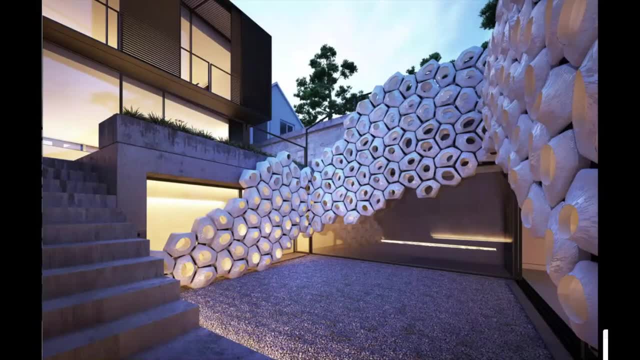 start to program the modules, whether it's vines and organic planting, Or if it's becoming more of an inhabited volume with animals, And then just a possible more aspirational image of how this could end up being deployed in more of a courtyard setting. 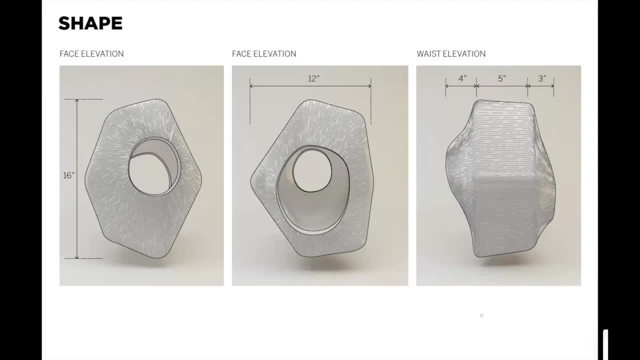 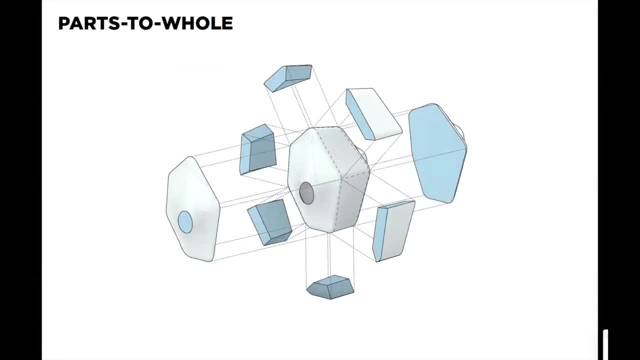 All right. So once we settled on the three-dimensional form, we started to think through some of the detail of it which was important for our concept. The first thing to figure out was to work with Andy very closely to come up with a way to divide up. 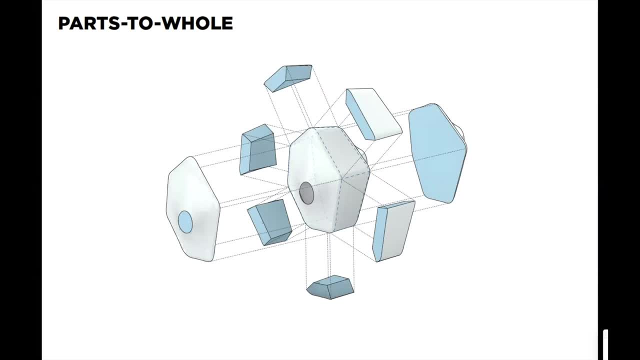 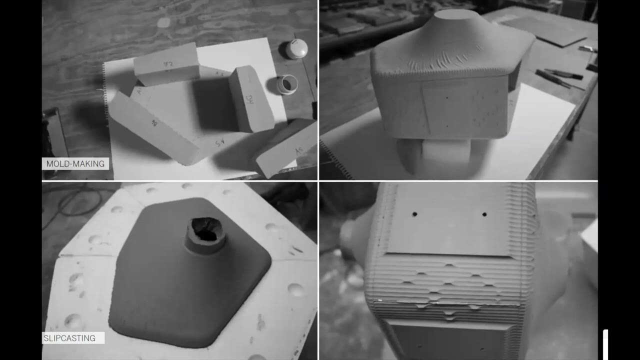 this fairly large volume into pieces for milling the master module. Since we were doing the milling ourselves, we had to take into account the z capacity of the element mill, And so this eight-part master module was sent to Andy, who reconstituted it as a matter of fact. 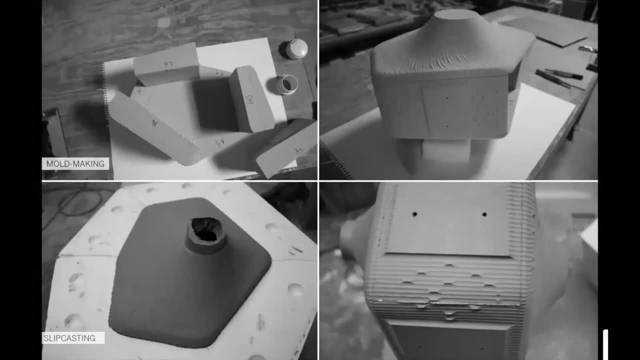 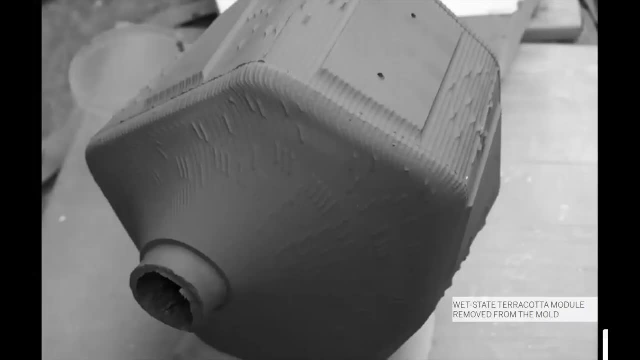 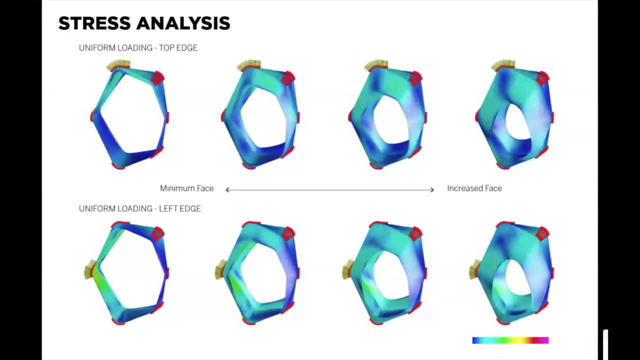 to build the plaster mold for the slip cast part, And so here you can see some of the process photos of that, the module, And this is the module as it comes out of the full mold. So the next piece of this was to figure out. 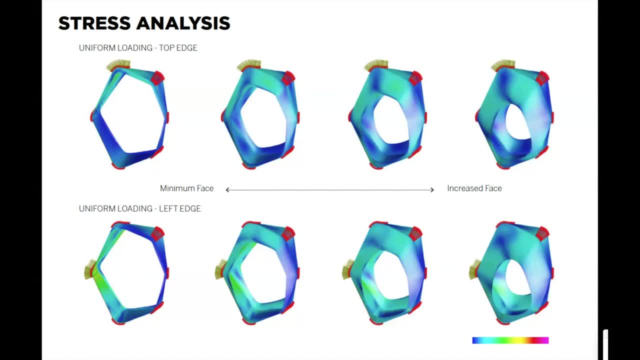 how to develop the openings. The opening was important for us for a number of reasons, So we worked closely with our collaborators at Walter P Moore. We worked with their team at the University of Minnesota to work through how large the opening could be. 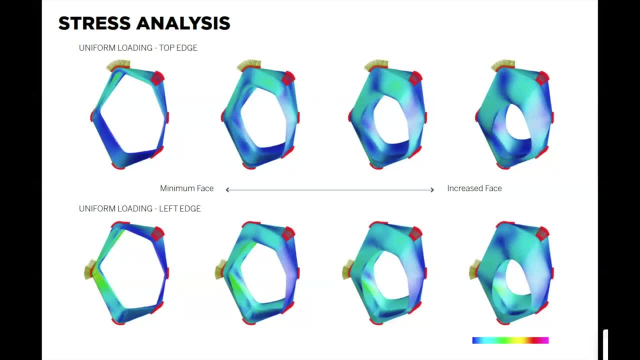 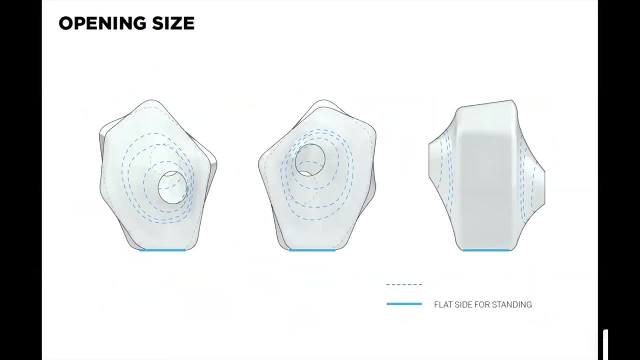 Based on the structural analysis, we realized that the waist of the piece is really taking all the load and in fact could take a stack that's at least 10 units high, And so then we could actually do whatever we wanted to with the opening. 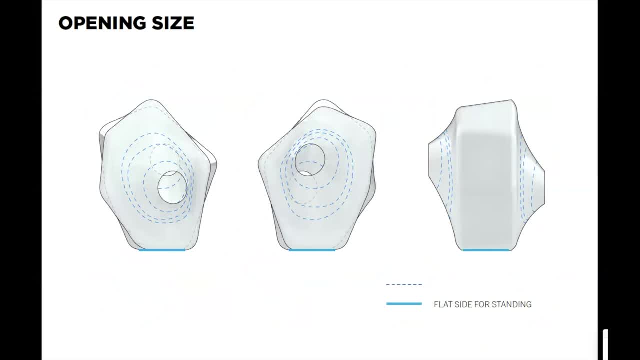 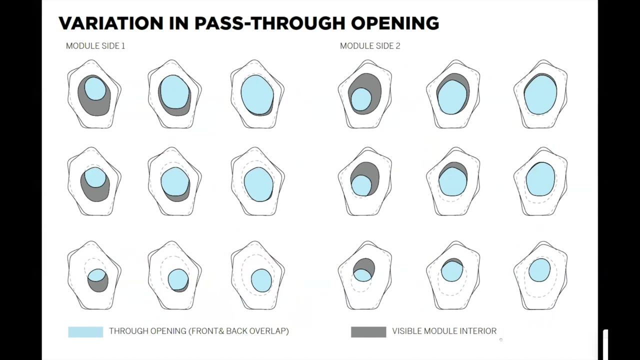 Next. So at that point we were able to design three different sizes that we felt supported our design goal, goals of some of the visual qualities of the piece. What we wanted to develop was a layered relationship between the exterior of the module, the interior showing through and then the through view, and to actually 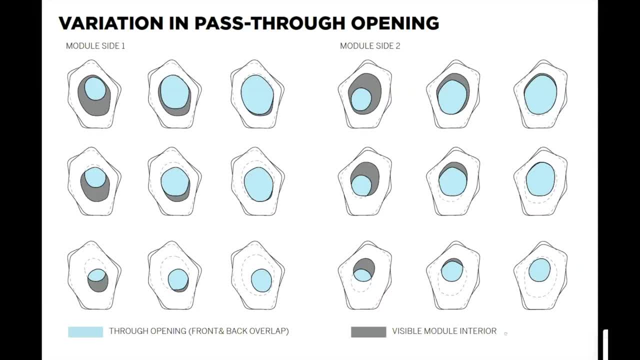 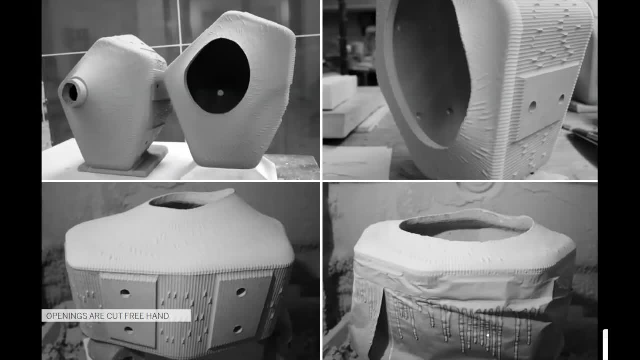 develop a range of options, as we have different openings on either side and this is meant to be really experienced from both sides. You can see in the top left photo the module as it comes out and then next to it one of the openings. We initially had the thought that we would develop a set of jigs for the 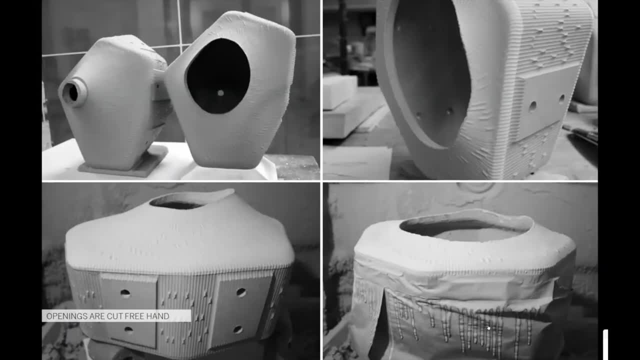 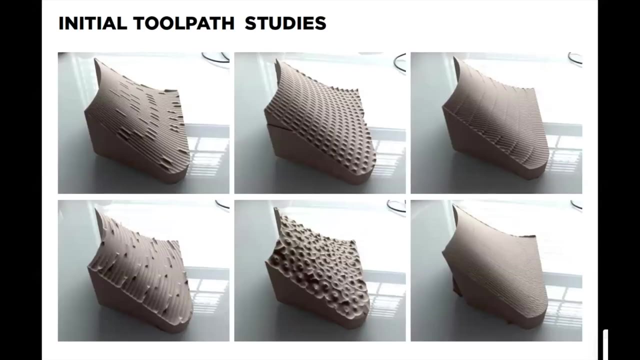 openings. but in working with Andy we determined that a freehand cut at the rough elevations that we had determined in our digital studies would be the best way to go here. So the next important piece in our detailed development was the surface texture, As we had studied some of the moss growth. 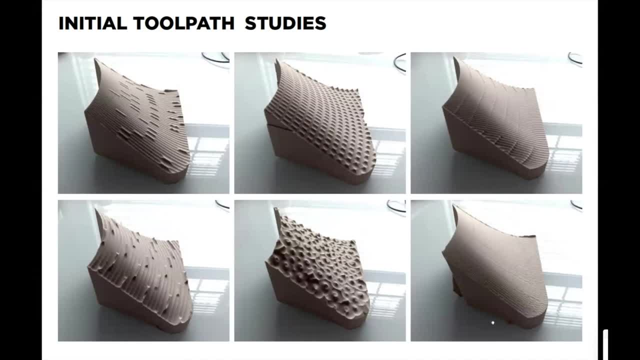 especially in the early 2000s and early 2000s, we found that the surface texture was a little bit different than some of the other bio systems. We wanted to create a texture on the outside that would support some kind of growth, and so we. 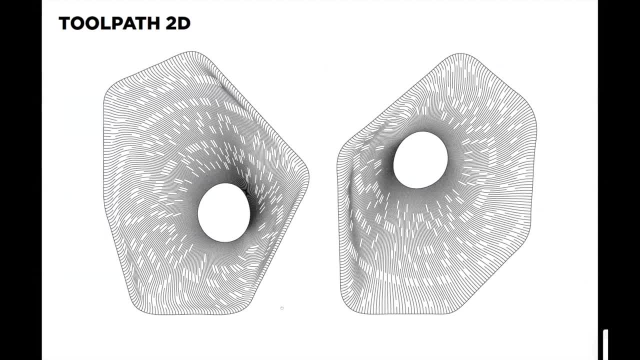 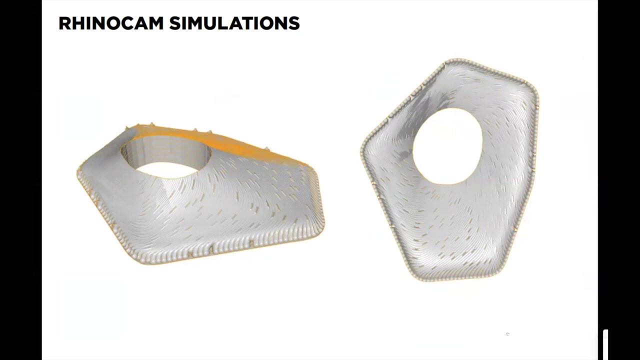 started with some early studies looking at different textures, and ended up settling on this radial twisted system because we felt that it fit most closely with the general design concepts of the project. There's also twisting and turning as part of developing the full system, So then we were able to simulate the line work in RhinoCam, and that was really the only 3D view that we had, because it only lived as a toolpath. 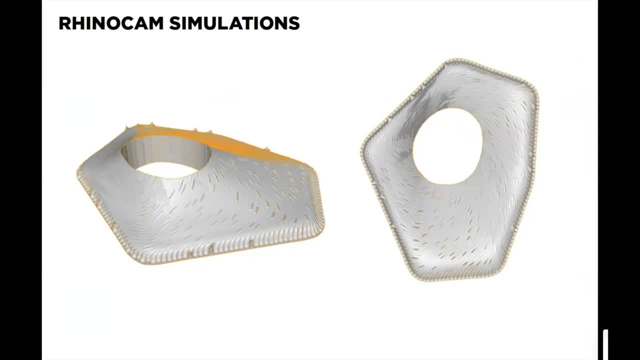 So the whole pattern is designed as part of just the milling process of getting the master module ready for any. It's not sort of a layer on top of that, And so next. So then, the first time we were able to really see what the 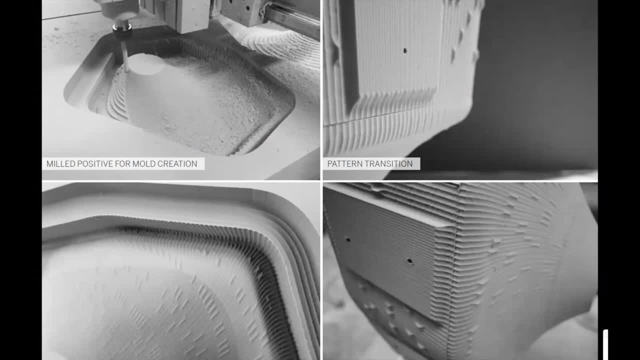 the pattern would look like as we were milling the parts to send to Andy And we had to actually think through quite a few details. On the upper left you can see that there's actually quite a bit of variation in the steepness of the part. 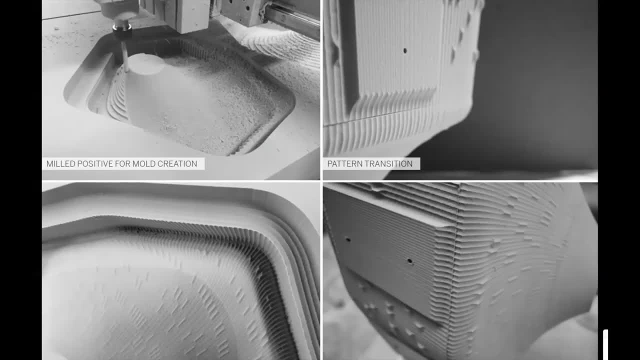 So I had to think through how that texture would play out with the geometry of the mill bit and the surface, And we also had to think through how the texture would line up across all the different parts that had to be reassembled together. So some fun kind of detailing there. 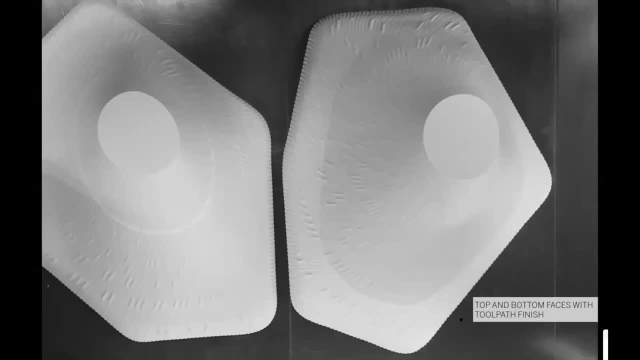 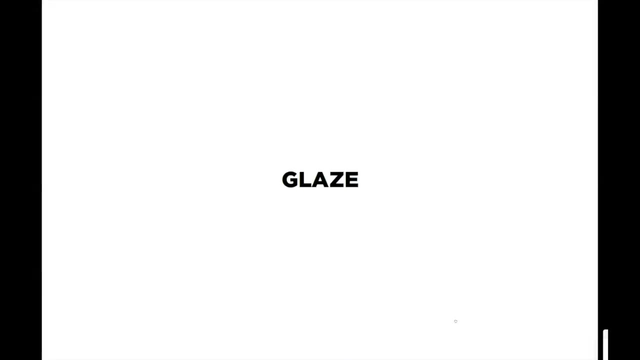 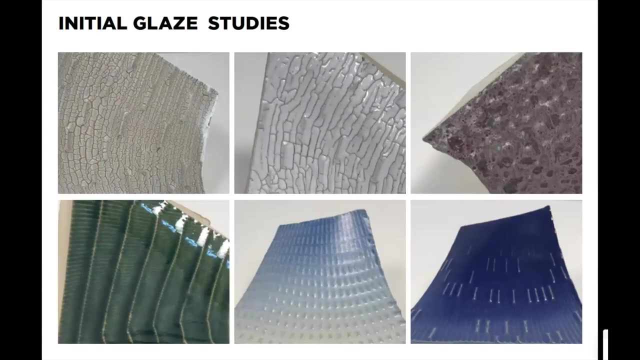 Next, And so this is the front and back faces before we send those out to Andy with the other pieces as well. OK, glaze. For the glaze studies. we wanted to explore three directions originally. One is the crawl group, which will 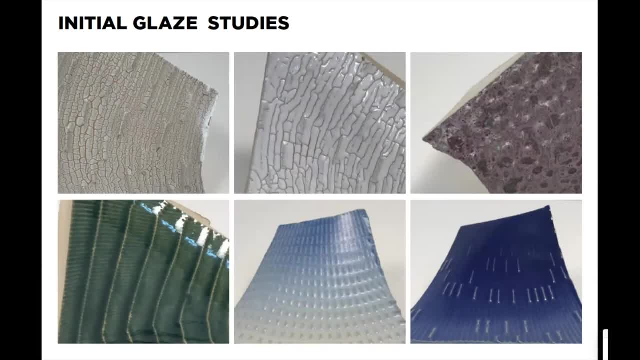 be creating this organic texture overlaid with very digital texture that we milled. The second group will be the volcanic group, which you can see on the top right. That will be about creating a really expressive rough surface so potentially the moss could grow on it. 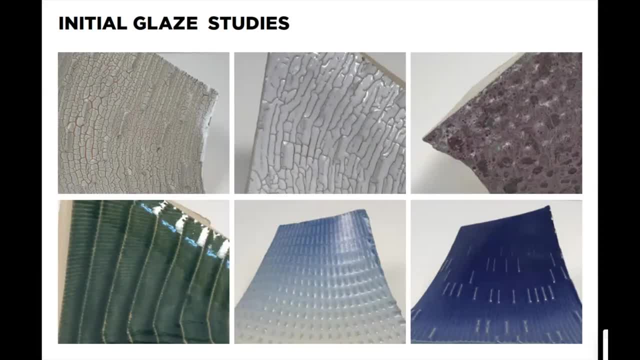 And then the bottom row would show the groups with a runny glaze. that would really enhance the CNC mill texture by the glaze pulling into valleys and the peaks getting exposed. And also we wanted to enhance the overall shape of the module by creating a gradient, color gradient. 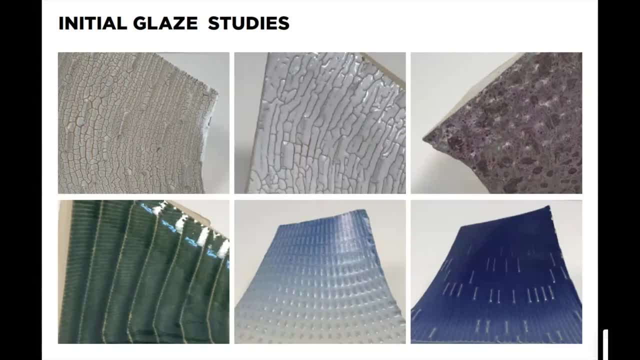 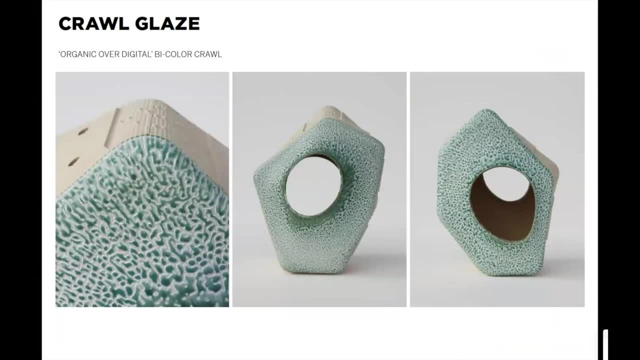 that would radiate from the opening, from the rim outwards. These studies, They were done on the relatively small pieces And, sure enough, when you glaze the overall module and it gets through the firing, you get the unexpected results. So one of those results is: this is the crawl group. 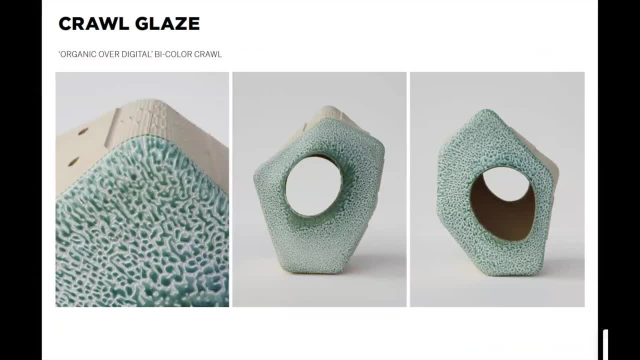 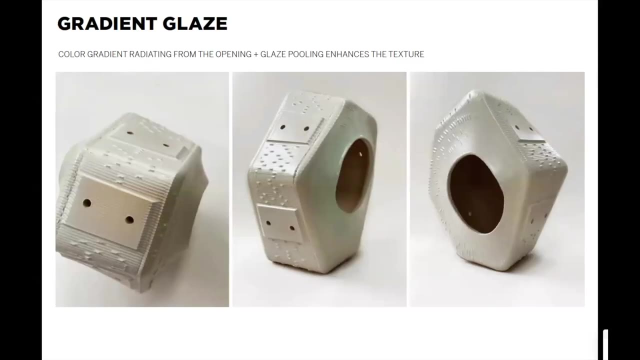 Andy apparently did use the bicolor, which was green sprayed over the white one. In this case the texture of the glaze itself sort of hides the CNC texture that we had. Second group is more gradient, So this is a good idea. 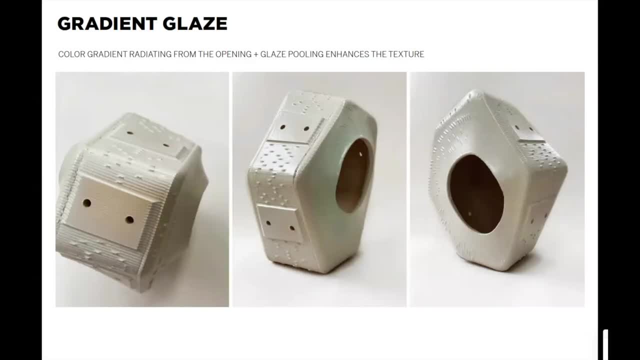 Here the entire module is glazed, versus the previous one where the waste was left unglazed. You see the green gradient radiating from the rim And you see some of the machine and how the glaze is pooling in this valleys to really enhance the texture. 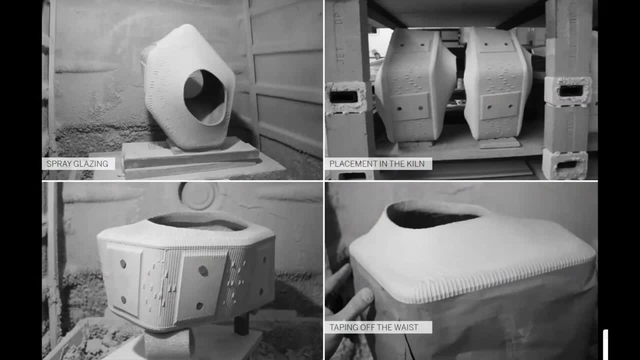 Some of the fabrication photos. Important to mention that one side of the module was made flat for the purposes that the module could stay in a can and can. Andy did make a special pedestal to prevent the glaze dripping onto the shelves and to increase the stability of the unit in its standing position. 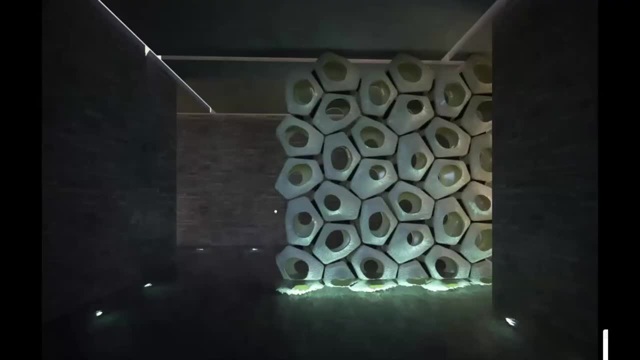 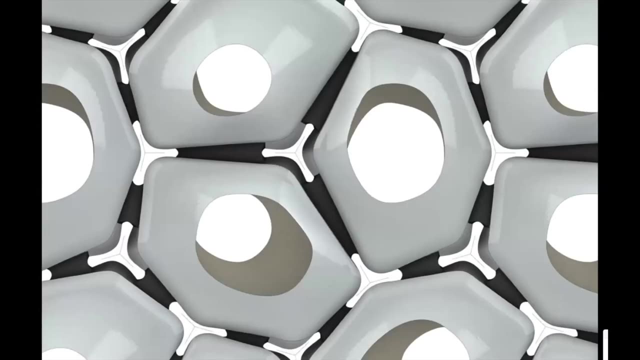 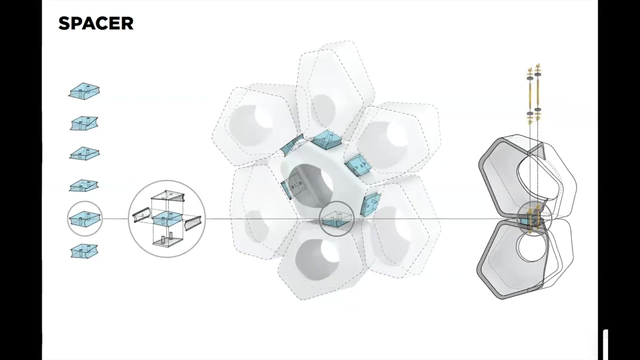 And this is just some Moody, inspirational image- how the glaze in our modules could look beautifully in a dim, light water environment. And another important component of the whole process was fabrication of the spacer. So the aggregation is essentially modules come together with the spacers between them. 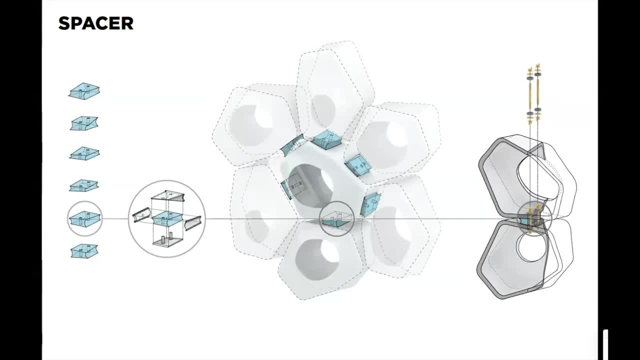 and then there is hardware that goes through. The spacers were selected to make out of rubber, silicone material for its flexibility and also so there is some play when there is a modification of the shape of the modules occurring in the kiln, so that we have some flexibility of the spacers to adjust to that. 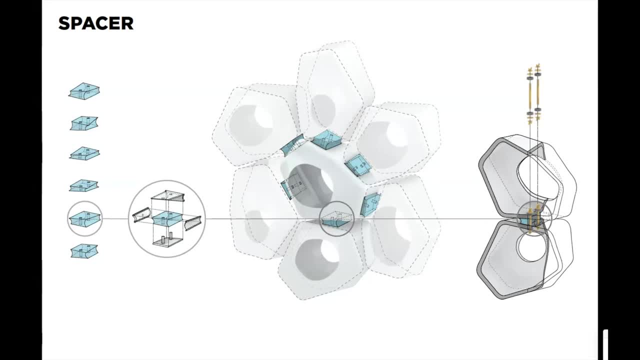 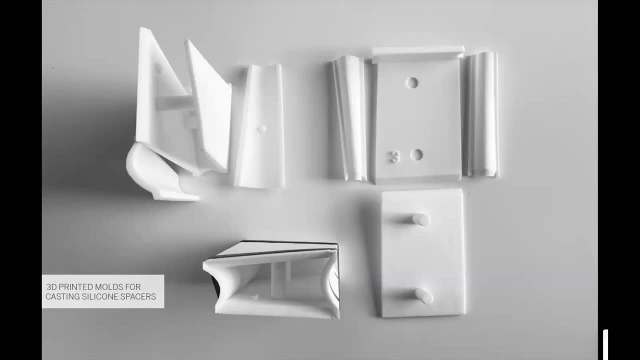 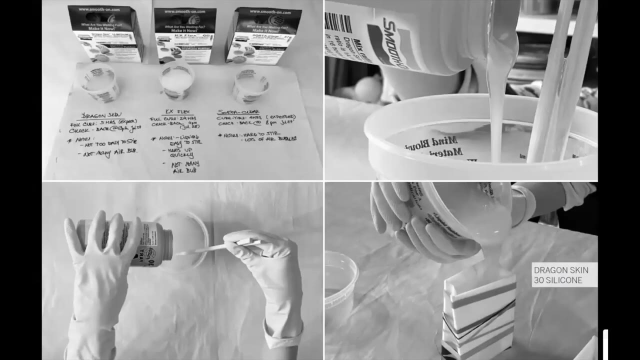 So each module has six sides. there's six sort of phoenix shape spacers. We did cast, we did create a mold 3D, printed them out of the nylon variant. It's a four-part mold. We did before casting, we cast different. 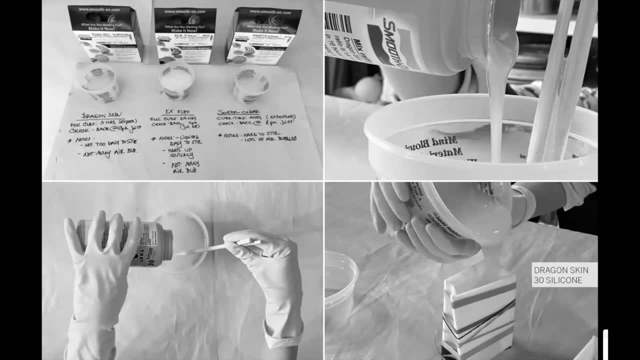 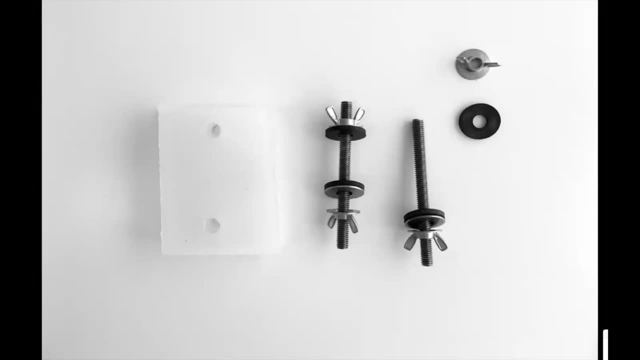 diameters of the silicones and sort of set along Dragon Skin 30,, which was rigid but at the same time soft enough. And this is, you see, a hardware which essentially three-inch steel rod with some steel washers and rubber washers. We did meet at the park once we got the three modules from. 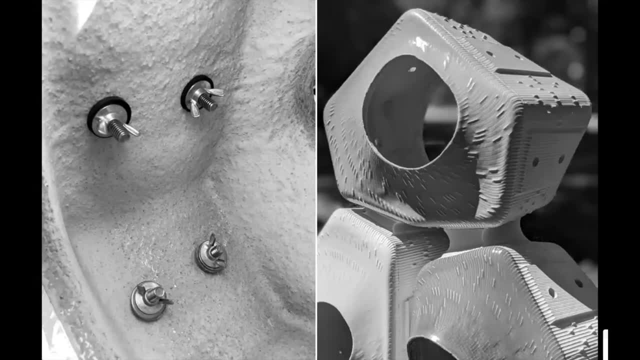 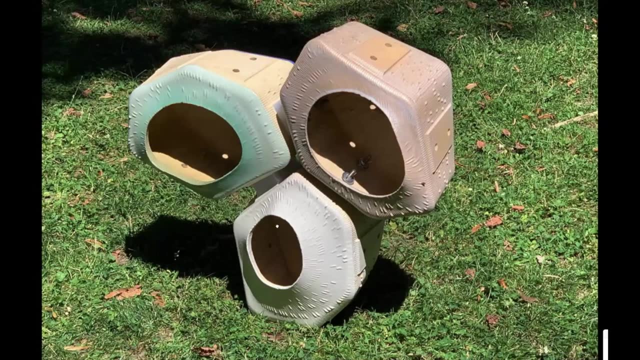 Indy, which we were super excited of, met at the park and then made the assembly and it worked. Some modules were held together sort of tightly. Let's see some photos, And then this: what you see in this picture is a. 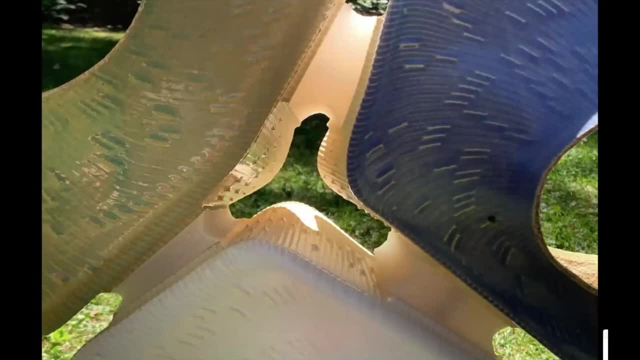 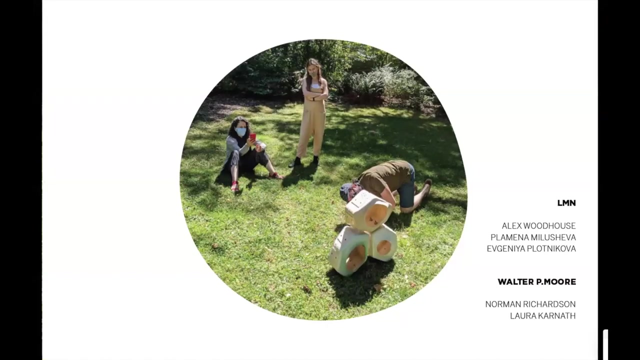 negative space, which is really artifact of the process. We didn't digitally model it, It just kind of happened And then it enhanced the overall sort of assembly and how the light comes through. There it is, And here's the team. Big shout out to our collaborators. so, Walter P Moore. 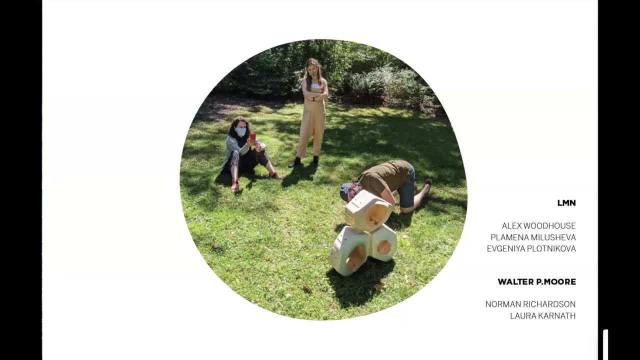 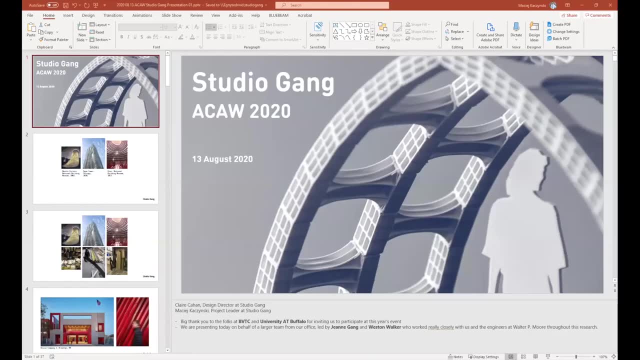 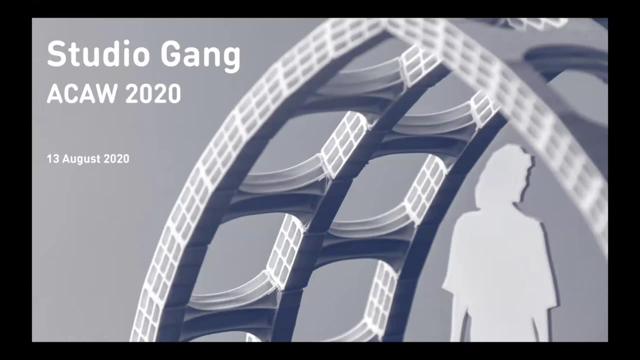 Boston Valley, Andy Braidman and the rest. Thank you. This is the end of the element presentation. Thank you, Greetings everyone. Good afternoon. I'm Macha Kaczynski from Studio Gang. I'm a project leader over here. 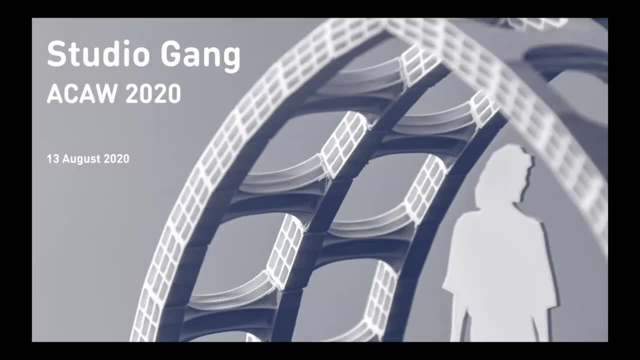 I'm going to hand it over to Claire, who's going to do the intro. Hi everybody, My name is Claire Cahan. I'm a design director here at Studio Gang. We just want to start by saying big thanks to Boston Valley, Terracotta and the University at Buffalo for inviting us to participate this year. 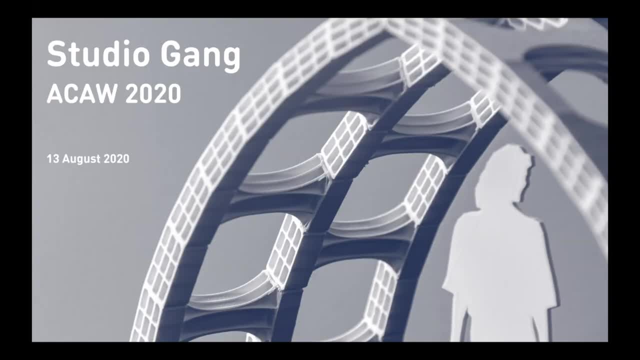 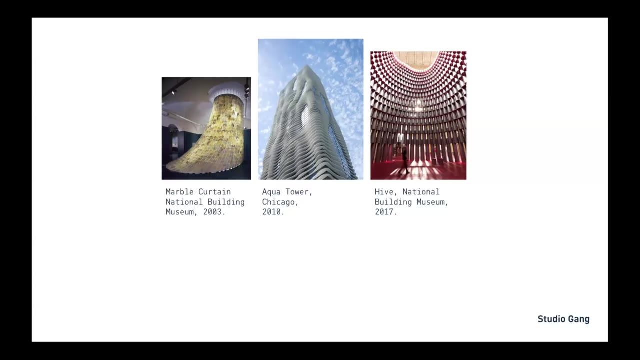 Macha and I are presenting on behalf of a larger team. here at our office We're led by Jeannie Gang and Weston Walker, who worked closely with us, and the engineers at Walter P Moore throughout the project. To begin at Studio Gang, we work on architecture and design projects at many different scales. Regardless of the scale or project type, one thing that our projects have in common is a process of material research and exploration. 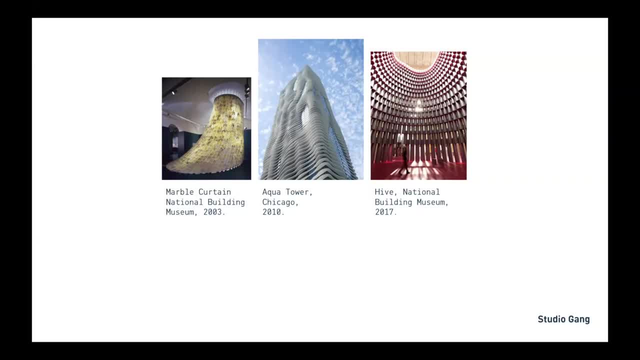 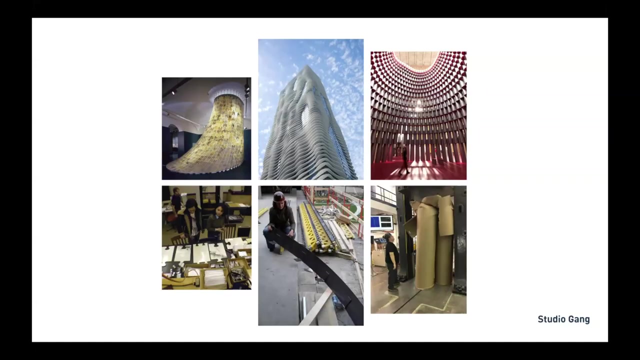 This includes both new and emerging projects. We're really interested in understanding what things are made of, how material works, how it breaks, how it performs environmentally and the cultural and historical meaning that materials carry with them. Our research and design process is iterative and hands-on. There's a lot of making and testing that happens behind the scenes, but it's always our hope that we can do it right. 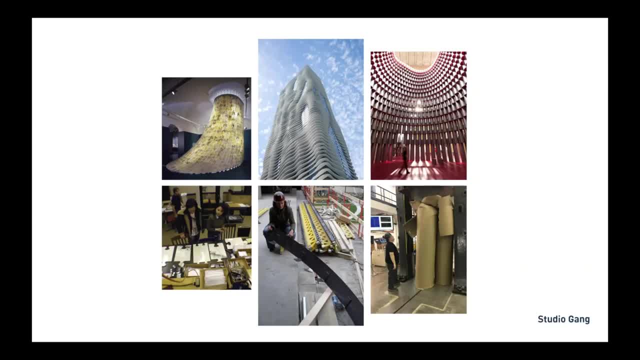 Our work is expressive of the materials we use. Projects like ACA are great opportunities to advance this research and to build the relationships with the experts. That includes material experts, but also the artists, craftspeople, community members and engineers who work with materials along with us. 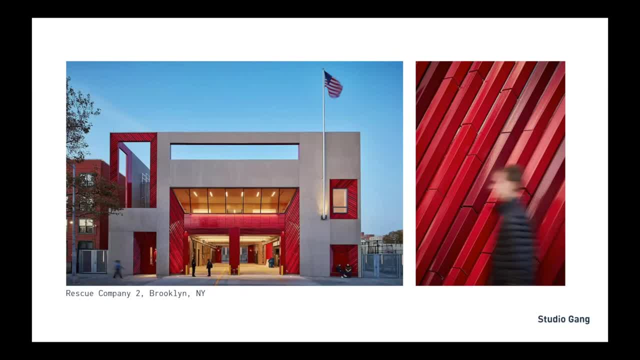 We really enjoyed working with Boston Valley Terracotta on this project. This is Rescue Company 2,, a training facility for FDNY, which recently opened in the Brownsville neighborhood in Brooklyn. The windows and openings are articulated with red glazed terracotta. This is a public building, so durability was a primary. 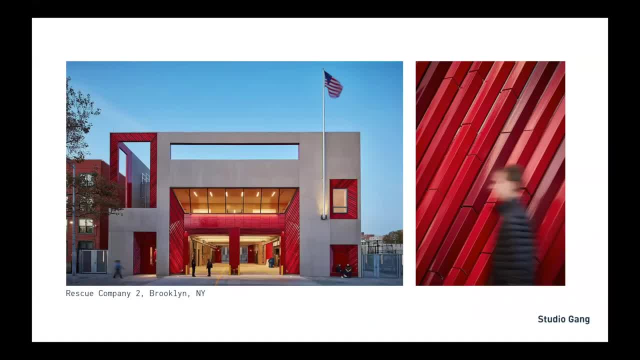 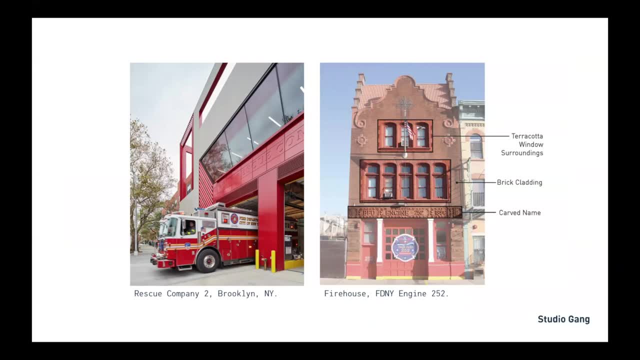 consideration. but the red terracotta was also a reference to historic firehouses. Historic firehouses in New York often have this vibrant red terracotta framing the openings, and while we really enjoyed working with this material in this way, we were astounded by the complexity and sophistication of the clips and 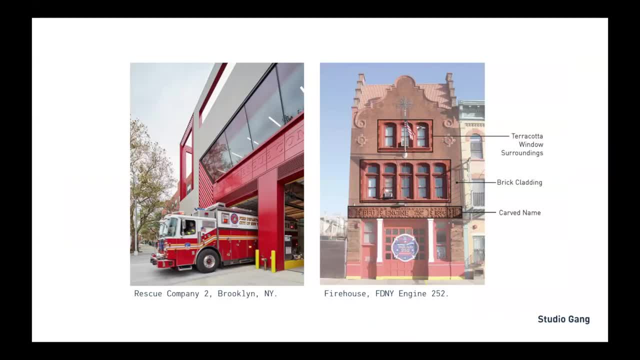 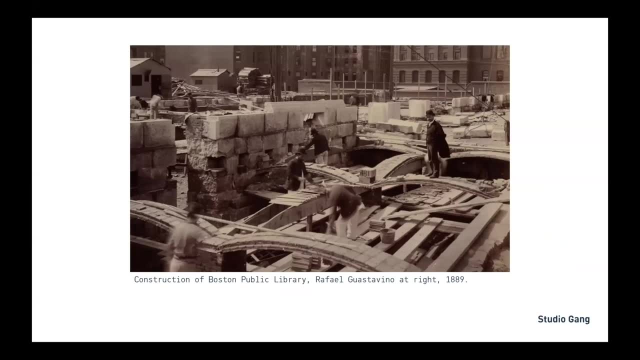 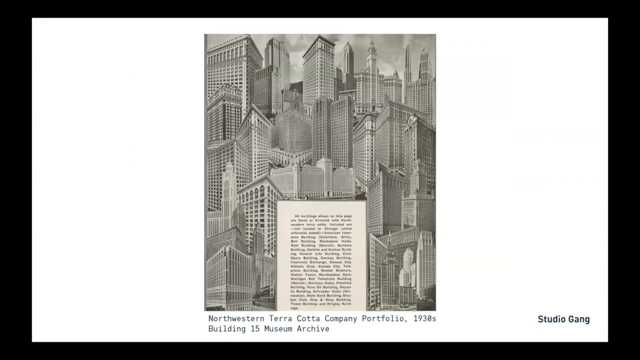 infrastructure hidden behind the facade which was necessary to hold up the terracotta pieces. Through our research, we know that terracotta is a popular facade material and this isn't new. During terracotta's golden age, it was used a lot, especially here in Chicago, on civic buildings. 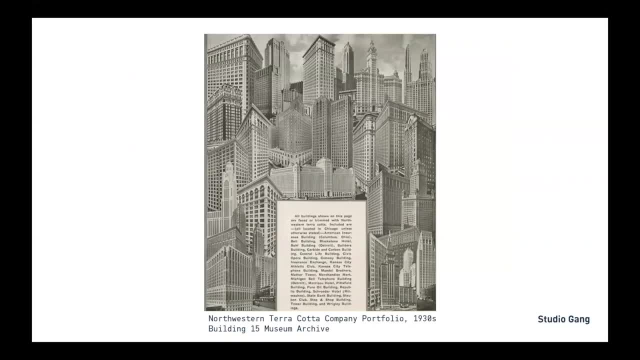 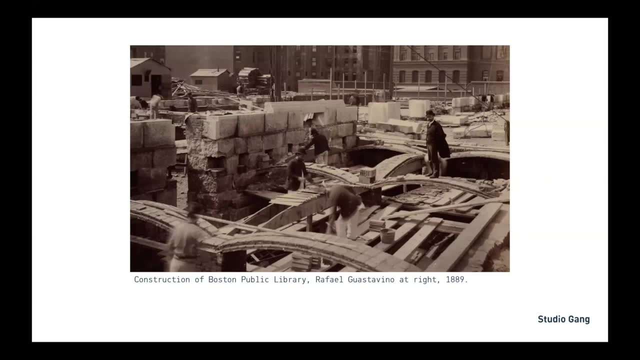 for ornamentation and then if you go back to the Guastavino matche. But ACA presented us with the opportunity to get to know terracotta beyond its facade application and really dig into the history. Not only can terracotta do more, we found, but it can do more things simultaneously. 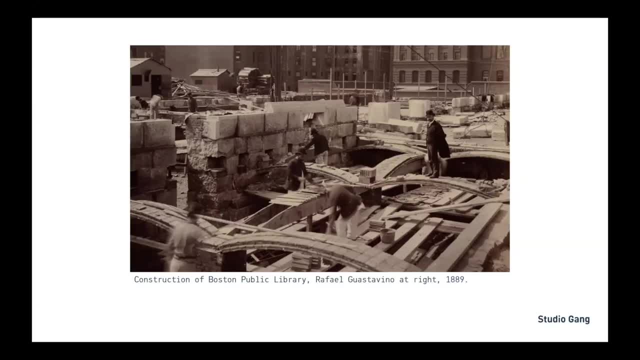 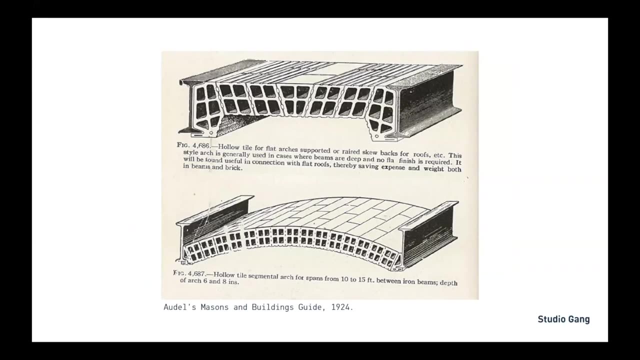 It can be a structure, fireproofing and of course, ornamentation as well. and you see that here in Guastavino's self-supporting interlocking terracotta with a very strong impression. arch- Next research slide. We were particularly interested to find these past examples of terracotta being. 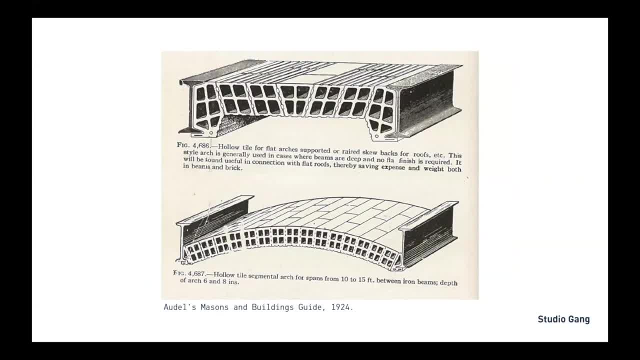 used structurally with minimal assistance and infrastructure. Here we see terracotta tiles forming an arch, literally able to hold up a floor slab, and perhaps we're taking a leap here. but we wonder: could this have become a forgotten application due to its tight tolerances? In this case, the two parallel steel beams had to be. 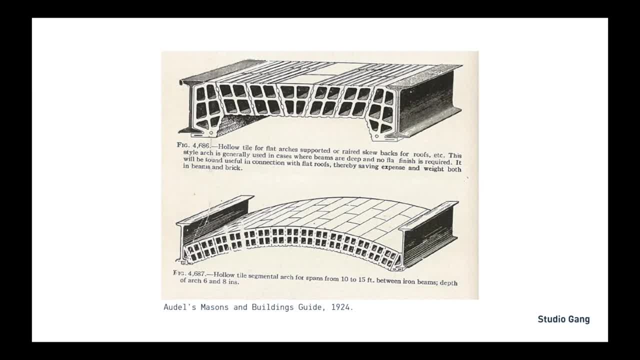 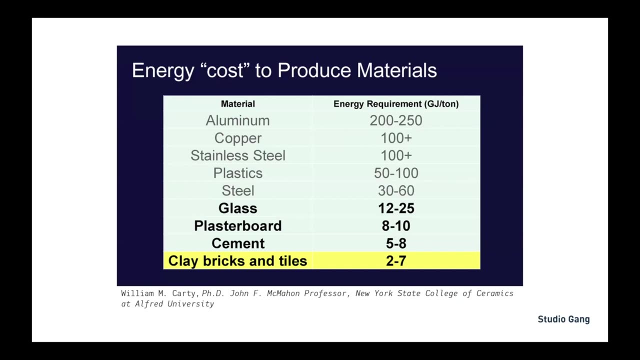 replaced to carry these tiles. and since we have new technology today, we wonder if there could be a new home for this old technique, And in our project we paired that with research by Dr Carty which was really great to have access to. We think this is. 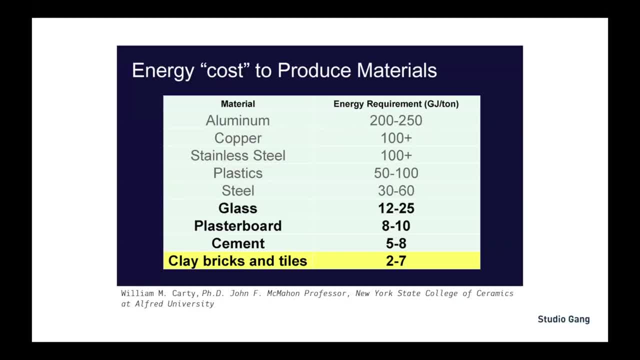 the right time to revive this material and acknowledge the necessity to maximize the environmental benefit, reduce waste and reduce the carbon footprint in the building. So we're really excited to see what we can do, and we're excited to see what we can do to make sure that this is being created by the building industry today. 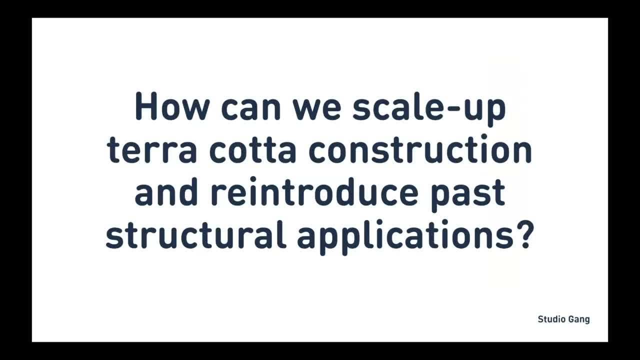 So with that, I'm going to turn it over to Maciej. Thanks, Claire. thanks for the setup. So I think in some way this is probably the most fundamental question of our research: How can we scale up? we'll return to that word in a. 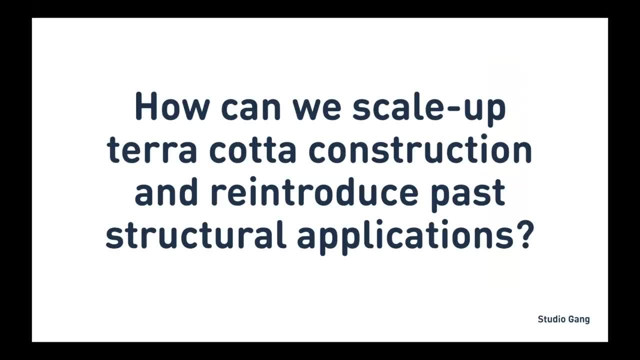 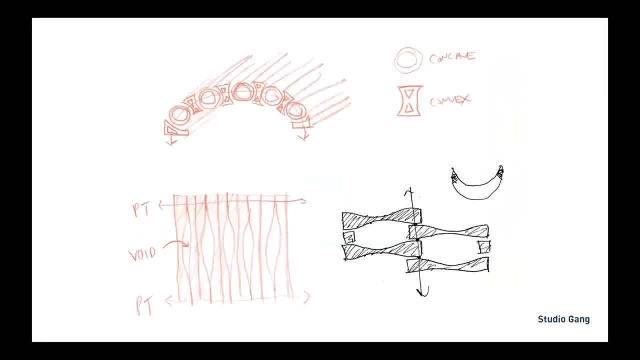 second, how can we scale up terracotta construction and perhaps, in so doing, reintroduce some of these past structural applications? So by scale up, I think I mean more specifically moving the whole building around the building. So we're going to start with the 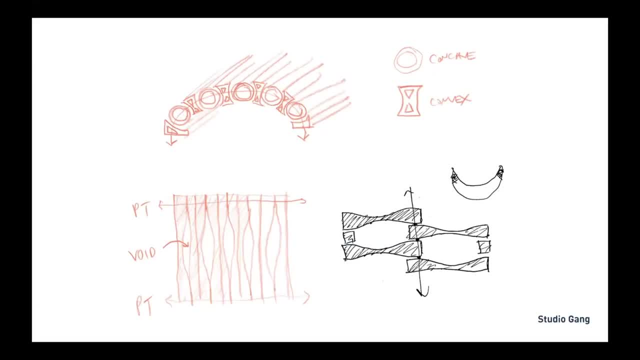 construction of the building. So I think this is a very early sketch of a translation from that initial research into design and this actually nicely summarizes, I think, a lot of the key ingredients that did follow us through the entire design process. So some things, some key ingredients you do see here. 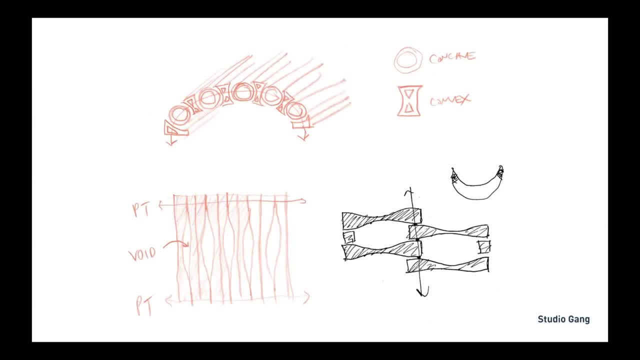 this is an extrusion. we were inspired by those initial images of the historic images that use that technology. Part A and Part B were necessary. we wanted to have two parts doing this assembly at least, perhaps one actually also As some kind of means to produce a singular or monolithic 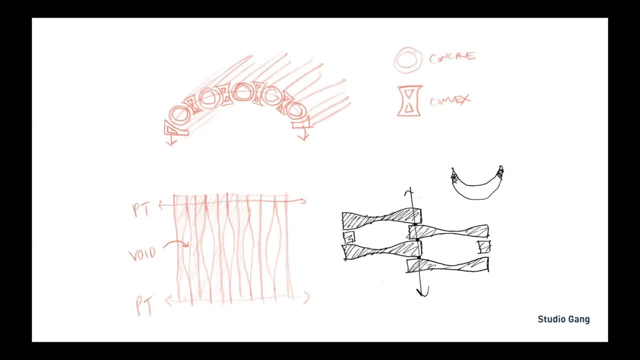 mega panel, if you will. There's this idea about assembling on the ground, whether that's in some kind of form, work, and then leaning up or lifting up to another, to another place and, perhaps working with this tensioning, finding places. are there other places where we could do removals of the material to actually 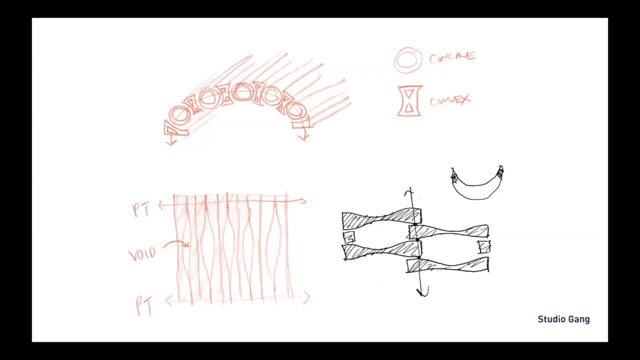 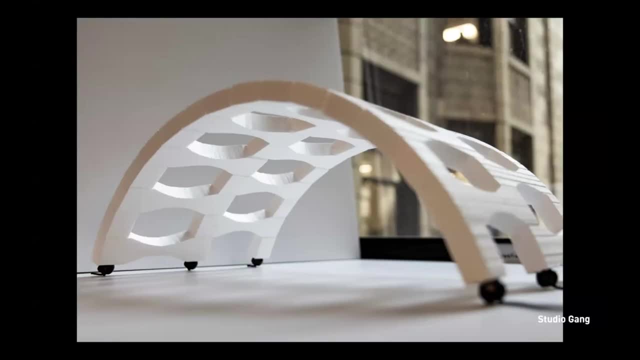 provide some some, some characters and some texture. Here's a quick conceptual model that we used to test the tensioning process, so this is literally holding itself up with tensioning. it's just a phone model. We did try a variety of configurations but really felt that a compressive. 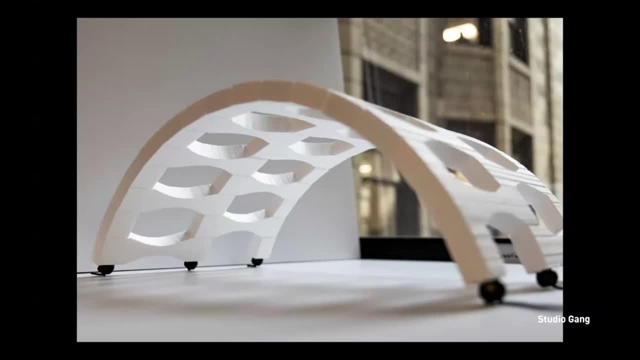 structure was the most honest and candid exploration of the material, and this, interestingly, in the semi-circular form that you see here, which, of course, is an inevitable byproduct of having a singular extrusion. we learned that this arch had a theoretical weight limit. that makes sense and according to our 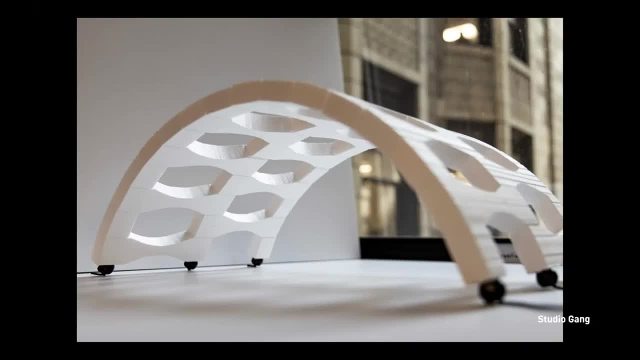 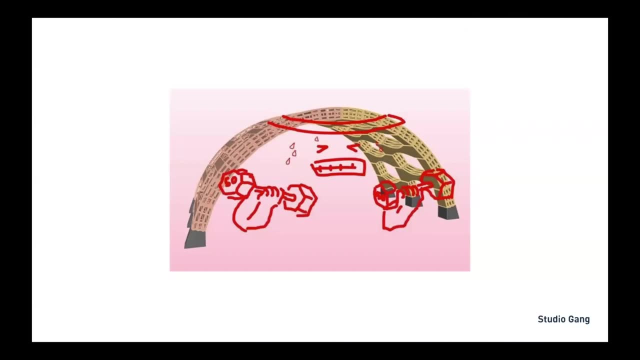 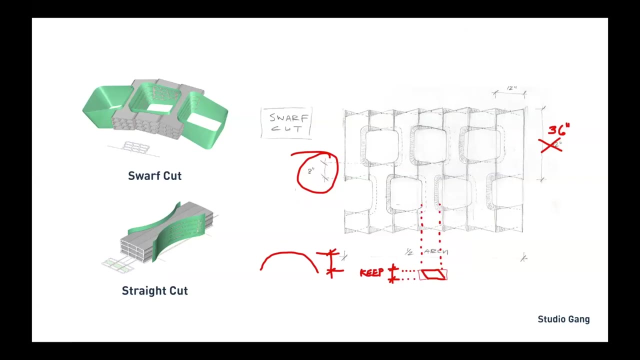 experts at Walter P Moore, we had exceeded that. so it was very clear to us. they told us clearly and tactfully that Archie had to lose some weight. so to that end we embraced wire cutting. so this was came a little bit later as a secondary operation. we had ideas about 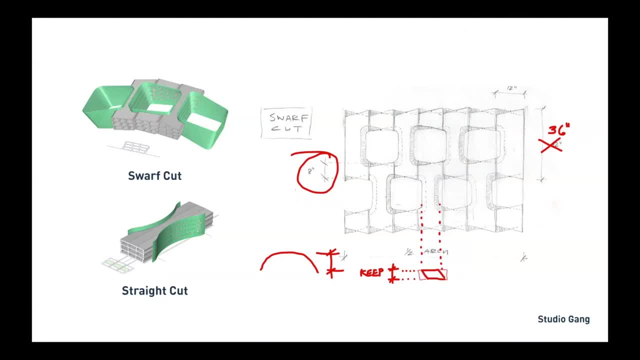 voids in the first place. but this of course, was to remove some of that material and, importantly, to to find- this is- this was kind of a found step- but to find lightness within a heavy material. so of course we work closely with Matter Factory in Boston Valley, Terracotta, to 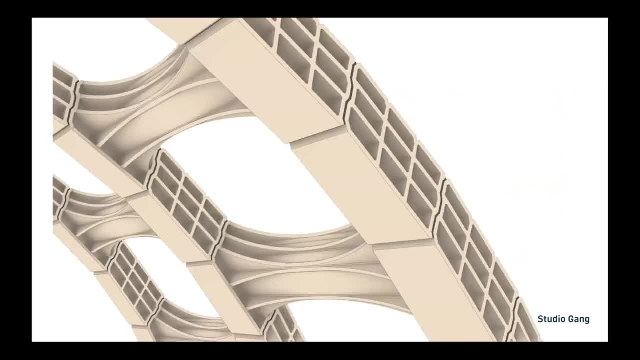 learn the rules of, and constraints of, wire cutting. Here's a quick close-up of some of those cutouts that we ended up using in our final piece, and again, our goal was to remove as much as possible. the cutoff of cutoffs, of course, go back into the, into the. 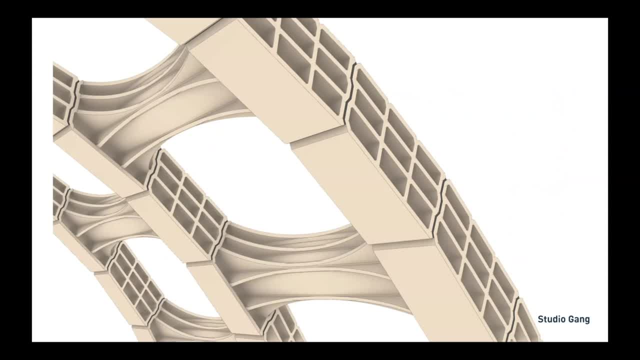 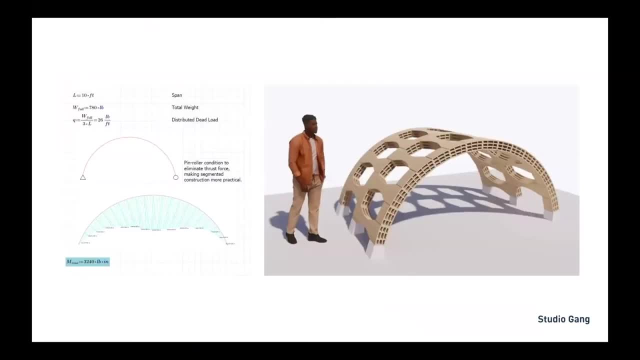 stream of the extruder and, of course, we did as much as we could without actually structurally compromising Archie, which was, of course, the name of our beloved arch. so, despite our best efforts to put Archie on a diet, we found that the largest available span to us was 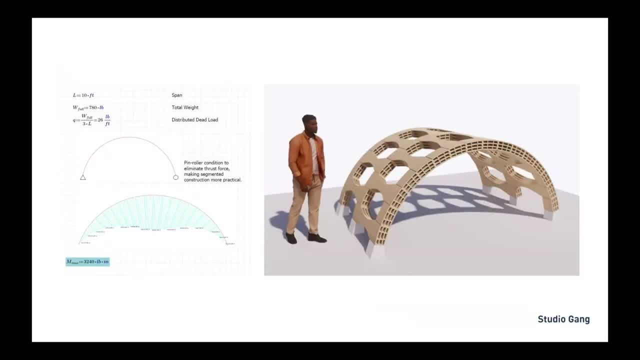 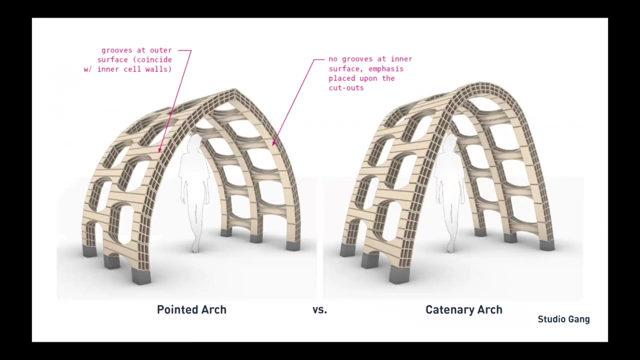 was still kind of at an odd and unoccupiable scale. so of course, for the purposes of the exhibition and also because we are architects and we just can't help but think this way, we wanted to find a way, of course, to make Archie occupiable. so we kind of scratched our heads and we 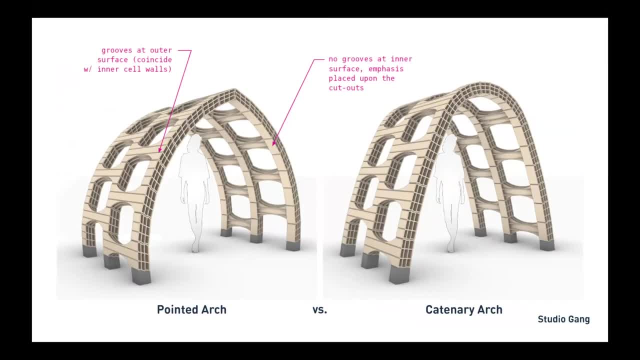 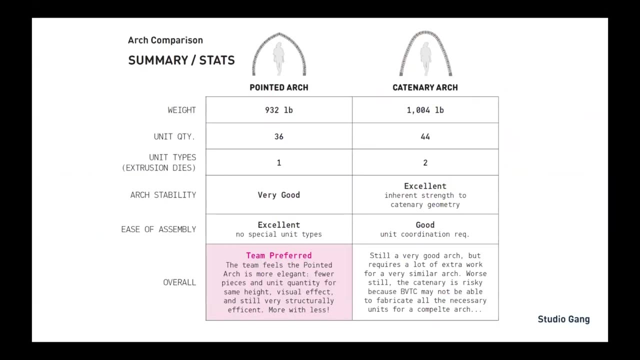 looked at our heads and I remember somebody saying what if we did a pointed arch? so that was immediately like very provocative. we of course had to compare that to a catenary arch, again achieving a comfortable, clear height beneath. we're very big fans of studio gang of taking. 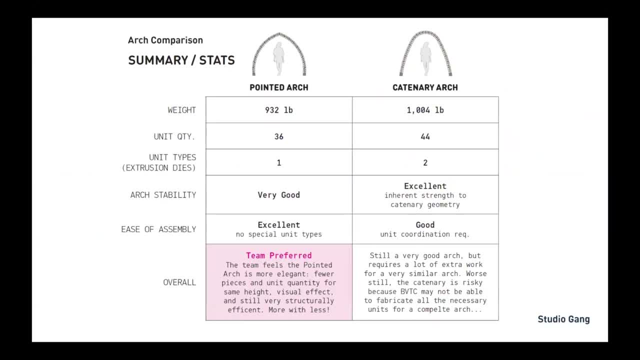 complicated facts or concepts or statistics and trying to present those in really clear fashions. and after sort of doing that with these two options, it became really clear to us that the pointed arch was definitely the winner. Again, it had fewer pieces, it had fewer unit types. 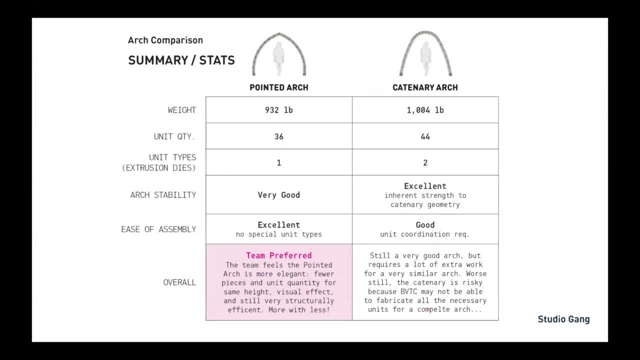 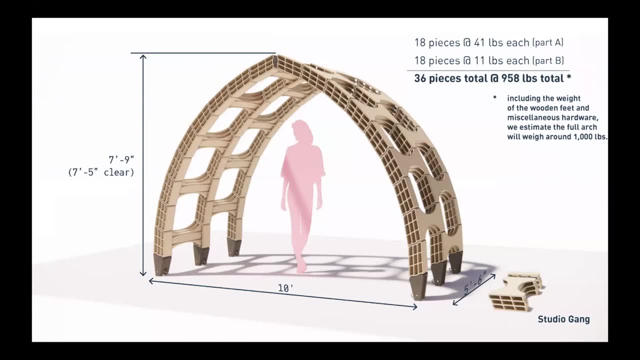 and also gave us the desired height and structural effect. Some quick stats for the final arch design. we've got 36 total terracotta pieces here, 18 of A the large, 18 of B the small, about a thousand pounds total. We do have neoprene gaskets between all the 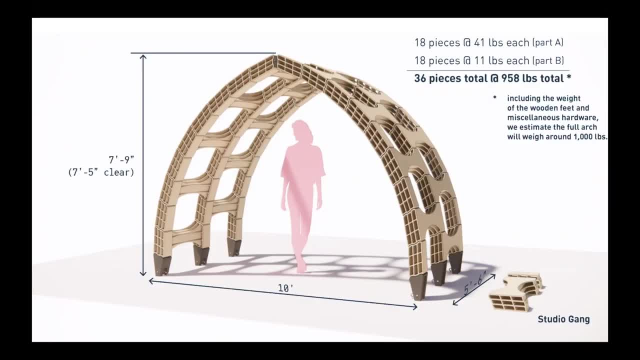 terracotta pieces. there are, of course, wooden. I'm not sure if you can see my cursor, but of course there are wooden feet and and a keystone. What you don't see here is the. actually, what you can barely see here is the, the dyneema rope which is doing the tensioning from the steel pins at the. 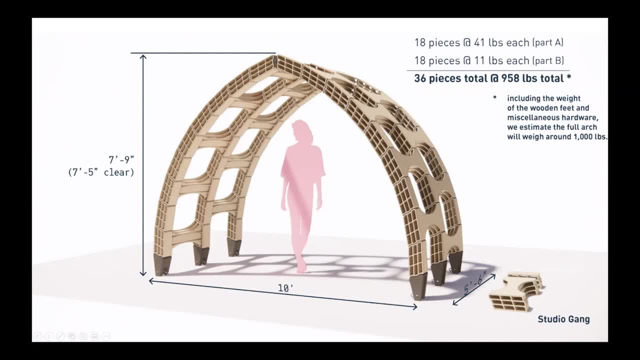 keystone down to the steel pins in the feet. so there is an important ingredient here that that isn't visible but is doing quite a bit of work. Also worth mentioning: the buildability was also very important to us. we wanted to make sure that even the larger piece was something that could be. 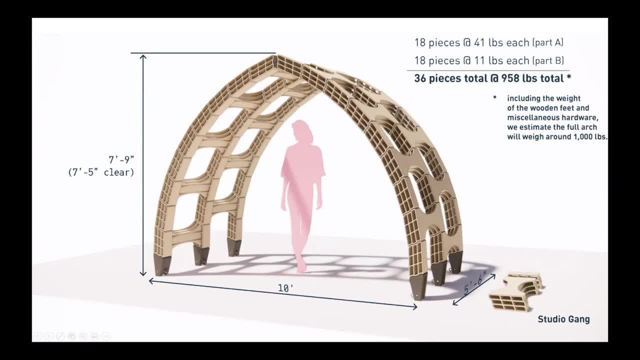 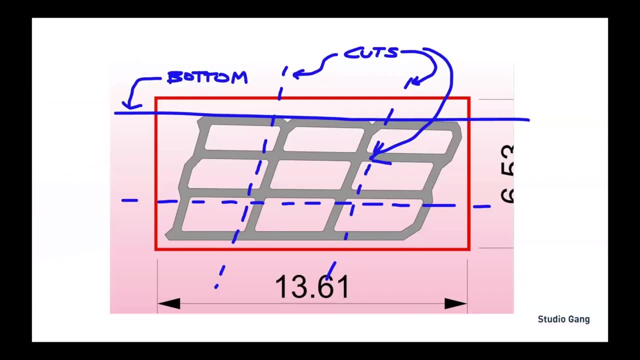 handled. so I think we were at 41 pounds. I'm not even sure if I can lift that, but I assume um two people lift that. um, it's also um. it's worth acknowledging that in pre-COVID times we had been working, of course, virtually uh, both internally. 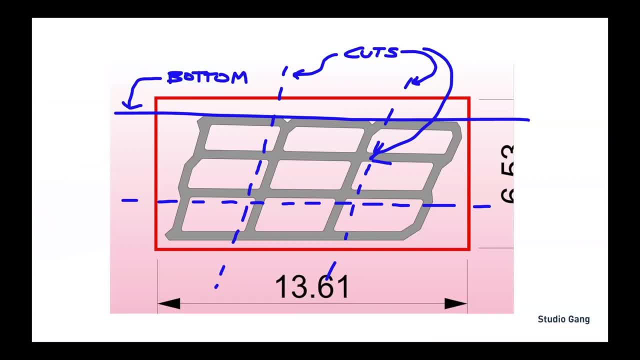 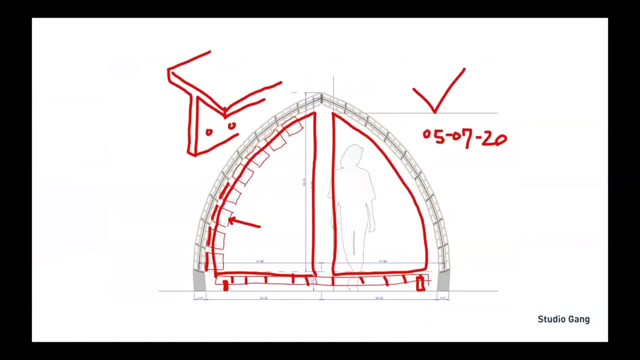 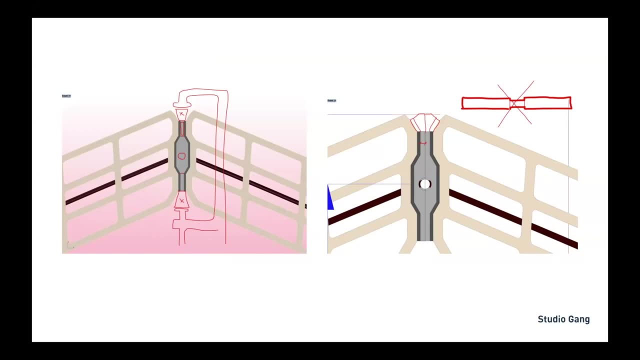 and across uh with Lawson Valley, terracotta and matter factory and Walter P Moore. but live sketching of course became a very necessary and fluid tool, of course, to collaboratively explore, exchange and even record ideas. very literally, you're looking at the sampling of our meeting minutes, as we came to call them. 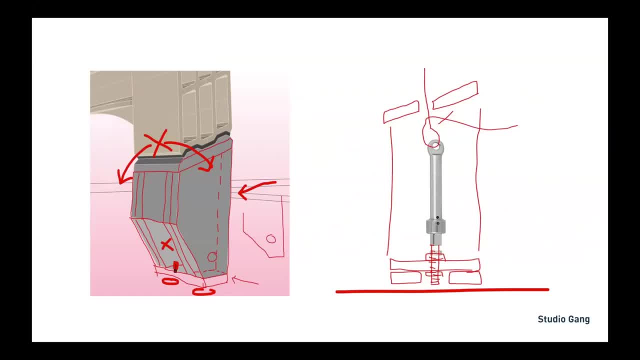 uh, here's some quick sketches and looking at some explorations into the- uh, the feet, and we were exploring how to house some of that tensioning hardware. uh, what you see on the right there, actually we ended up not going in that direction. and again, um, explorations and how to bring. 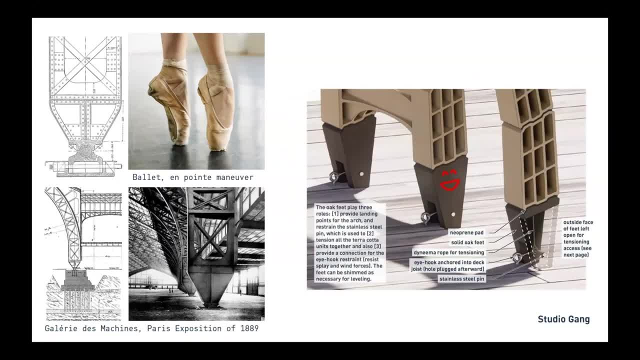 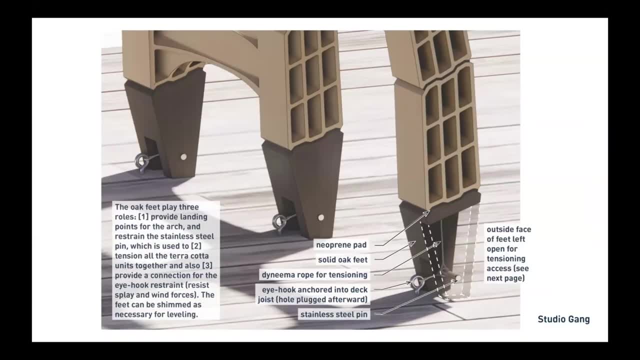 levity and lightness into the seemingly heavy material. uh, it should be very clear also that the intent of this presentation is absolutely not to dive into some of the technical side of the arch. uh, we think that, um, this is really intended to give you. this slide here is intended to give you a. 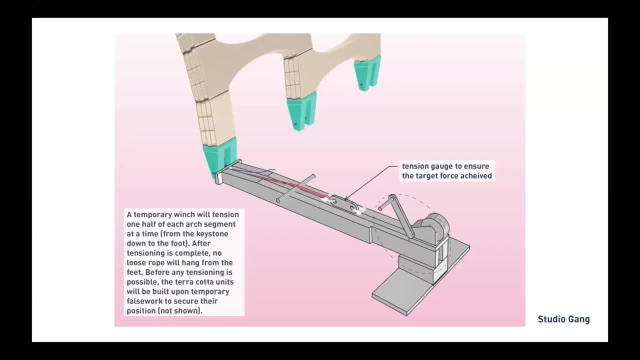 technical flavor of the of the feet, um, and also the tensioning, in this case the tensioning apparatus, uh, which we designed to to tightly and snugly bring Archie's posture um into uh. it's a beautiful form um. note that we don't show in this image any kind of temporary false work. that is certainly a part of. 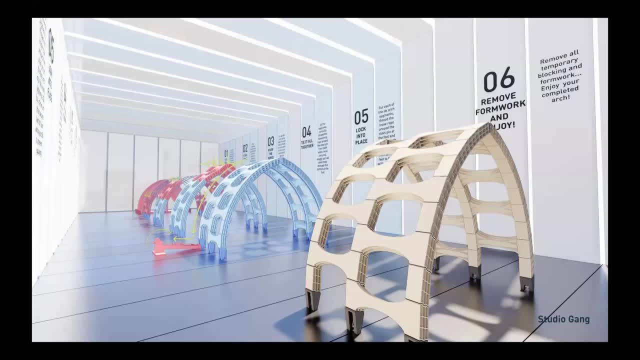 this of how to stand Archie up, but if you would like to learn more about all the steps necessary to build an arch, please be sure to check out the virtual exhibition- everyone's received that link at this point, uh- where we diagrammatically illustrate the full sequence of events to build an arch and 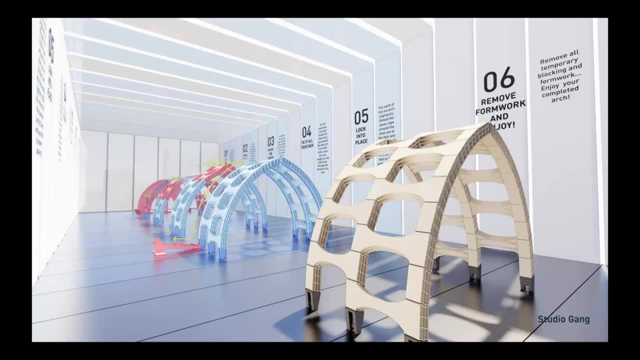 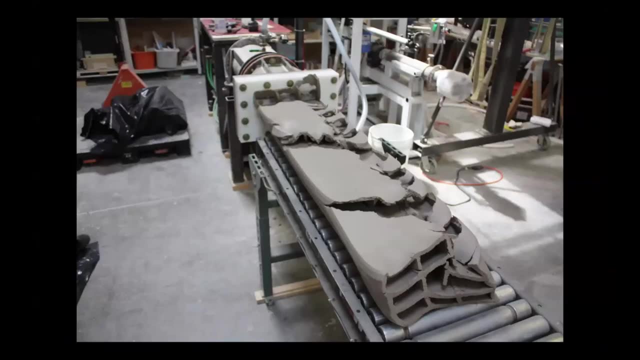 as you can see, there are exactly six steps to do so. uh, you'll find in this presentation that there is actually not a single image of an actual arch, so here's a behind the scenes peek at our progress. this is one of the many extruder trials that took place at 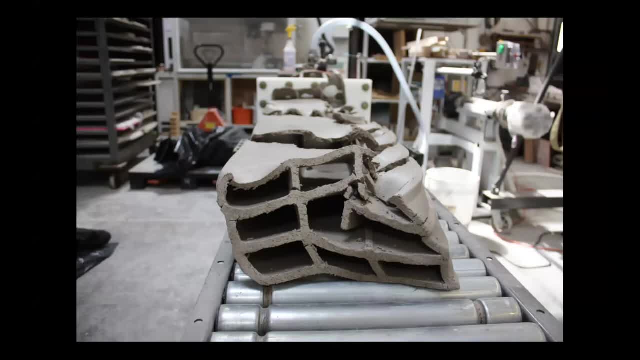 matter factory. so, uh, well, i'm not sure if you can see this- while we here at studio gang weren't able to get our hands dirty on, uh, we were actually really excited. i mean this entirely. we were really excited and thankful to learn more about the extrusion process. 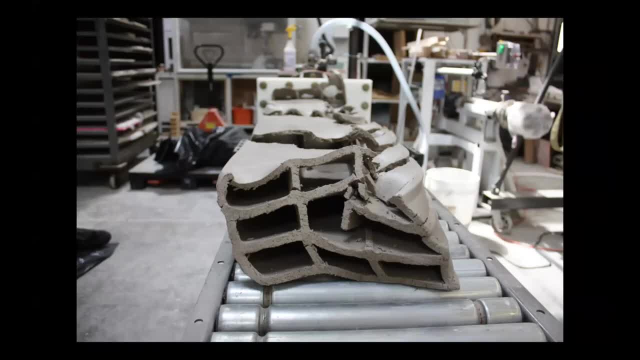 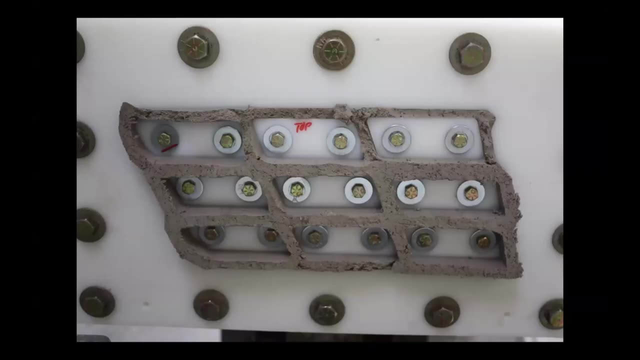 uh, through these failures, through, uh, through matter factory, and i, i again mean this entirely and earnestly- that, uh, we are profound believers in the learning that happens through through failures, particularly with material accelerations. so i won't do this explanation justice, but let me try, uh, so it turns out that the extents of the 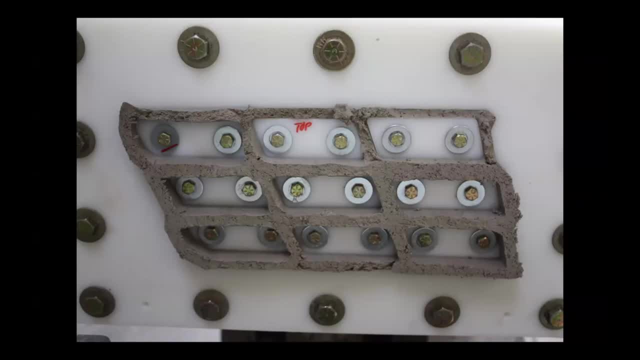 profile were a little bit too close to the limits of the extruder. beyond, which changes the. this is fascinating, uh, very fascinating. which changes the flow and the memory of the moving clay. actually, as it's being pushed through the dye, the clay produces eddies and its own currents, kind of like rocks in a. 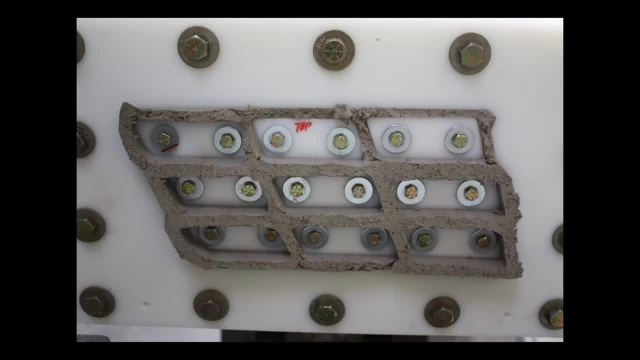 turbulent river so it builds a, a bias or a skew into the extrusion. uh, if you look casually at an extruder it appears conceptually obvious: right like clay plus pressure, plus dye equals extrusion. but really we should all, i think, acknowledge the extraordinary craft and care that goes. 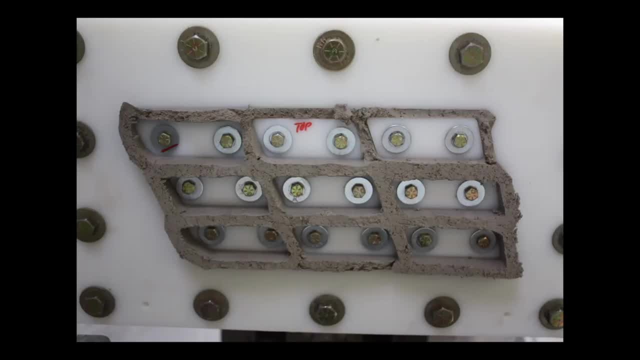 into every success that we see. so big, big thank you to andy raymond and the matter factory folks who made the valiant effort to get all these pieces to run and took the time to very carefully explain all the hiccups that they were finding. 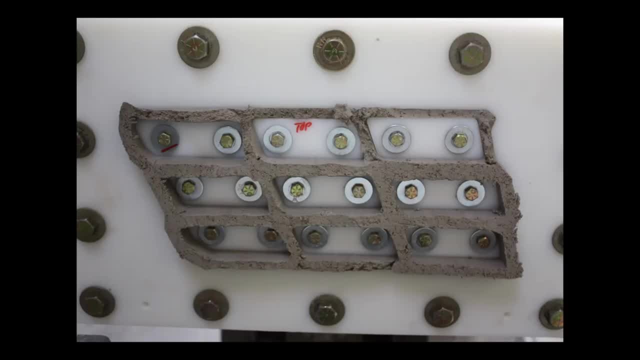 and also big, big thank you to john kraus and the experts over at boston valley, terracotta for offering to take over this extrusion. i can't tell you how excited we are to get these pieces in our hands and i'm very excited to be able to share them with you guys and to um, to give archie a. 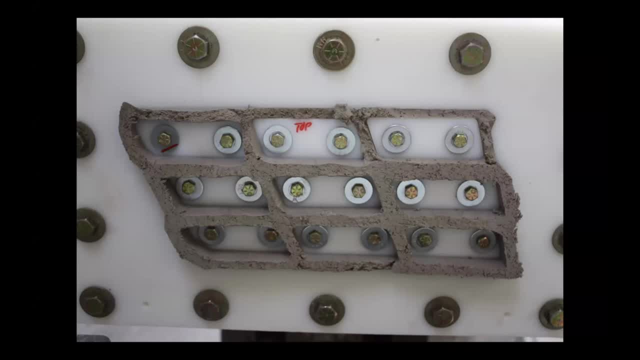 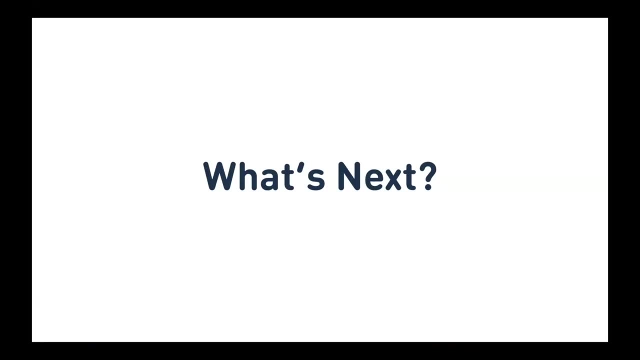 home here at our chicago office. uh, please do check out our website in the coming weeks, where we'll be posting images about the construction. so what's next? a couple peeks at some of the other explanations that we are hoping to do in the future. uh, initially we had hoped to find i 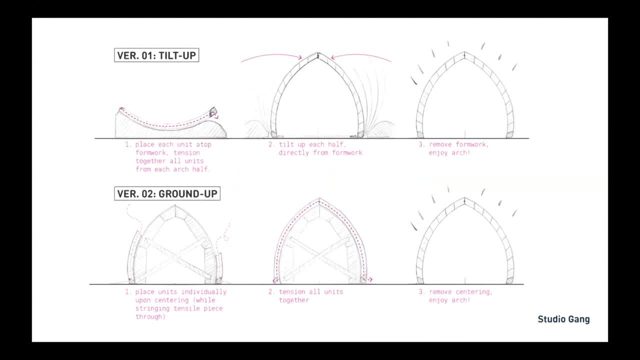 think, a greater, let's say, constructional mileage out of the tensioning procedure and in that would be in an attempt to obviate the need for a temporary false work, which can be of course itself uh, quite, quite a lot, but i think that's a good point. um, but we ultimately found for our case that we 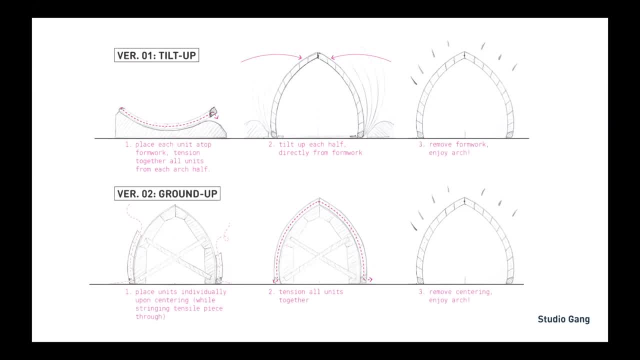 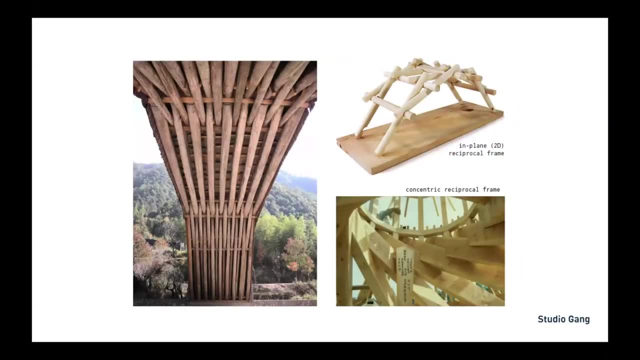 do intend to use a conventional ground-up false work, but the tilt up, uh, the build on the ground tension tilt up does seem to have a lot of potential that we haven't yet fully exploited. uh, we would also like to expand our line of research into reciprocal frame structures made of terracotta. this was 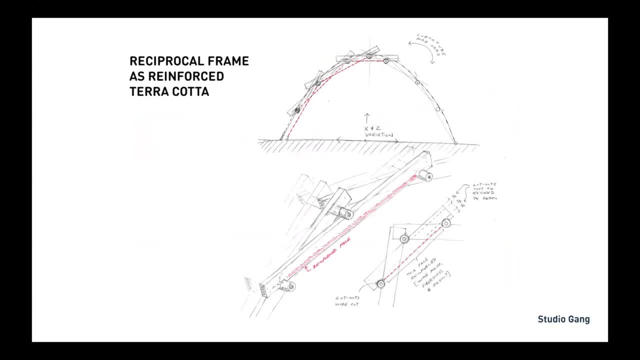 another angle of research we had entertained, which of course would require, you might say: well, machi, that's not going to stand up and need some tensile reinforcement. and i would say: well, okay, then we should integrate some kind of tensile reinforcement, uh, post extrusion, of course. and so boston valley, terracotta, uh, if we are invited, 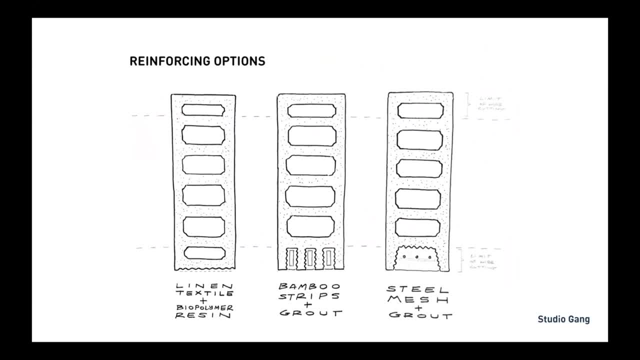 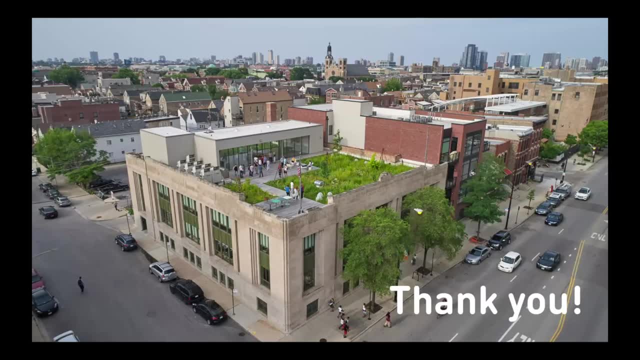 back next year. uh, we call dibs on post-extrusion tensile reinforcement research and uh, thank you very much. this will be hopefully archie's uh home in the future. home on the range, we say: uh, please do, uh, visit us. i should say that this is a semi-public space. 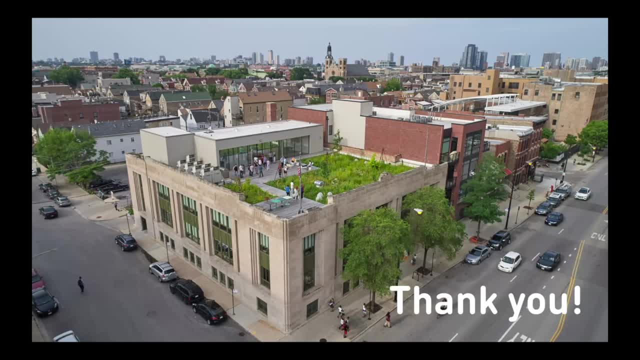 uh, where we host events, etc. so it is possible at some point in the future, when we can um all get together, that you could see archie yourself. thank you very much, great thank. thank you very much, uh. so, um, what what i'd like to do now is to just 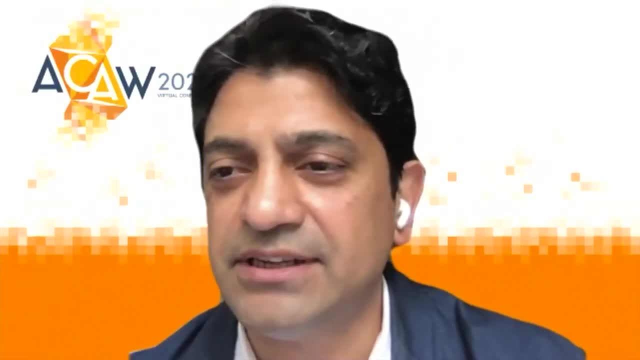 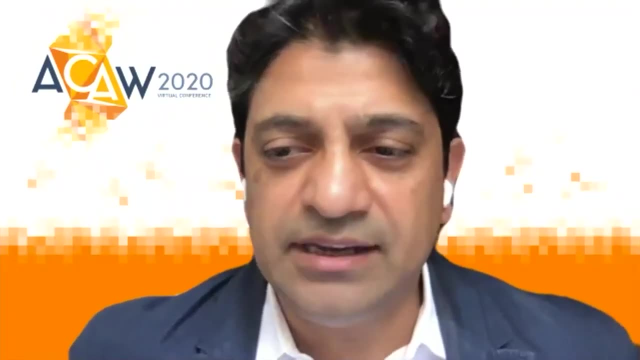 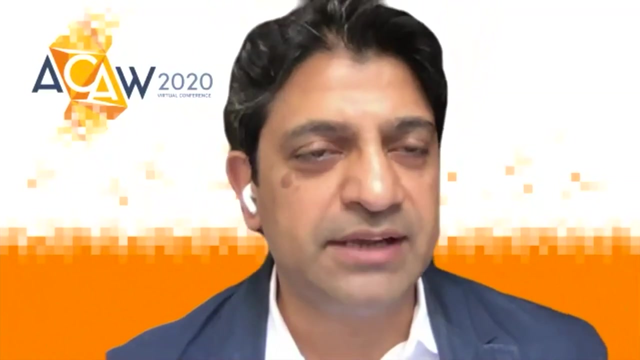 ask all the panelists to make themselves visible. i will also make them visible for the um, the attendees, and maybe we can get started. uh to the attendees: if you have questions, please do put them uh in the chat and and we can pass those on. so, first of all, thank you everyone. the the work is again uh, uh, a lot of work to 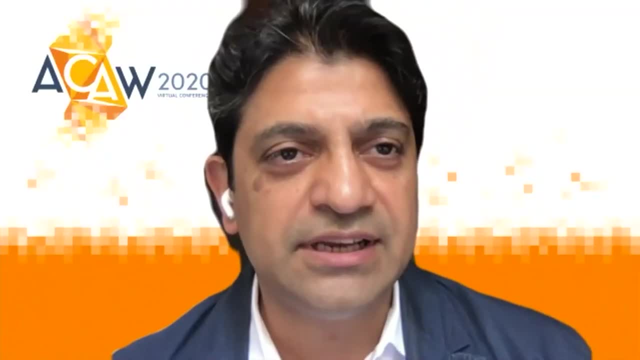 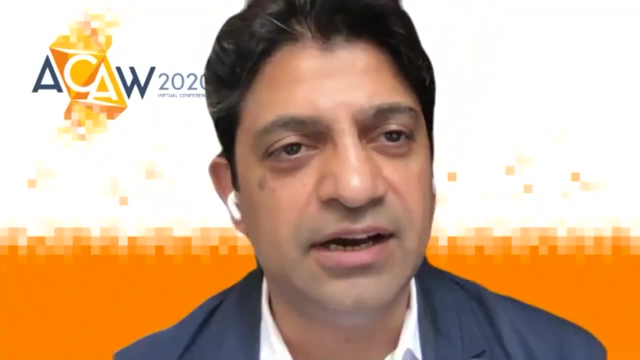 be done with, um, thoughtful, exuberant, uh, with really interesting kind of directions. i wanted to maybe shift our discussion a little bit in in a different way. uh, for for this uh uh series, because it isn't, uh, the facade that we're doing. we're doing a lot of interiors, we're 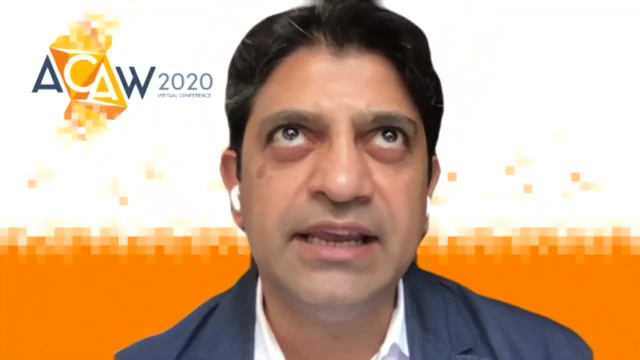 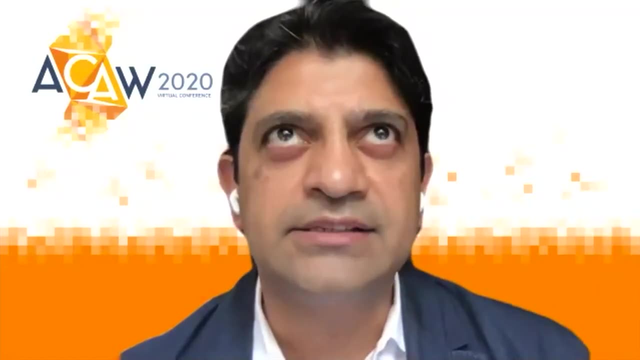 doing a lot of other other things with it. um, one of the things that in the past a cow uh came up was: you know how good is uh terracotta as a uh as a collaborator material with other materials? uh, a lot of. In other words, it works very well. 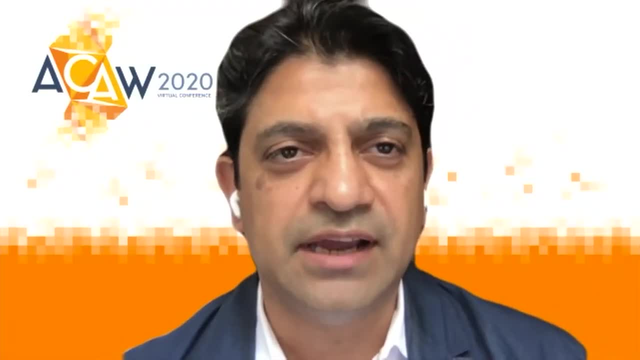 And we're sort of seeing some questions, let's say, as to how these other materials, whether it is organic material, living material that has to sort of occupy it or, for that matter, gaskets and other things, or as post-tensioning, let's say, in the last presentation. 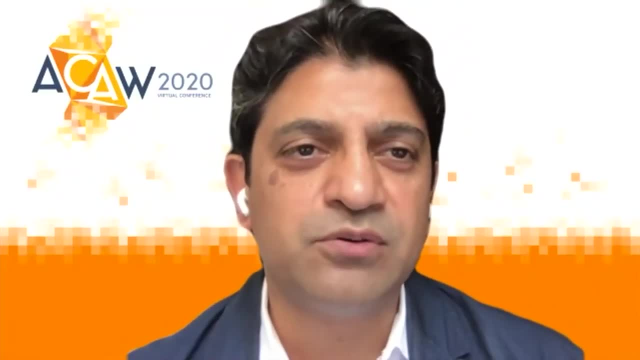 Can you speak a little bit to you know, I think there's a question of the form, but of course that is specific to, let's say, the geometry problem. I'm thinking more of the assembly problem. How is your thinking about these assemblies and how these things attach to actually architecture or become architecture themselves? 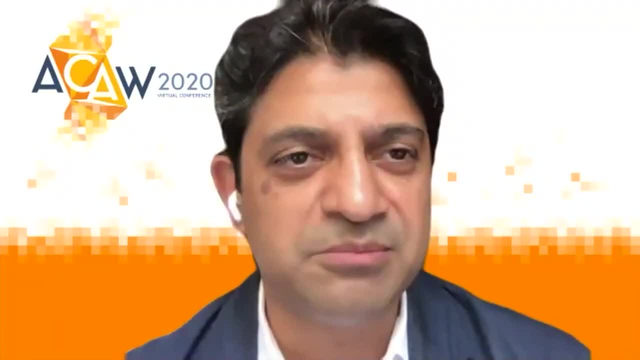 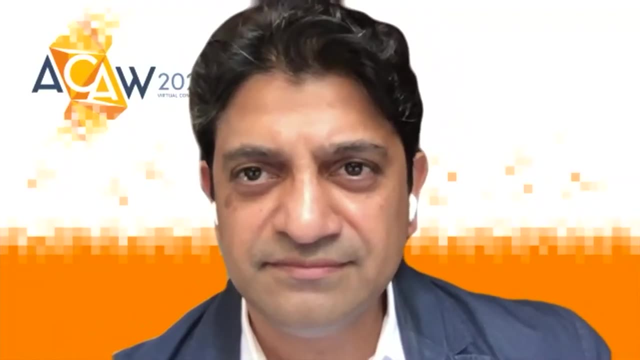 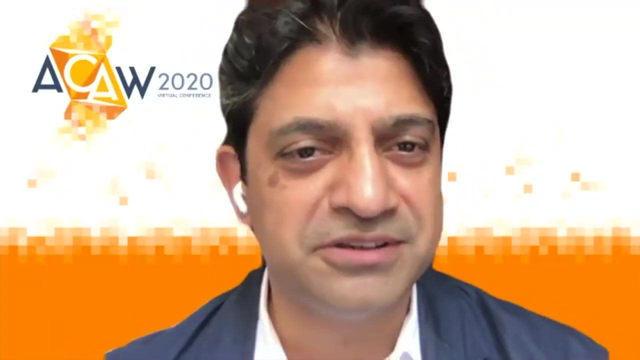 What are some of the challenges that you guys are seeing? now that you've been working with the material and the conversation you've had, Maybe the structures- people can take that on first, because I'm sure they're the ones who, Gustav, I'm imagining you probably have a lot to say on that. 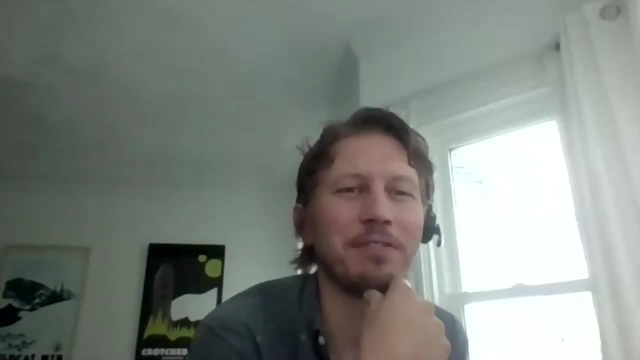 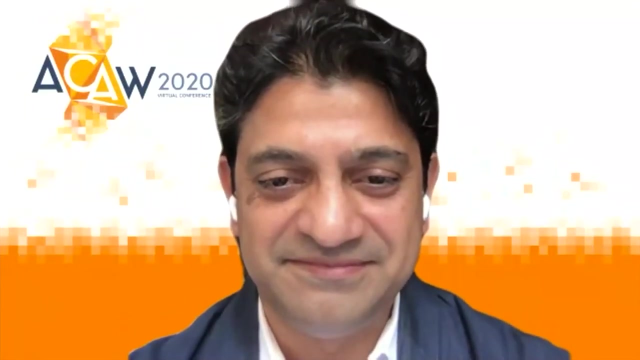 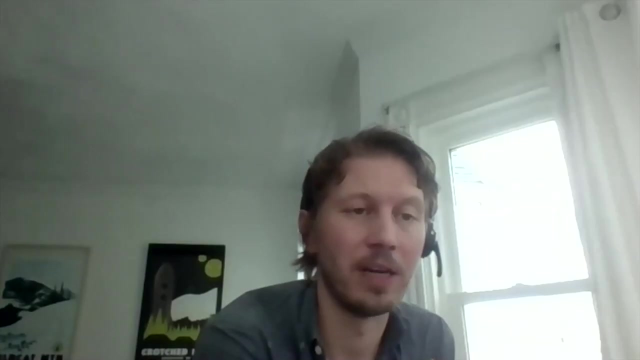 Yeah, I was waiting to see if someone else would pick that up. Yeah, so you're right, We've been involved in various kind of projects with this great event- for this is the fifth year running now actually- and have tried, you know, our hand at many, many different ways of kind of treating terracotta, both from a sort of material- more I wouldn't say molecular, because we don't quite have that ability- but like the material makeup, all the way to the assembly. 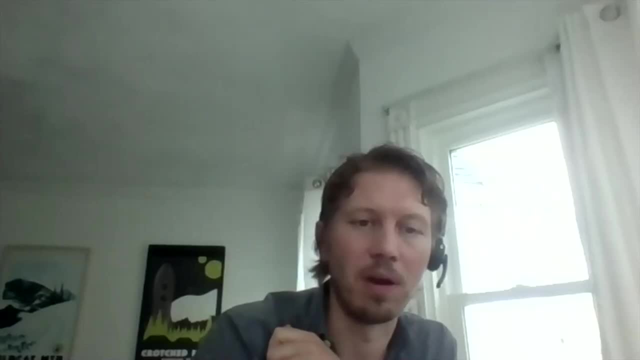 And I mean one sort of continual red thread, let's say, is always the. you know the way that terracotta traditionally wants to be treated, meaning that it's a compression material and that, with varying success, we try to induce bending and tension into it, which you know- the last project here, for instance, would be an example of that right. 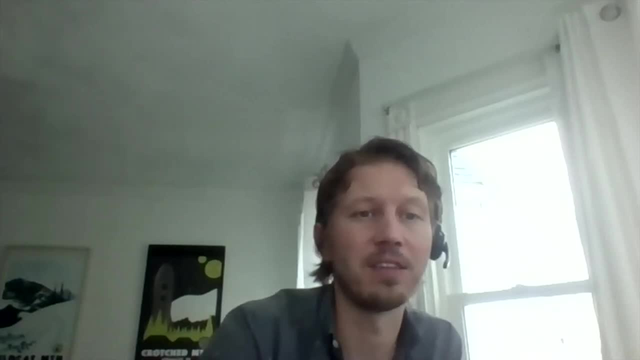 And you know, sometimes it works and sometimes it doesn't. So I think that that is that's a very interesting kind of path of exploration that is fairly little, little tried, tried, yet you know it's not so well traveled yet. just because it- I mean, I'm not going to speak for everyone, but in my own experience- maybe that says something about me- it fails mainly most often, right? 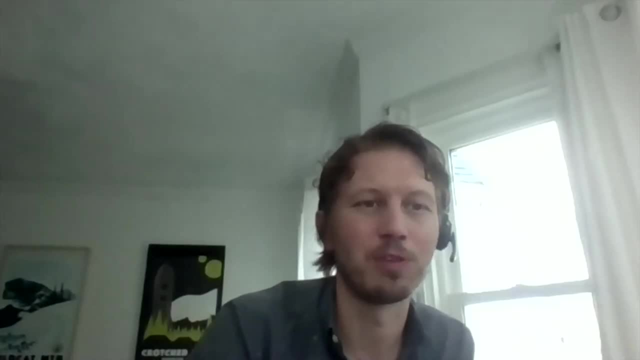 And after a while you know, yes, a failed experiment also proves something. but after a while you also sort of want to get something out of it, right? So I think, if I speak to the project that I was myself advising on this year, 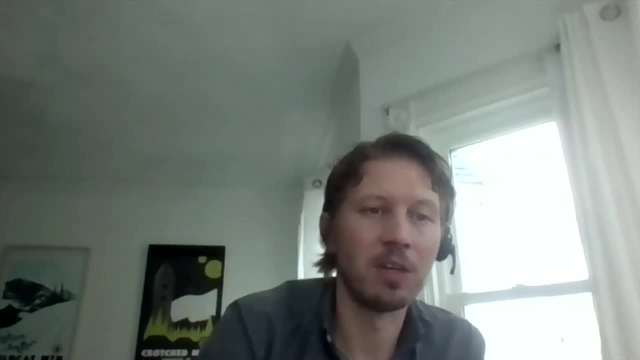 what I really love about that is that we are: we're not necessarily questioning, like you know, what the terracotta can do kind of with its physical, mechanical properties, but we're rather elevating the you know. 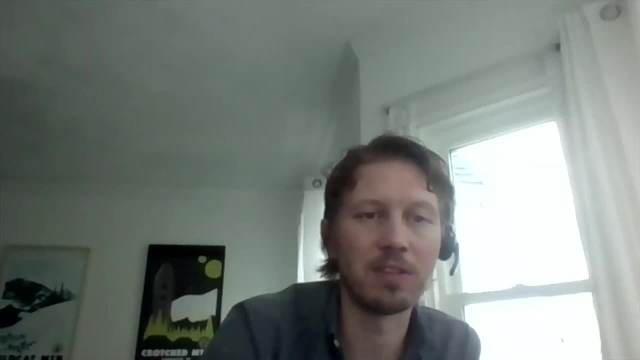 like Doreen and the group mentioned the first of all, the amazing ability to just make shapes the way you want, right, and then to make those shapes do different things and you know the performance, you know carrying. 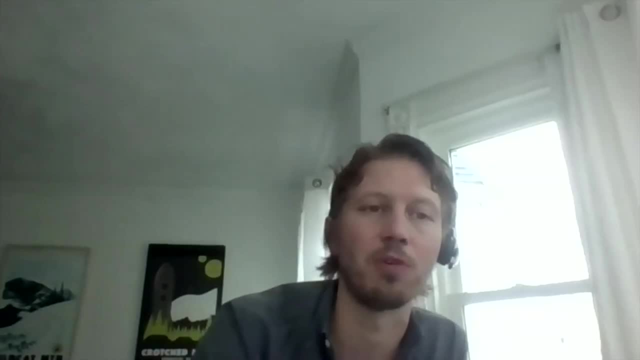 carrying plants holding water being semi-translucent for for that sort of thing, And I really, you know, I've really enjoyed that aspect of it, even if it's fully. that piece, if you will, is fully in the architectural realm, you know. 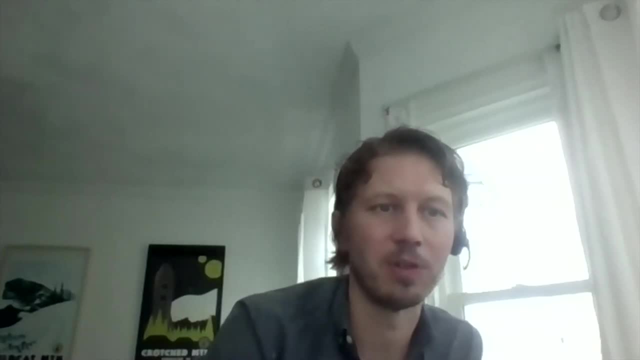 there's little engineering with it and we advise some kind of you know, assembly and attachment. but we do get to kind of nerd out on things like the pull-out strength of a Kyle anchor as opposed to a traditional rain screen clip. So sorry I digress a little bit, but I do think that the big sort of unexplored area still is really the to push the limits of kind of the physical, the mechanical properties of the material and the physical performance of it. 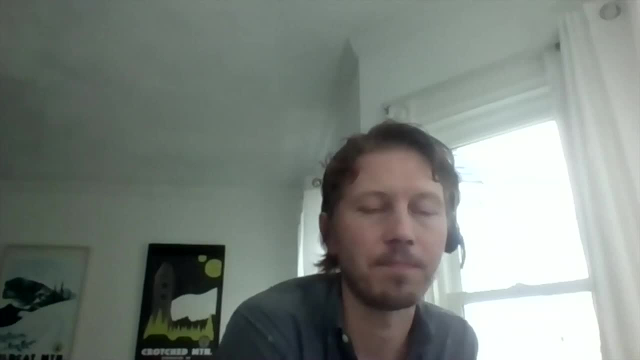 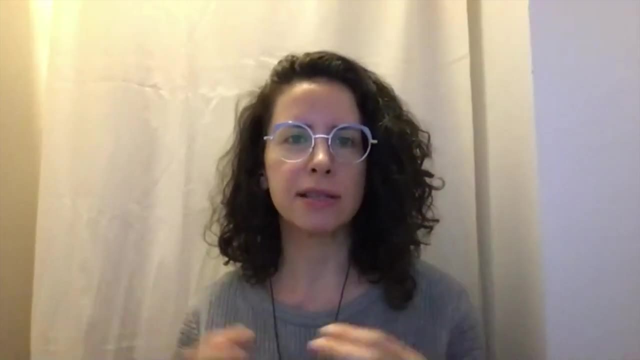 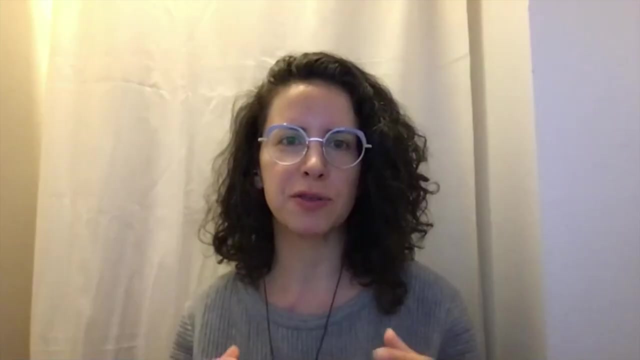 And I think that's largely unexplored yet In Canara- and somebody actually brought this up in the chat- that you have sort of more during a system. I think when we were initially developing our design, we sort of wanted to push it to be. 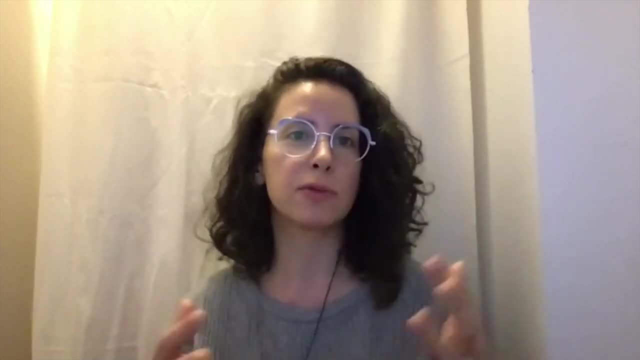 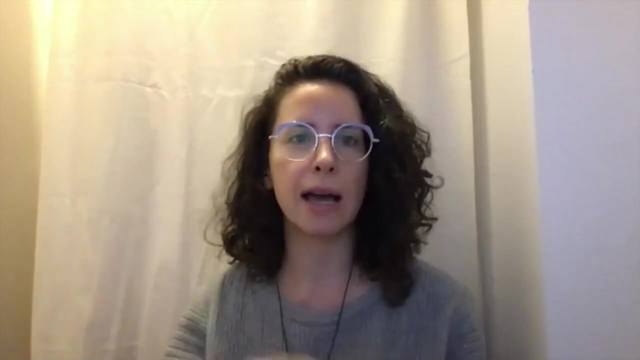 to not have any other elements besides, maybe a mortar, even a dry stack, and then thought: well, maybe we could mortar it. I mean, it was really designed as a brick, something that could stand on its own and stack, and we'll work with Walter P Moore to actually 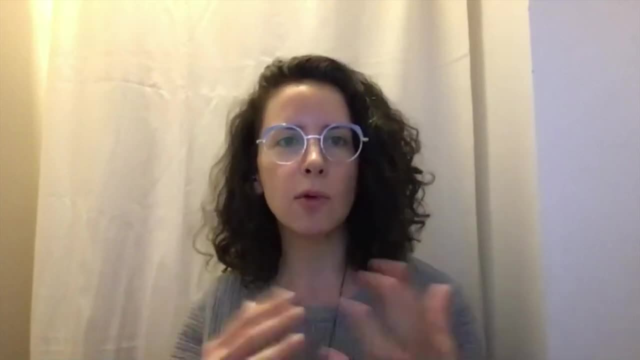 develop it in that way And then, realizing that the mortar was not really feasible for the workshop as we had intended it, we shifted to the custom gasket and hardware system, which actually opened up the possibilities of how we develop that negative space. 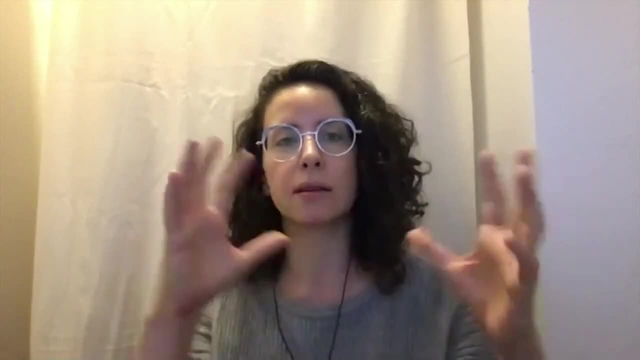 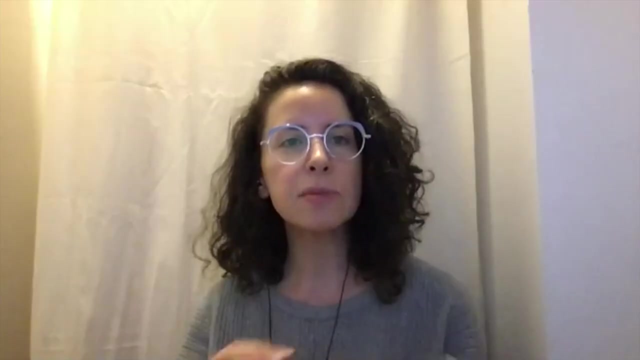 which became a really important part of the project And as much as we designed the module itself, that in between space started to become just as much of a design element. So the added material, as much as we initially were kind of resisting it. 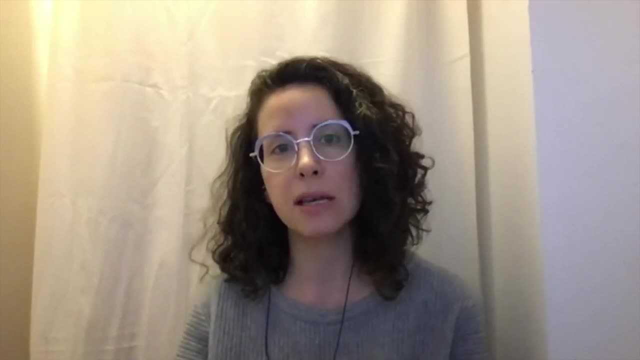 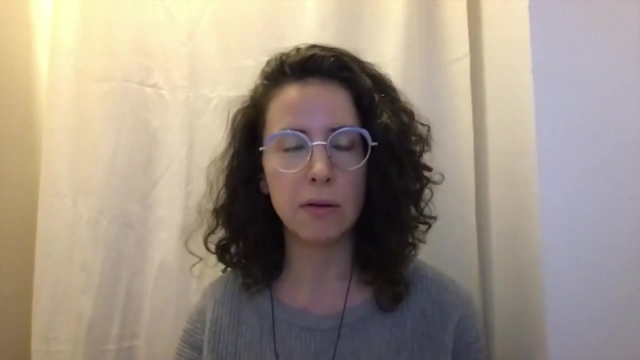 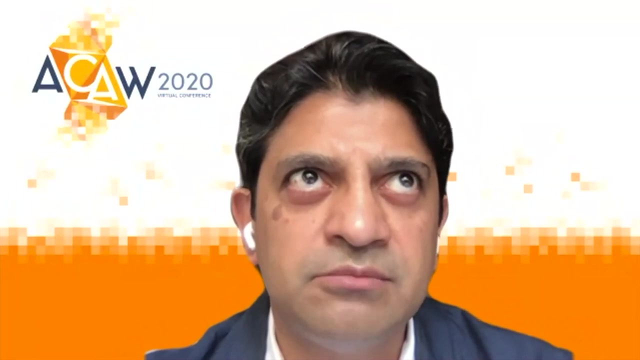 really ended up adding an important piece to the process. So I think it opens up possibilities that might not be available if we sort of take a more purist approach to it in a way. I mean one question I had as you were showing that silicon gasket- I mean silicon probably. 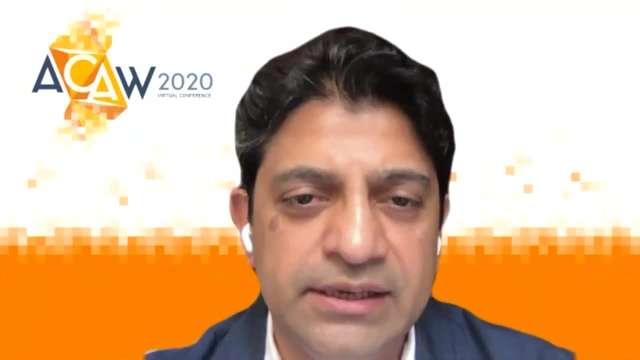 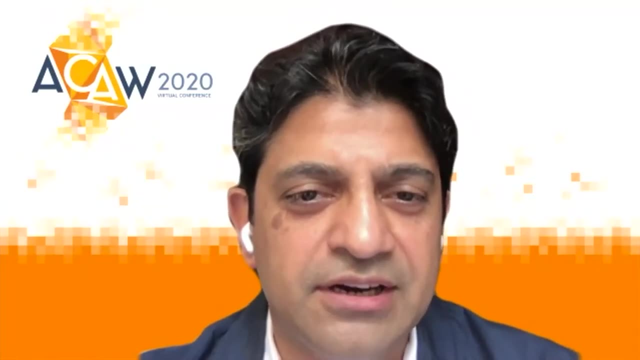 in terms of its ability to sort of handle that kind of weight and so forth, may have less than 20 years on it and you have a material that's a good 100-year material there on top of it. I'm wondering if actually its own deterioration. 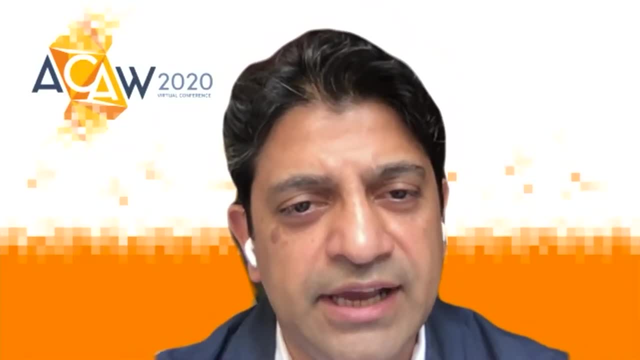 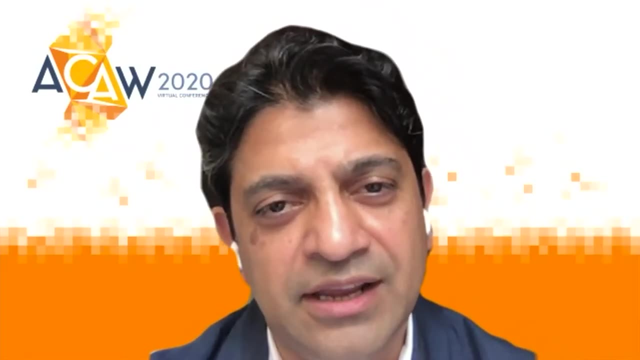 did you feel that that would be okay in terms of whether that gasket performs precisely or not? I think those connections are getting to become more and more interesting, especially when we're looking at these modern systems and this whole question of maybe the older systems. 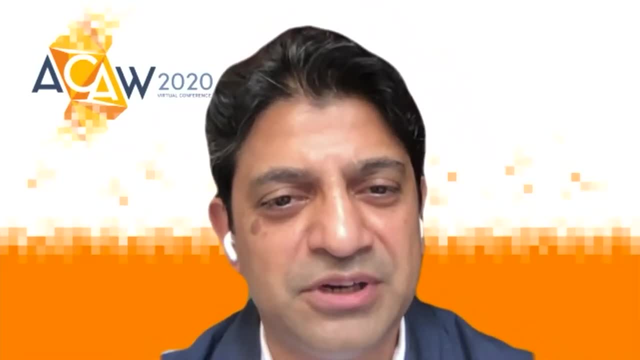 of putting things together, whether it's mortar or stuff, or really had maybe better sensibility for longevity and durability. But maybe your geometry seemed to be able to stand itself because it was like a dry stack right That even if there was a collapse. 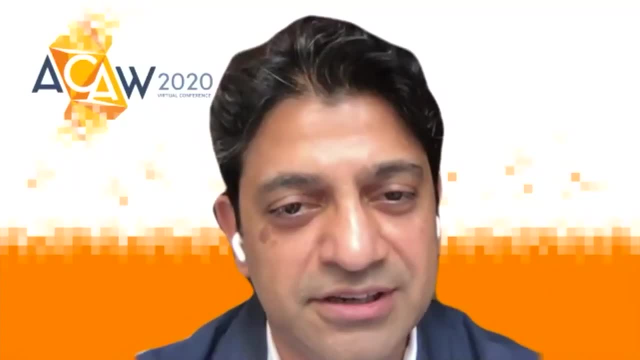 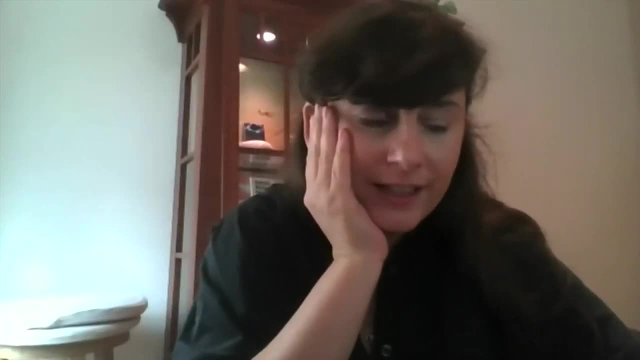 it wasn't gonna collapse, It would just sort of get tighter or something. That's a really interesting comment, because certainly, like Guastavino, his tile work is structural, And so I think in the conversation about structure and terracotta I'm kind of with Gustav in that there are limits to terracotta. 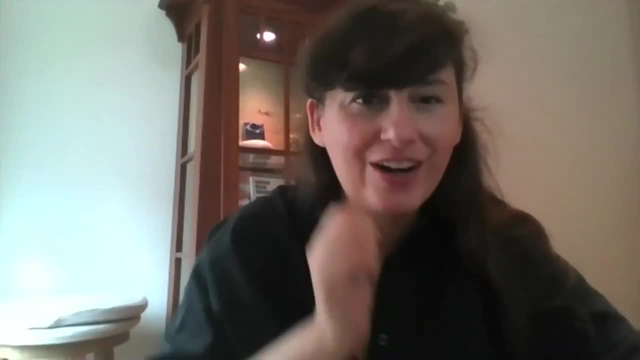 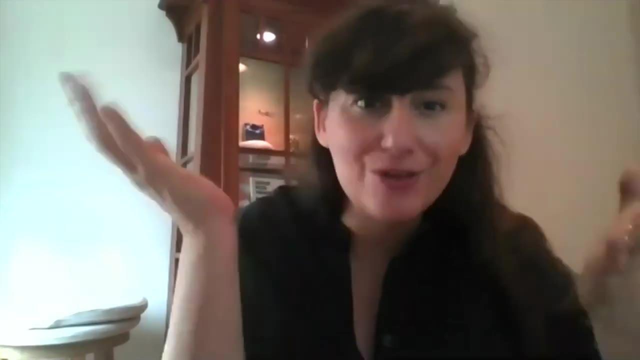 and playing to those limits might not be a bad thing. However, if there was an argument to be made for limiting the amount of aluminum connections in order to not use as much aluminum, because we all know that's, you know, dangerous looking forward. 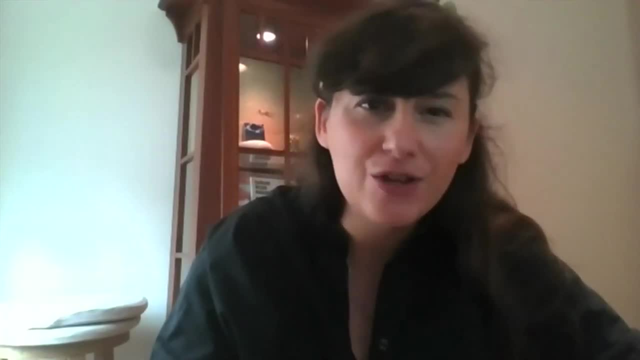 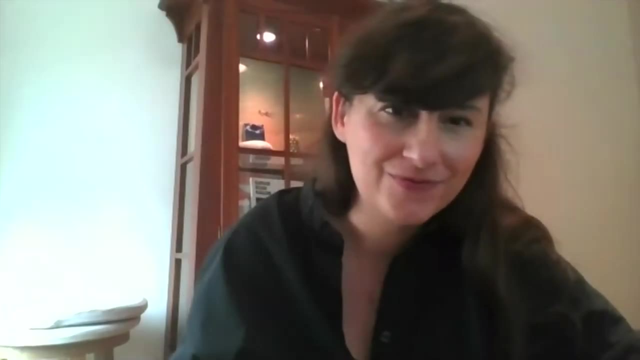 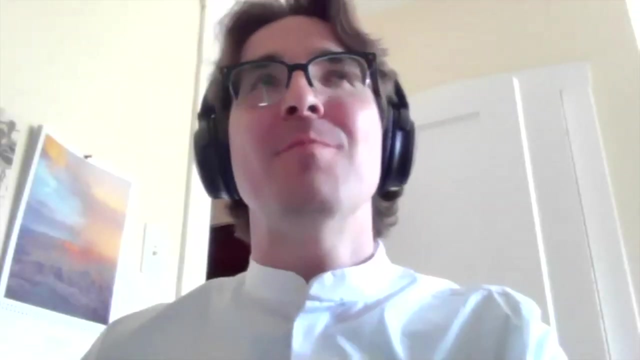 I would be interested in that, Like, how can you minimize the number of connections? I'm not sure We haven't studied that, but I would love to. Well, I think. sorry, Dorena, I love that One of the pieces of research. 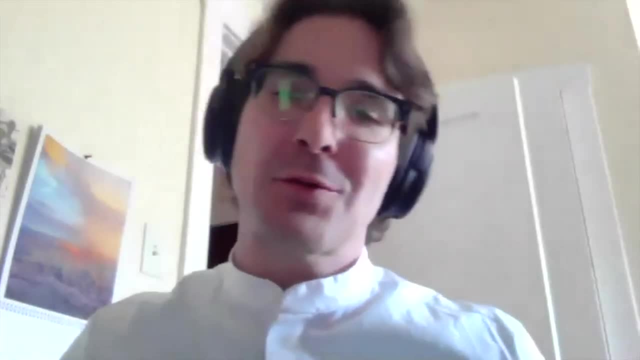 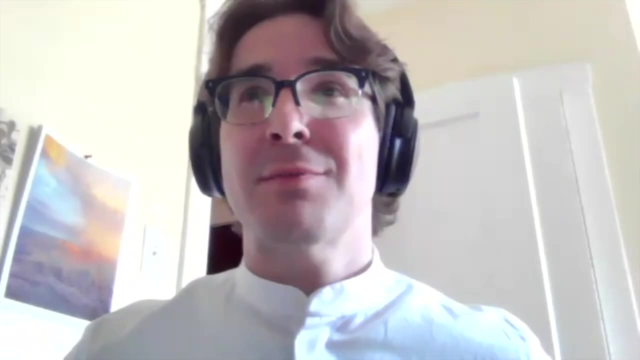 before we kind of initiated our kind of material research. so the historical side of it, that was never quite answered. but I'd be really curious to know if anybody- this might tie into that a little bit- and I'd be curious to know if there's anybody out there- 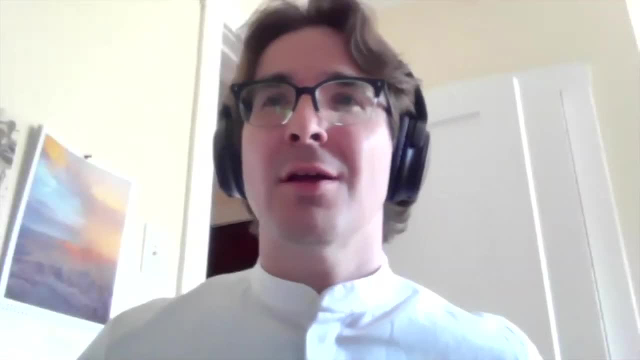 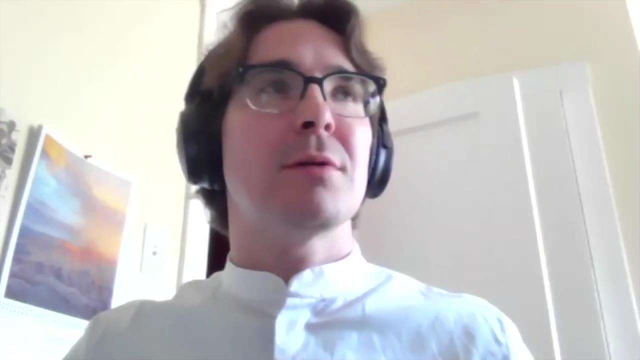 that knows more about this, but we were trying to find more information on the reasons why some of these structural applications became less favored. We did find some that were a little bit more obvious, but some that we really couldn't explain. We touched on that lightly regarding the tolerances. 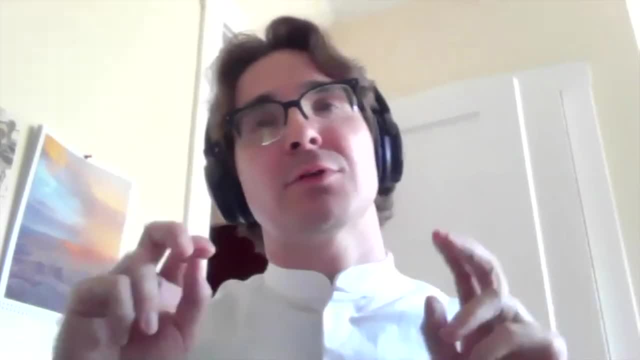 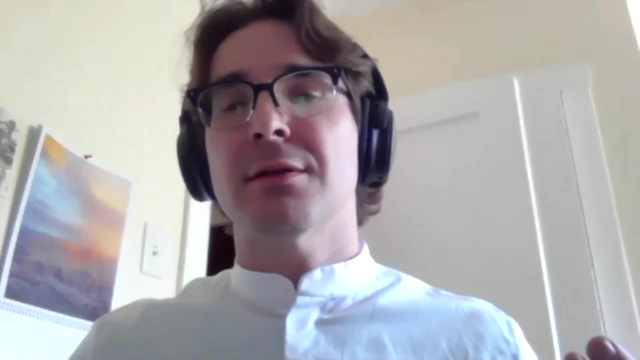 of some of the surrounding infrastructure, if you will, to accept the terracotta pieces. But one clue to that might be to why historically they did. but one clue to that might be to why historically they did. but one clue to that might be to why historically they did. 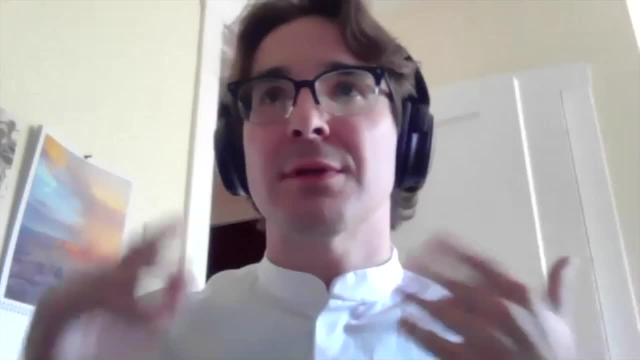 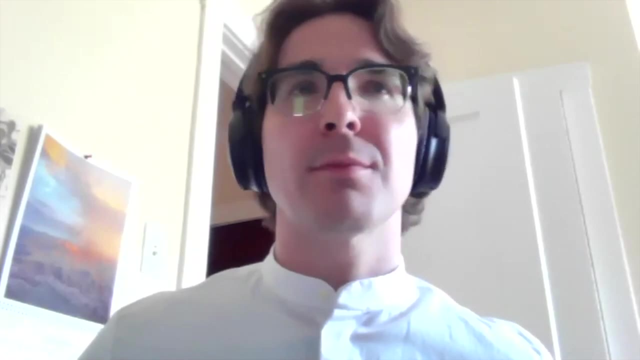 they seem to have dropped out of favor to the facade And of course we again like we know that they make a lot of sense in both applications, but why do we only see them on the facade now? by and large, I think to some of the points and Omar. 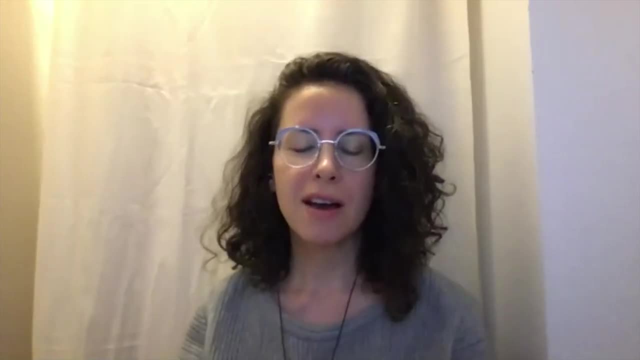 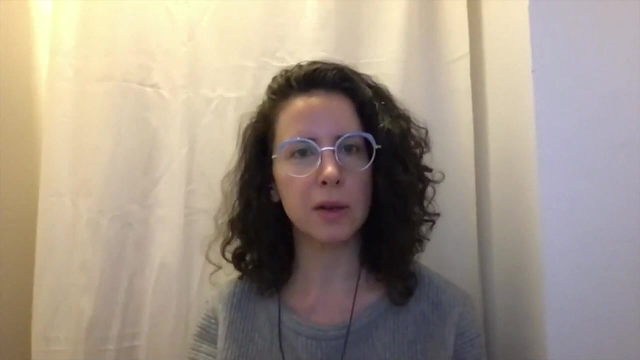 your point in particular about the durability of the material. one intent in trying to think through how could the system actually be more of a standalone system without needing some of these extra pieces? without needing some of these extra pieces- was that we did imagine it as something. 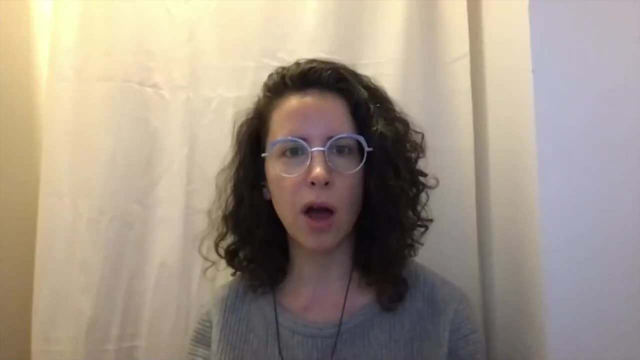 that could stand out in nature. I mean looking at the some of the rock walls, the moss-covered rock walls, that inspired some of our thinking. There was, I think, maybe a notion that in an idealized setting, if we could figure out how to do this, 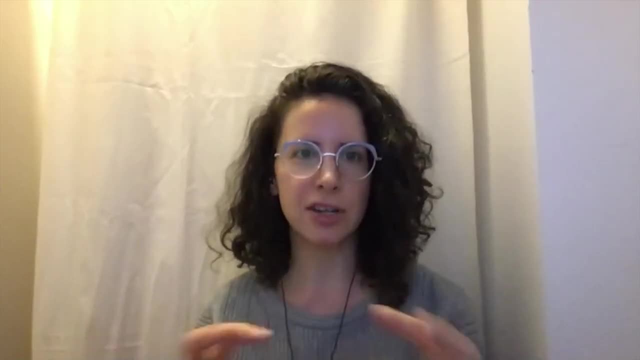 you could actually build this as one of those walls and let nature kind of take over and start to fill in those cavities and provide the glue that would hold it together. So I mean, that's kind of looking at a much longer process. but 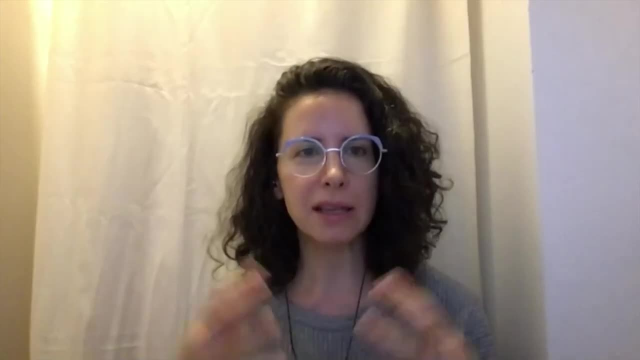 So I mean, that's kind of looking at a much longer process but longer time span of it, But I think that was something that was. the ideal version of it would have been that in a way, Yeah, no, that actually speaks to duration and longevity. 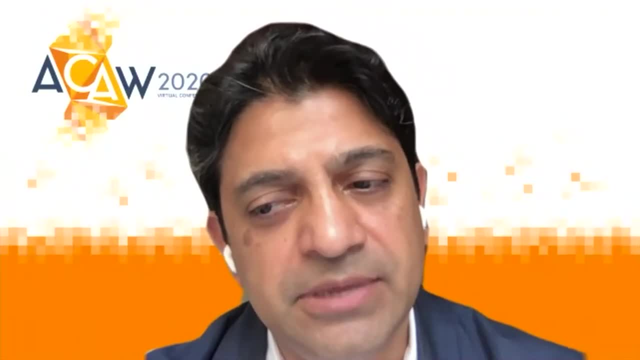 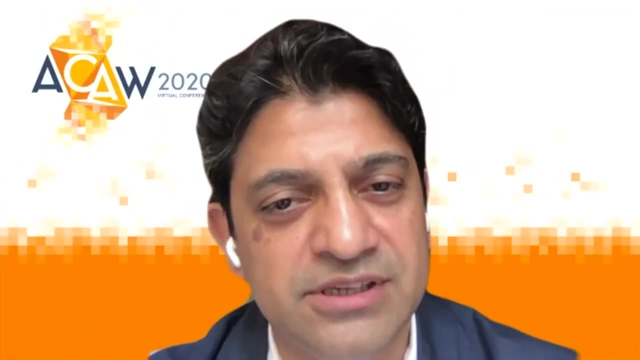 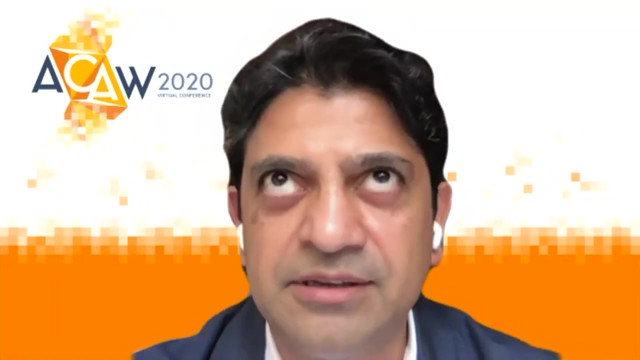 in an interesting and nice way would evolve. Just speaking a bit to Maciej's question, initially it was really the fireproofing qualities of terracotta that was the attraction. So for the large, the tall skyscrapers were to protect the metal and that's why it was structural. 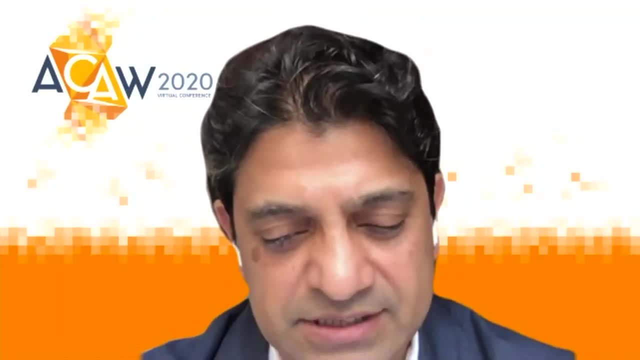 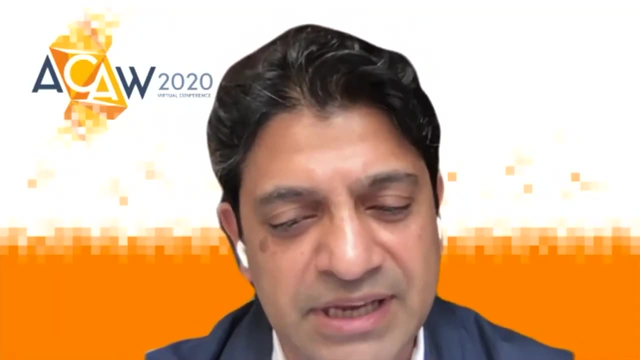 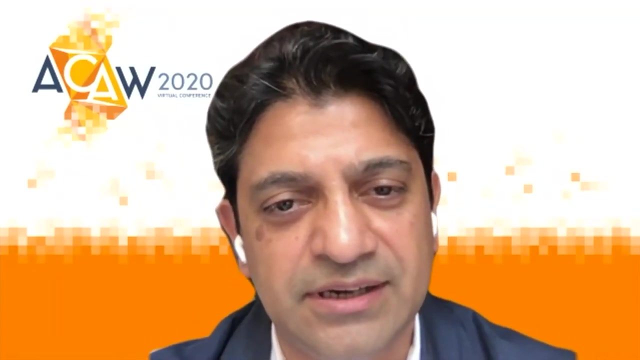 And we see that still a lot in the buildings of the 50s and so it's kind of fireproofing partitions and stuff. But yes, I guess, as we began to become more modern, yeah, it just lost its fancy, just was too ornamental and so on. 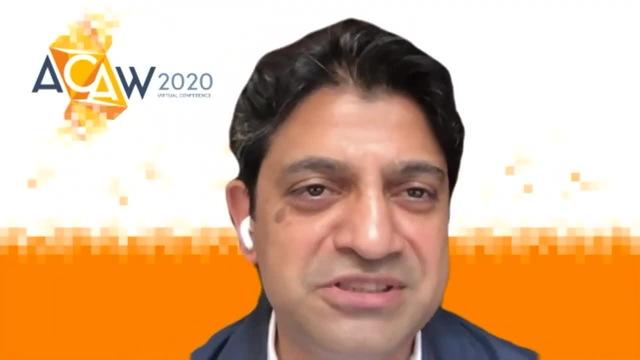 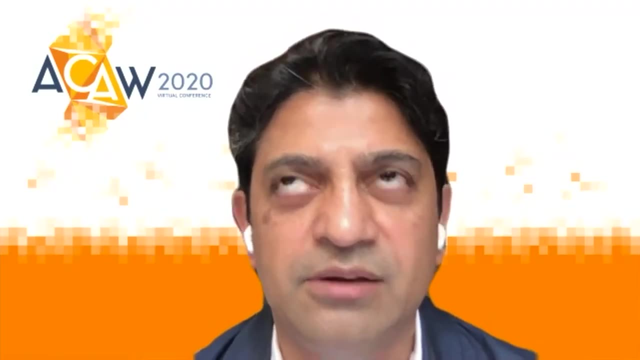 But I think it was PLP who sort of brought up, of course, the self-preservation of the facades. It's a question of now the facade as a potential fire. We saw this terrible thing happen, Of course, in London with the fire going up on the facade. 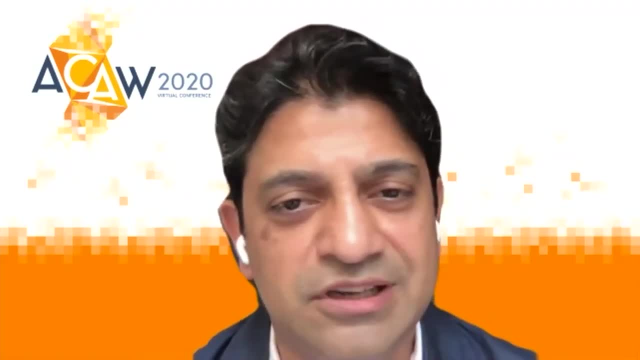 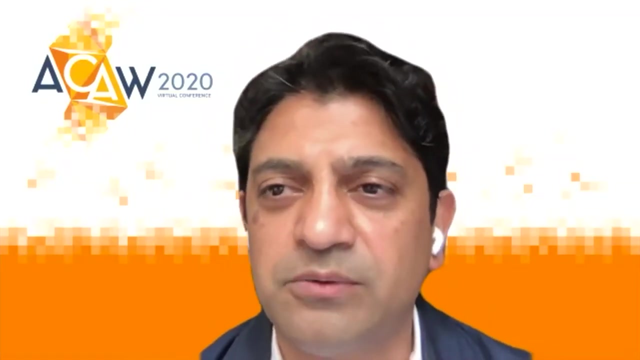 This is one of the another really interesting quality that we haven't really explored in Eolital, about fire and fireproofing as a kind of phenomena that terracotta's actually a really great material to sort of work with. Are there any questions you guys have? 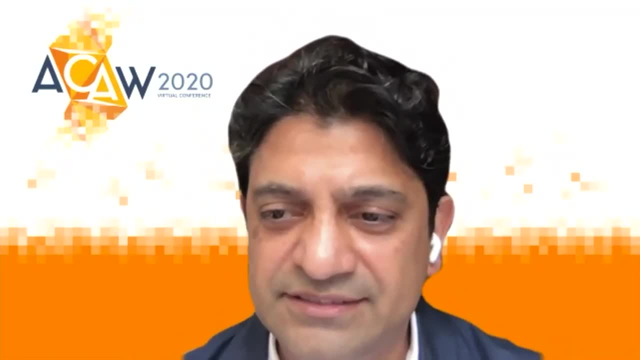 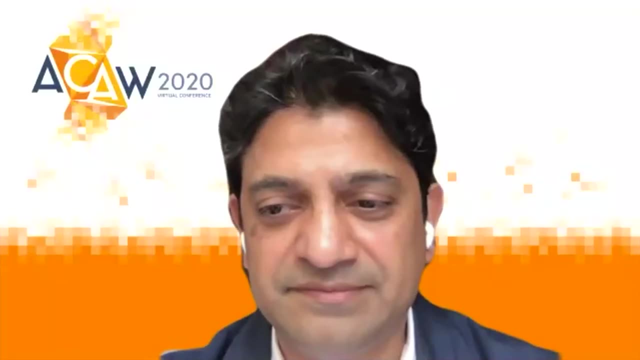 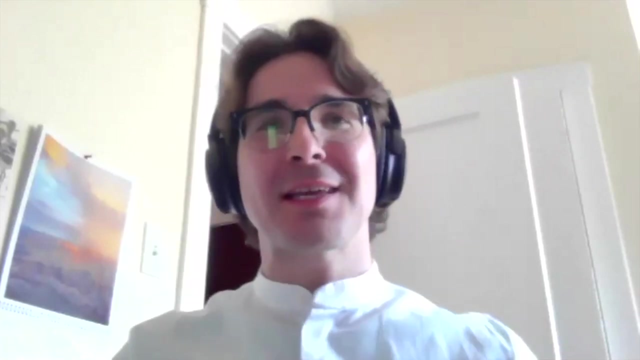 each other. I'll just say this isn't a question so much as, like a kudos I was. I was very much impressed with the, the alignment of your tool paths for the, the different mold pieces, of the molds that came together. so I want to acknowledge that I know how difficult that such things can be, so hats off. I. 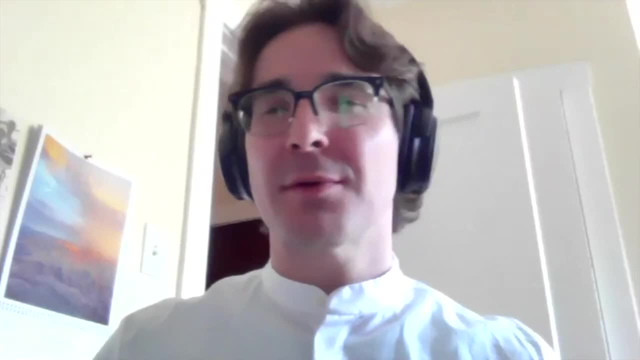 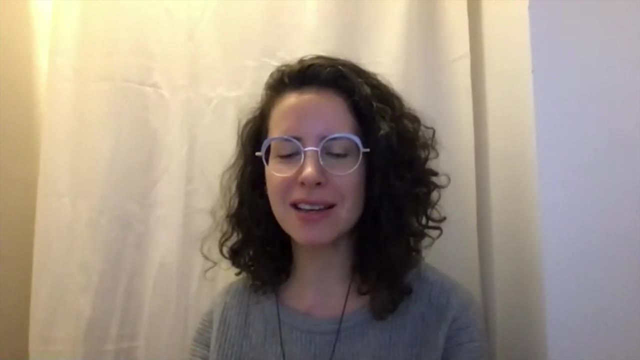 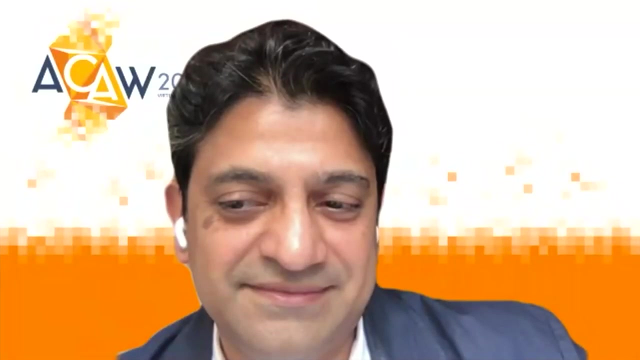 believe that was from men. I think you spoke about that portion of it. yes, thank you it it. I think somebody much- I think Andy- mentioned how things that look pretty simple or straightforward- yes, that there's actually so much more that goes behind them. this is one of those cases where we spent way longer than you. 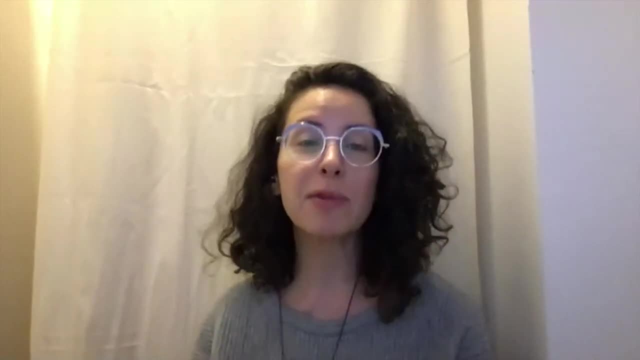 would imagine developing those alignments and- and we didn't actually basically had one shot to do, couldn't really test it because we had limited access to the element facilities given all the covered restrictions, so we sort of had to get it all done, kind of imagine like, okay, this is. 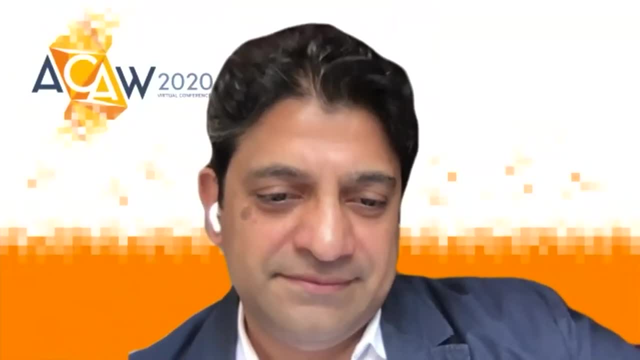 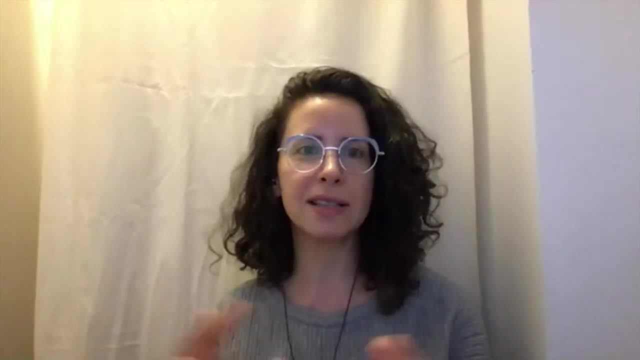 gonna work. you think it's gonna work, go in there and just like hope so and thank you. I mean, Andy has a tremendous amount of work to then make all that happen because at the end of the day, he gets these separate pieces and he has to fit.